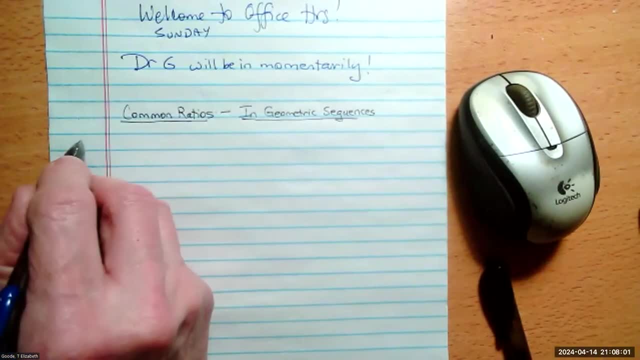 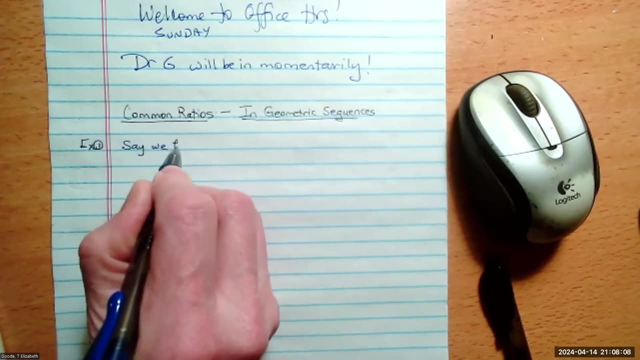 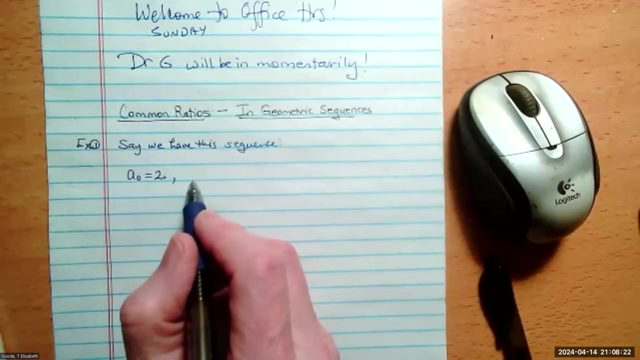 So shall we look at an example? Let's look at an example. Let's say we have this sequence. Let's say the initial term is two, So a naught is two. Okay, And let's say that the common ratio turns out to be three. 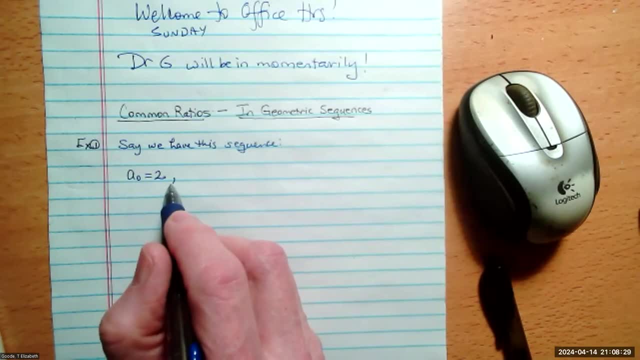 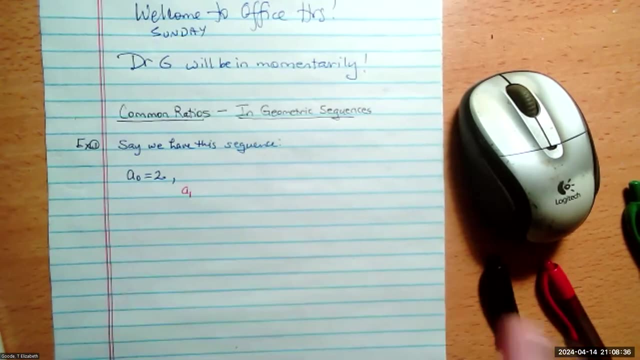 In other words, we're going to multiply by three, over and over again. Okay, So the term a1 is the term that we get when we multiply a sub zero times three. What would a1 be? We multiply two times the common ratio three, we'll get six. 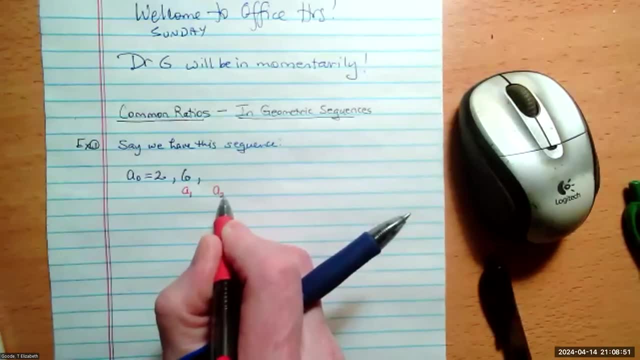 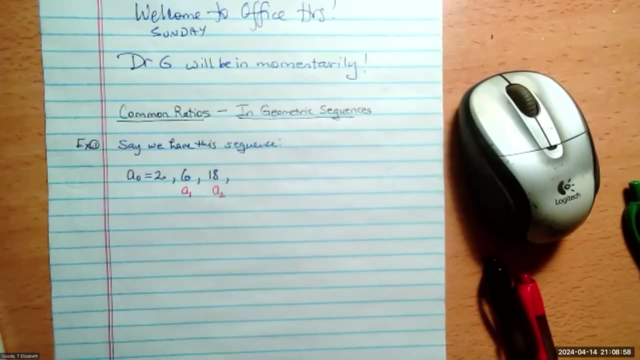 Okay, And now we just keep multiplying by three. So we take six and we multiply it by three, We get 18.. What would the next term be? Three times 18 is 30, plus three times eight is 24, that'd be 54.. 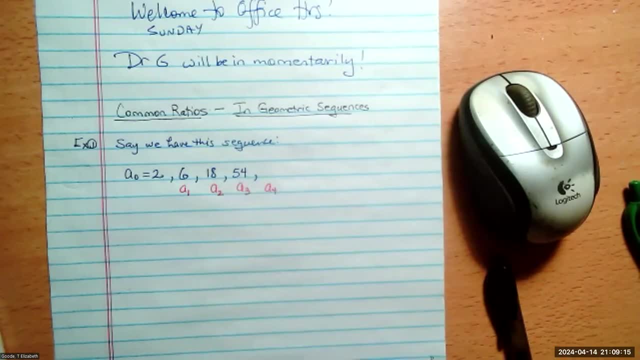 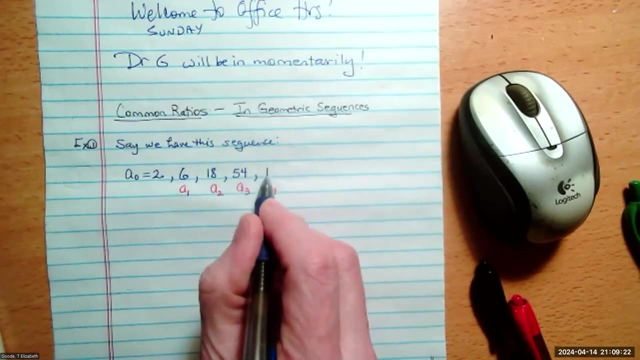 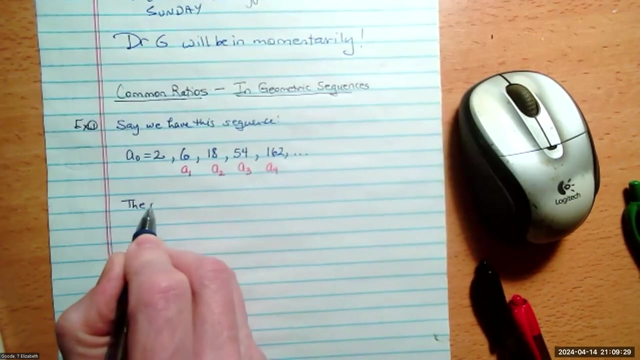 And then we multiply that term by three to get the next term. So three times 50 is 150.. Okay, Three times four is 12.. So 162.. That's enough to see what's going on. Okay, The common ratio is a sub k plus one divided by a sub k. 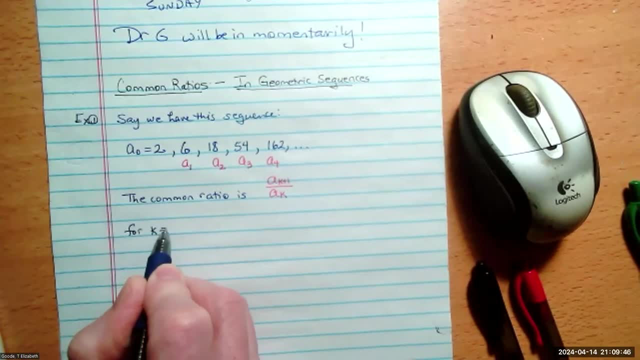 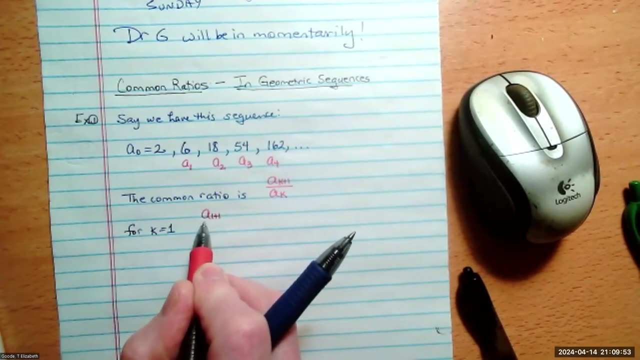 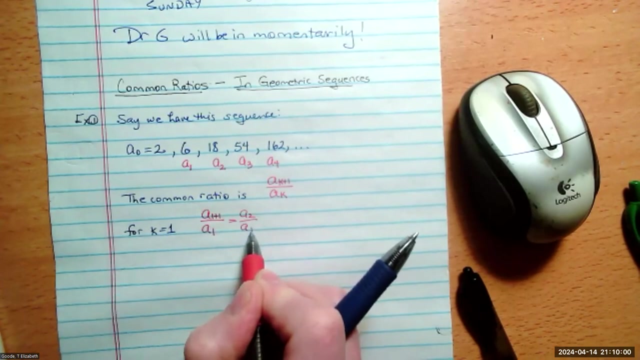 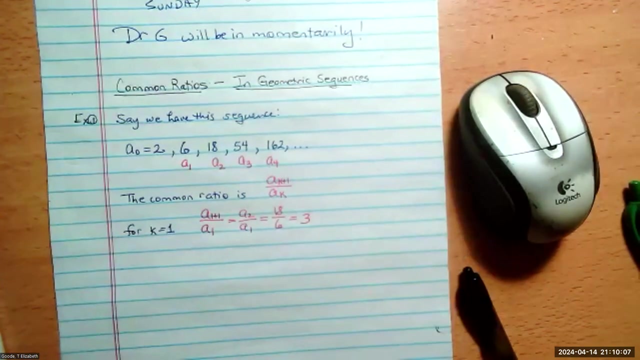 So for k equals one. Okay, The common ratio is a sub one plus one divided by a sub one is a sub two divided by a sub one. Well, a sub two is 18, a sub one is six, and we get three. 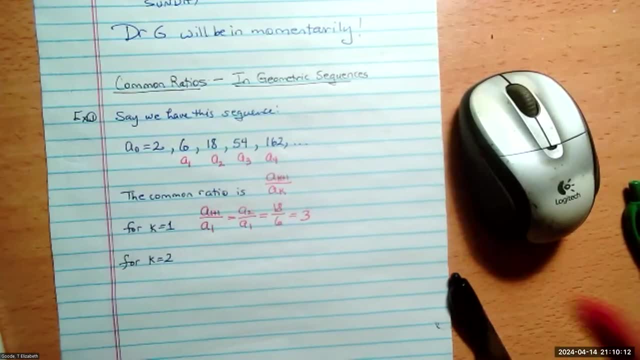 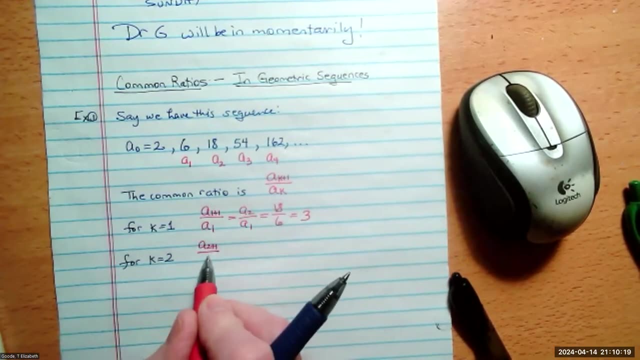 Let's look at: k equals two, We should get three again. A sub k plus one is a sub two plus one divided by a sub k. Well, k is two, So divided by a sub two. So we're looking at the ratio of a sub three divided by a sub two. 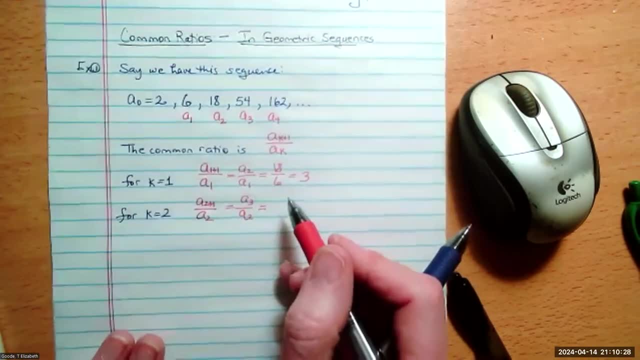 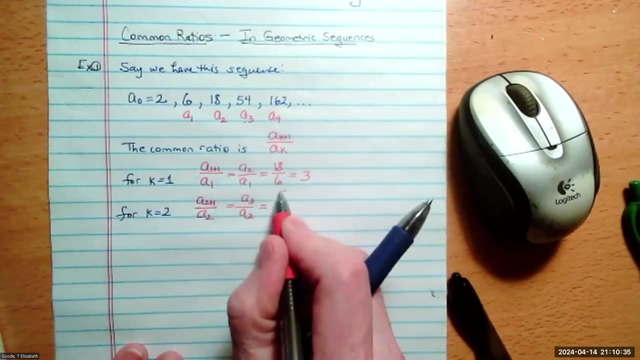 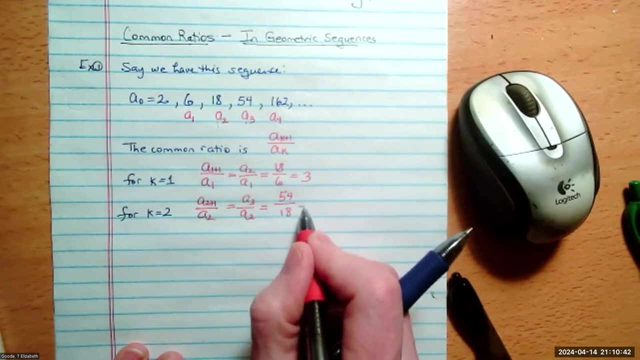 What is a sub three? 54.. Yeah. And what is a sub two: 18.. Uh-huh, And when we divide 54 by 18, we get three again. You see, So for every k it'll even work, for k equals zero. 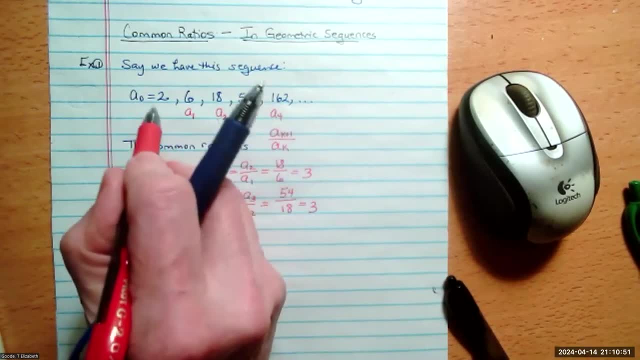 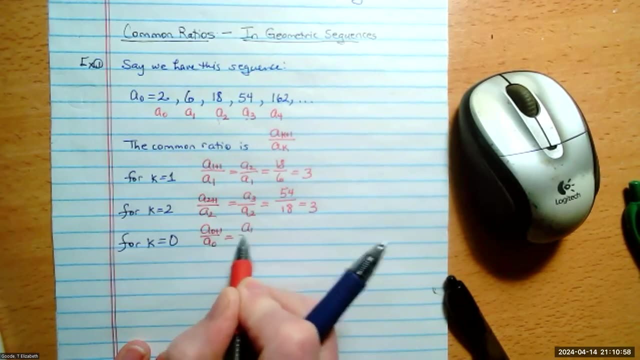 Okay, When k is zero, see, this is a sub zero. a sub zero plus one divided by a sub zero is a sub one divided by a sub zero. That's kind of the first one, actually, that we could do if we wanted. 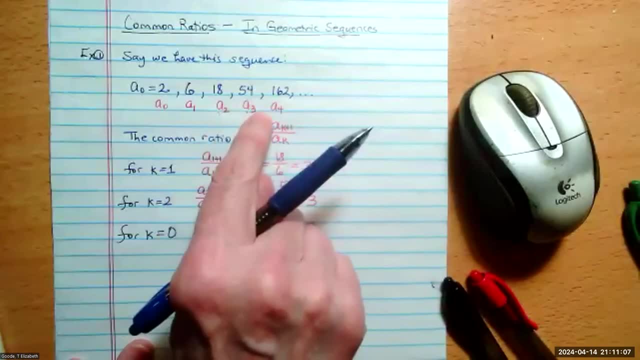 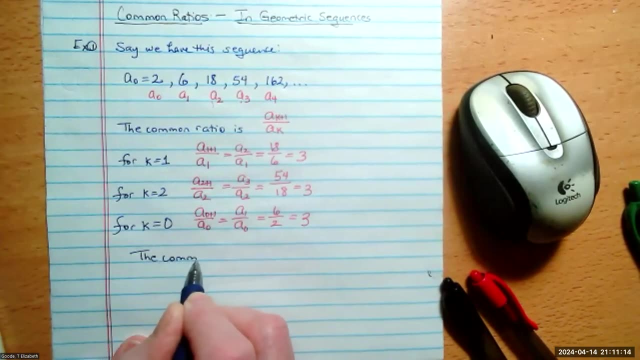 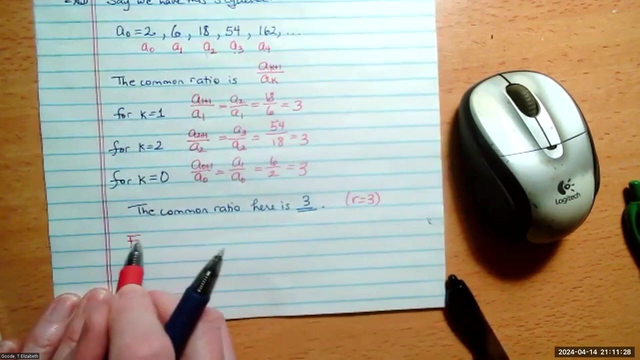 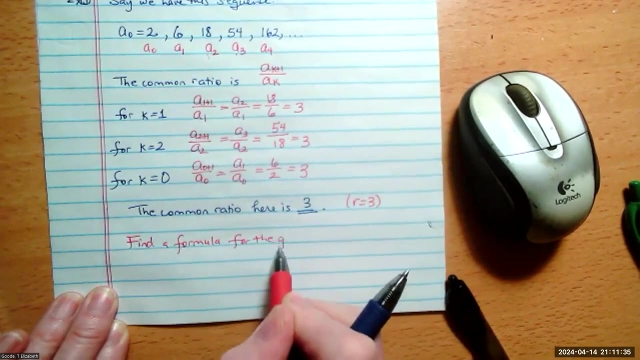 We get three over and over again. So we'll multiply it by three to get subsequent terms. Does that make sense? Yes, So the common ratio is three. So we call that r. r equals three. And now let's find a formula for the general term, a sub n. 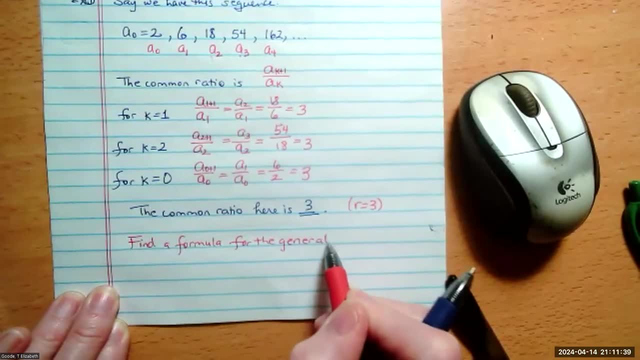 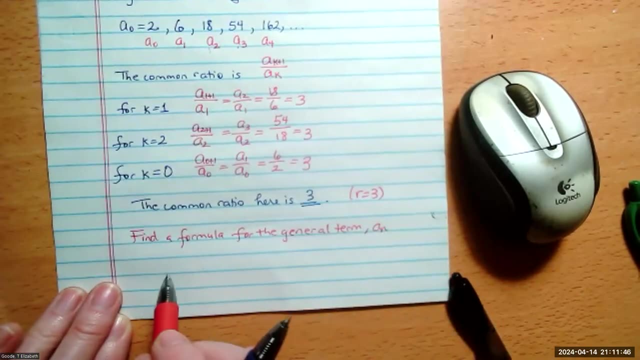 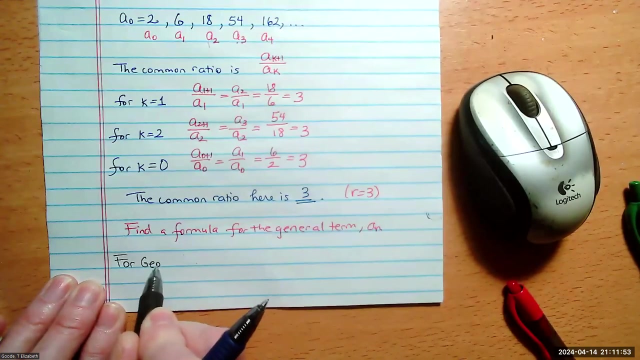 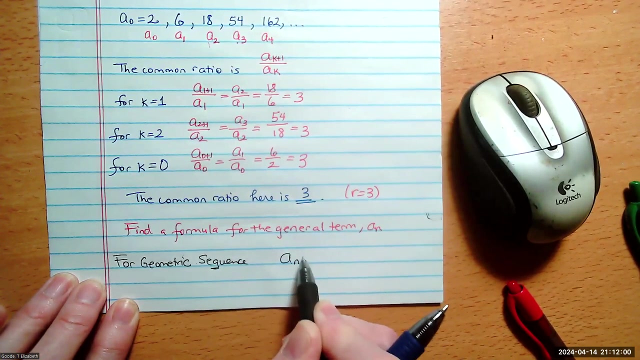 All right. So if you go back and look at the notes In general for a geometric sequence, there's a formula for how to get the term a sub n. A sub n is the initial term. it's always a sub zero times r raised to the nth power. 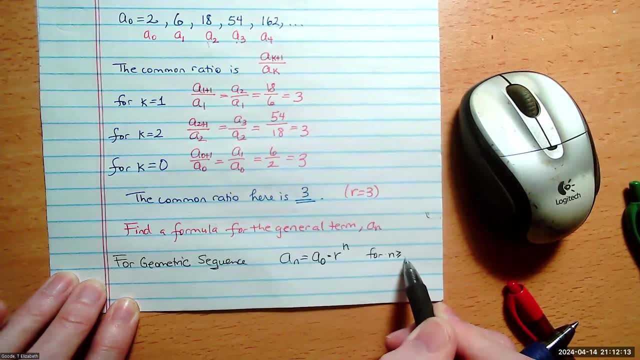 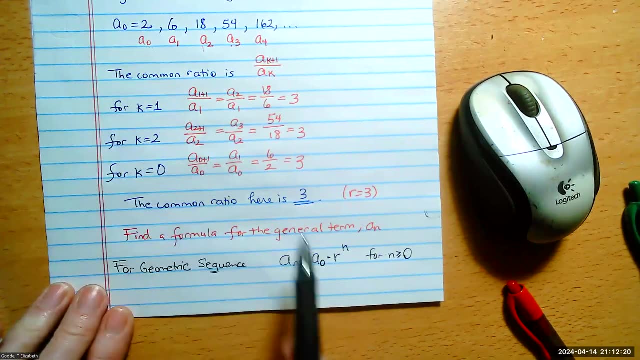 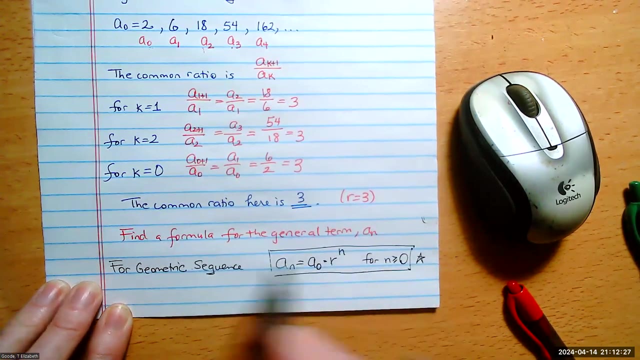 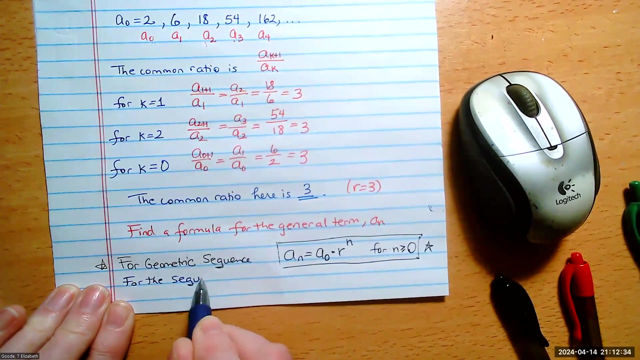 And this is for n greater than or equal to zero. Okay, Okay, Okay. So this is going to start with the first indexing number being zero. This always works. So that's just in general For this sequence. in Example One. here, the initial term is two. 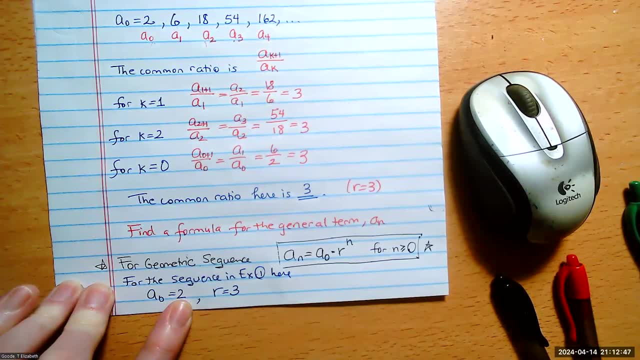 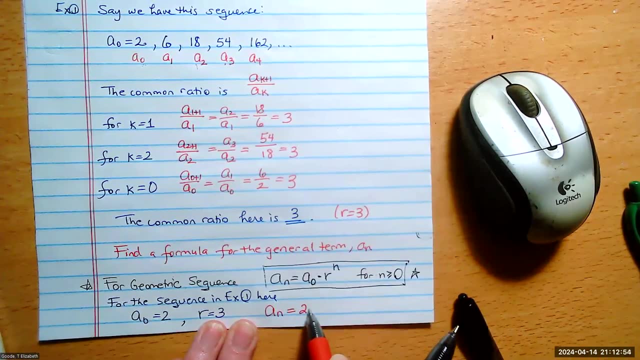 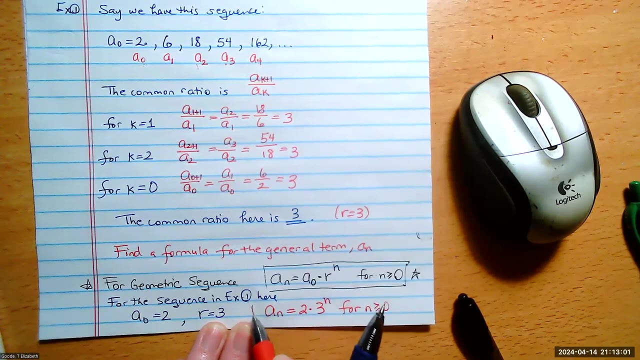 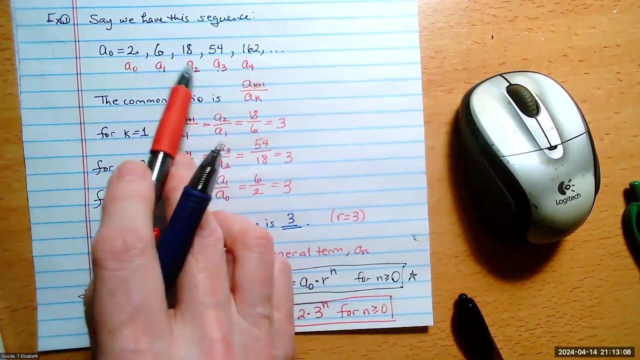 The common ratio is three. So the formula for a sub n is 2 times 3 to the n for n greater than or equal to 0. And you can check that and it will always work. It'll give you each of these terms like a sub 3. 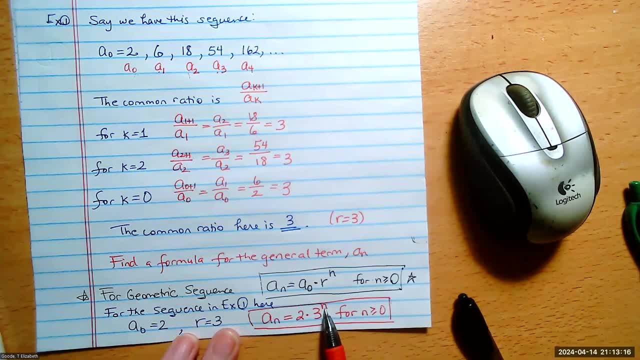 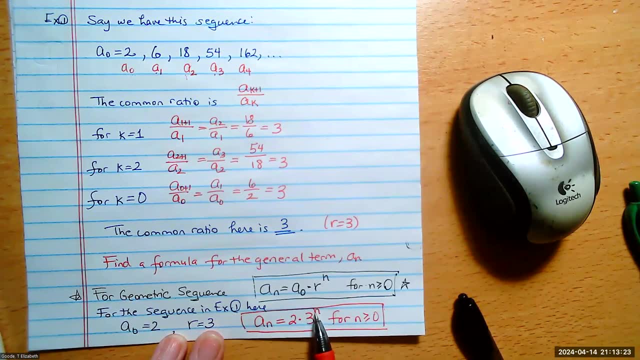 should be 2 times 3, raised to the 3.. In other words, 2 times 9.. Excuse me, 2 times 27,. my bad, Yeah, that's 54. Let's check it for a sub 2.. 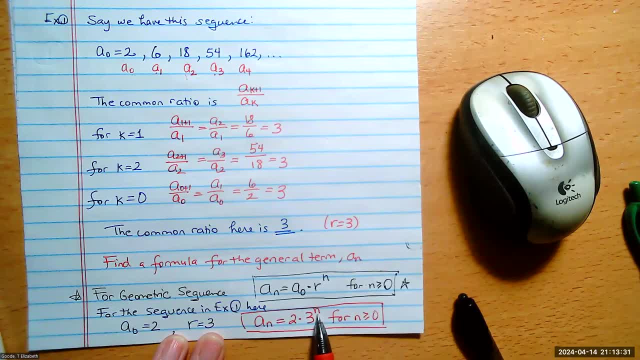 a sub 2 should equal 2 times 3 squared. Oh, that's 2 times 9.. Yeah, a sub 2 is 2 times 9, because it's 18.. Let's check it for 1.. a sub 1 equals 2 times 3.. 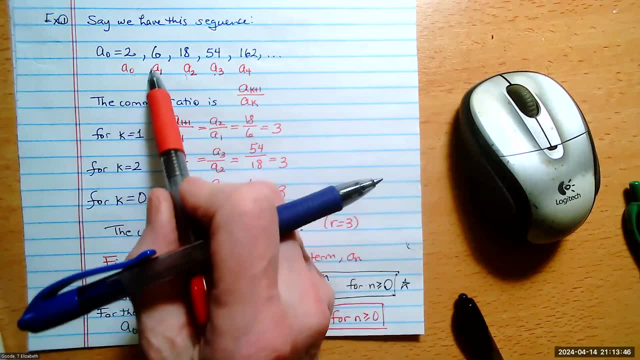 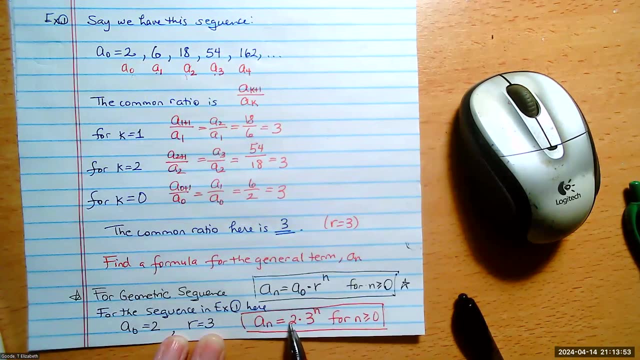 That's 3 to the 1.. That's just 2 times 3,, which is 6.. Yeah, a sub 1 is 6.. We could even back up and check it for 0.. a sub 0 is 2 times 3 to the 0.. 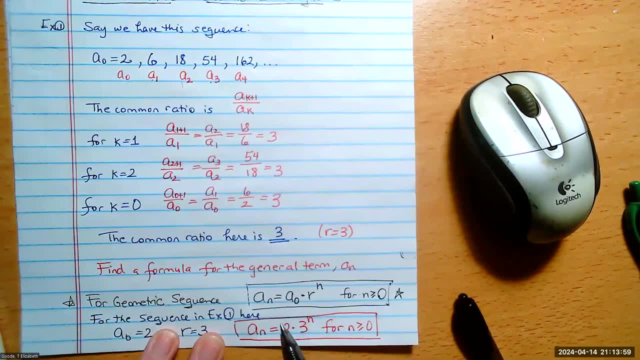 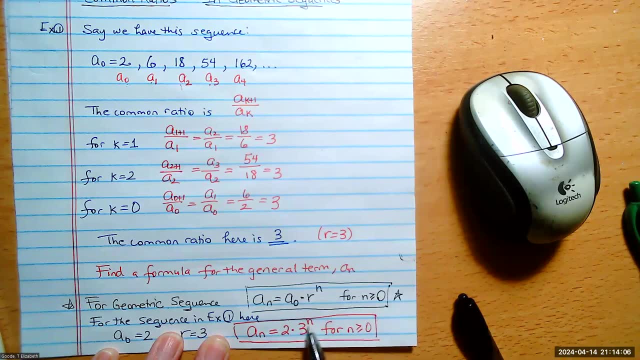 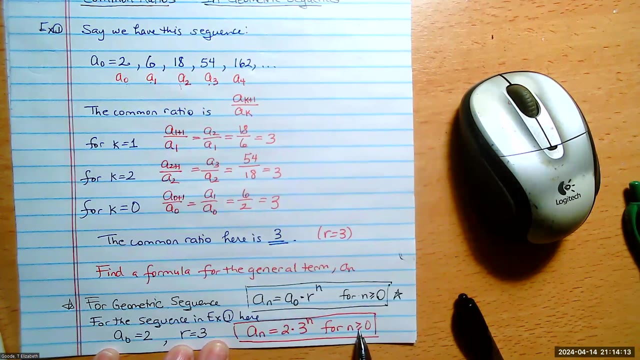 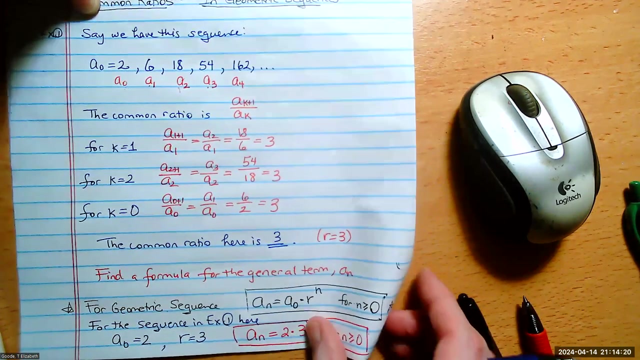 What is 3 to the 0? 1.. And isn't a sub 0 equal to 2 times 3 to the 0,, or 2 times 1?? Sure, See how that works. Yeah, thank you. Want me to give you another one to work on now. 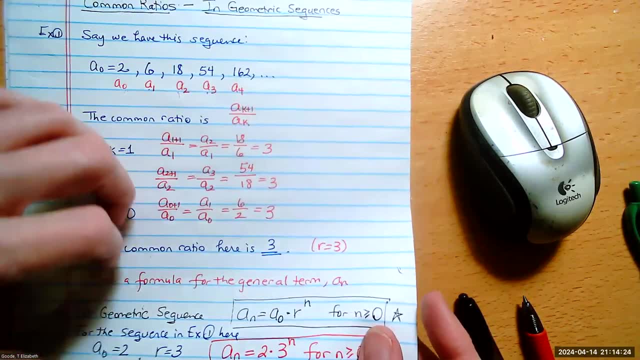 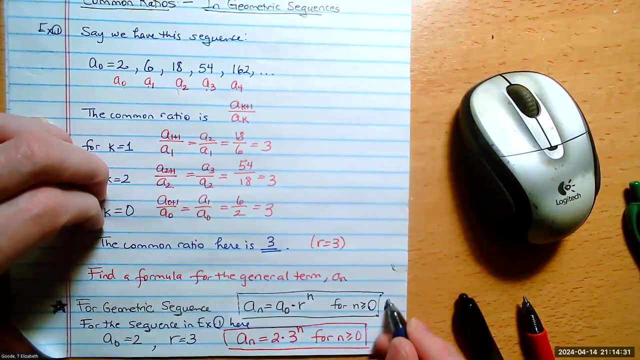 Yes, please. All right, let's do another one And we'll keep this formula in general. This is the general formula that just works for all geometric sequences. We just have to figure out what the initial term is: a sub 0.. 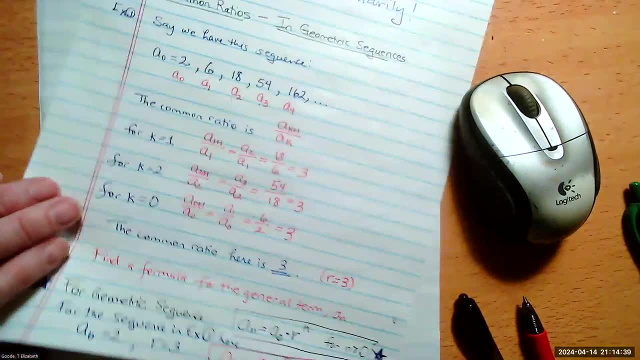 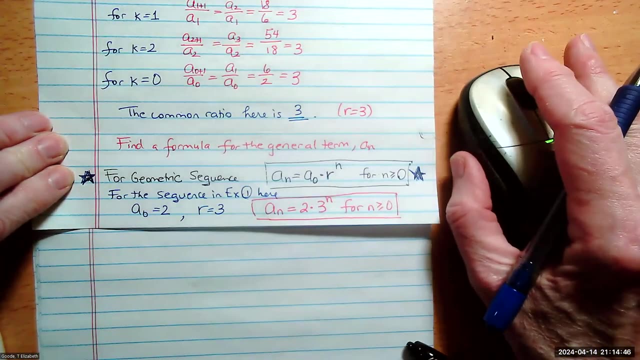 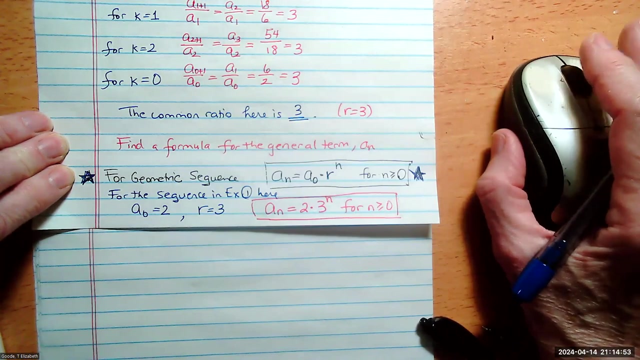 And then we have to figure out what the common ratio is. So how about this one? I'm looking at the notes, because I gave some do-laters. All right, let's do the do-later. This was from day 18.. 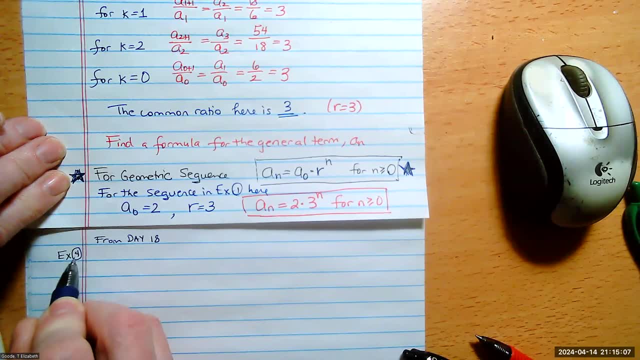 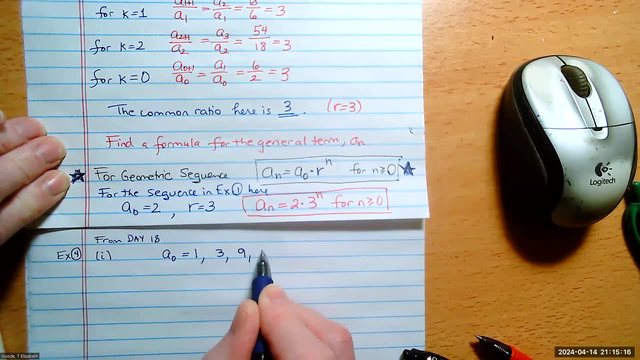 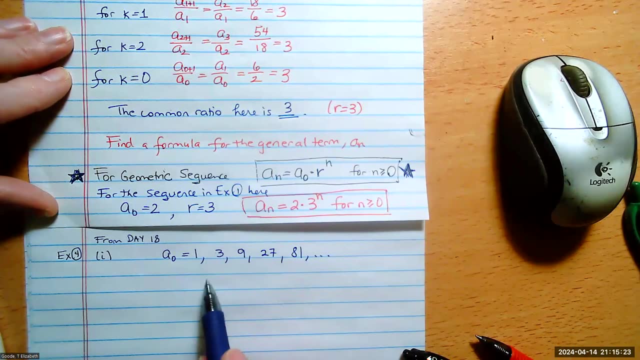 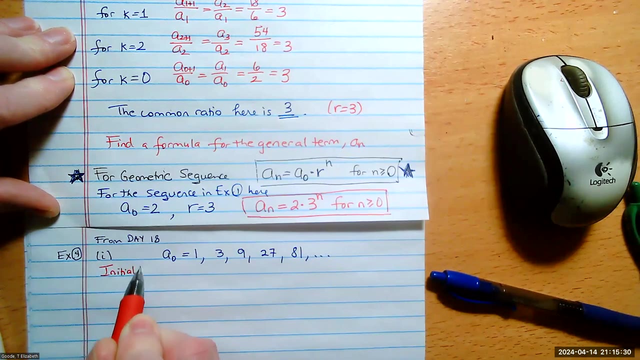 It was: a0 equals 1. 3,, 9,, 27,, 81,. dot, dot, dot. So it's a lot like the one that we just did. What's the initial term? It's a sub 0.. 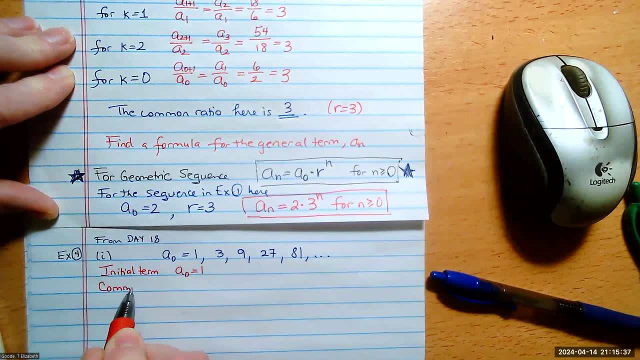 It's 1.. What's the common ratio here? What are we multiplying by, over and over again, 3., 3.. So our general formula says: hey, a sub n is the initial term, which is 1 times the common ratio, 3 raised to the n. 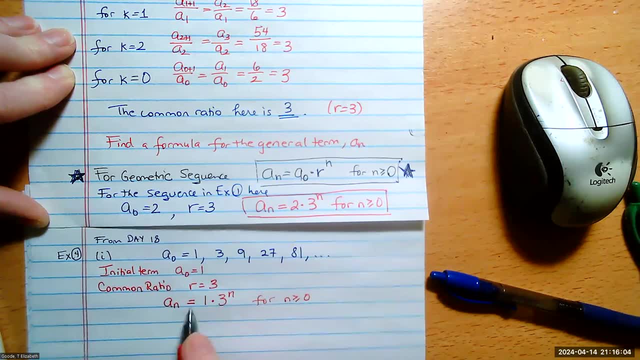 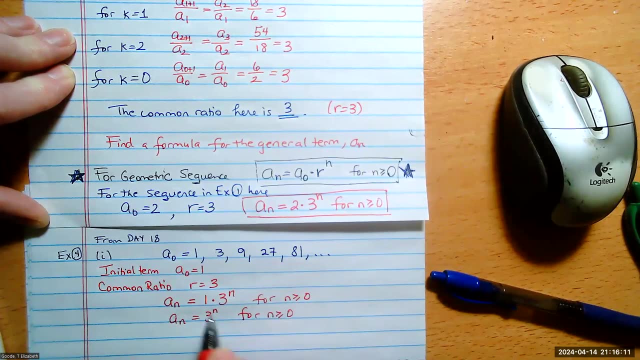 And that's for n greater than or equal to 0.. Or you could just write a sub: n equals 3 to the n for n greater than or equal to 0,, since the initial term was 1.. Instead of like 2 or some other number. 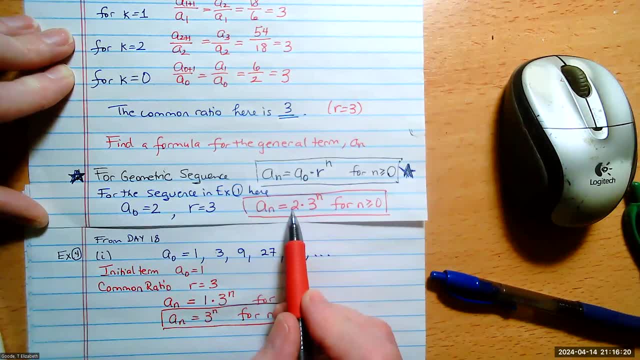 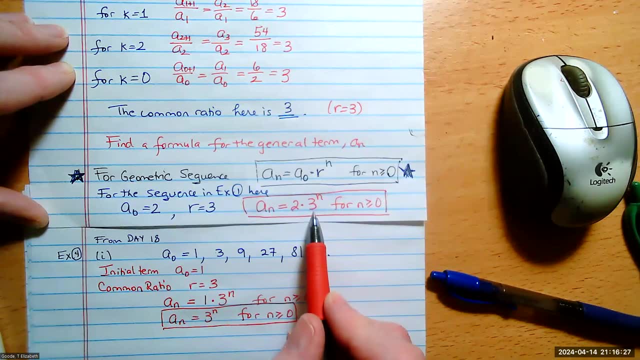 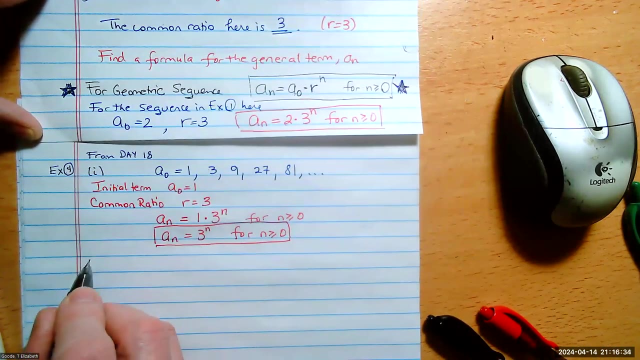 Notice here in this formula, in our example 1 that we just looked at, the 2 isn't getting raised to the n, Only the common ratio 3 is getting raised to the n. All right, let's look at example 4, number 2.. 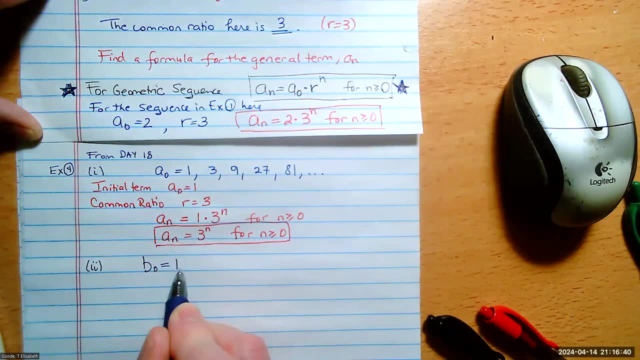 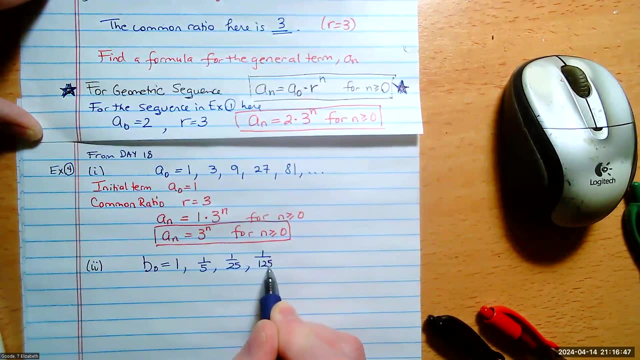 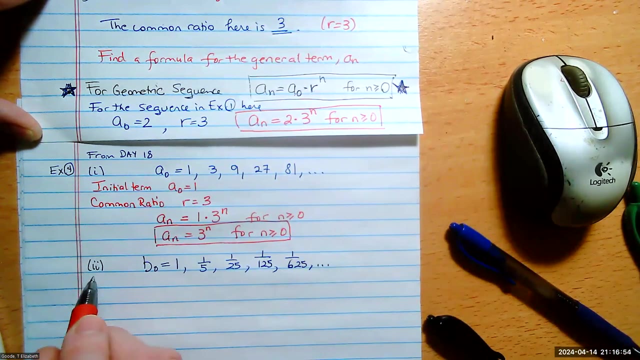 We're told that sequence is: b0 is 1, and then it goes to 1, fifth, 1 over 25,, 1 over 125,, 1 over 625,, dot, dot, dot. So the initial term is: what is the initial term? 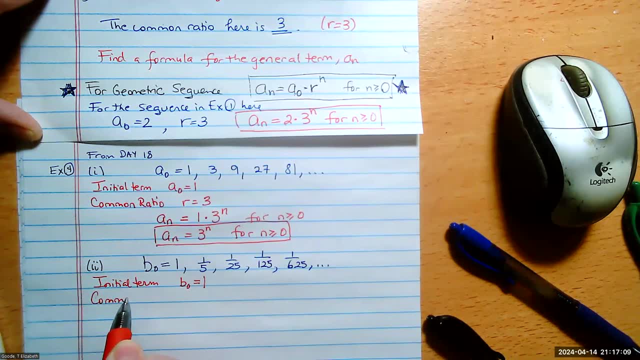 1.. Good, What's the common ratio? What are we multiplying by, over and over again, 1.. 1. fifth, So the general formula is the initial term times the common ratio raised to the n for n greater than or equal to 0.. 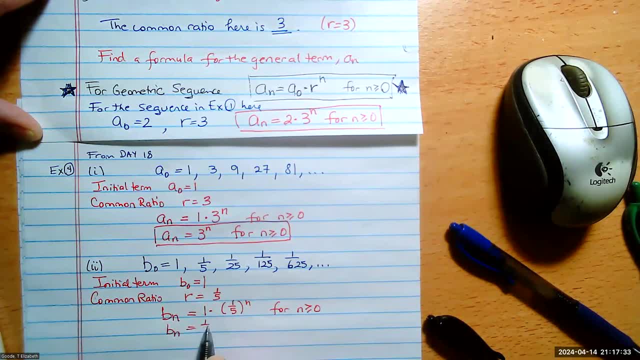 But you know, since it's just 1 times that we can just say it's 1, fifth raised to the n for n greater than or equal to 0. So those are really easy because the initial term is 1 in both of these. 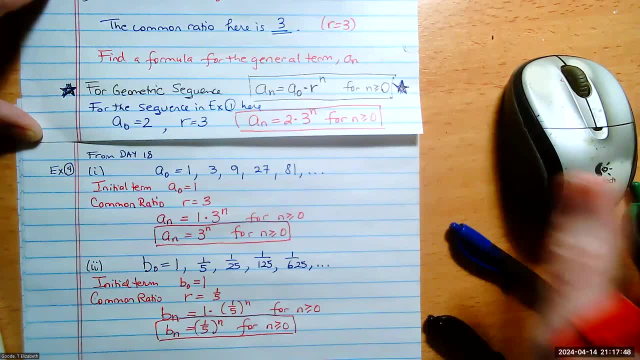 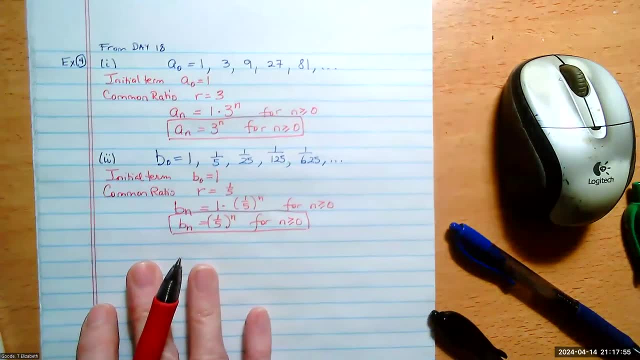 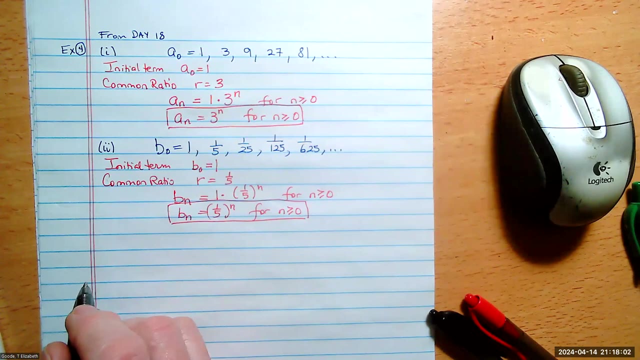 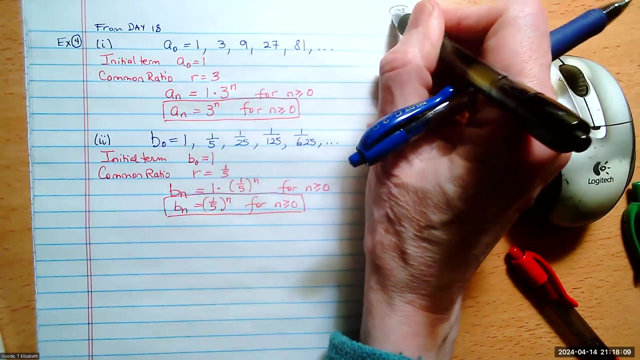 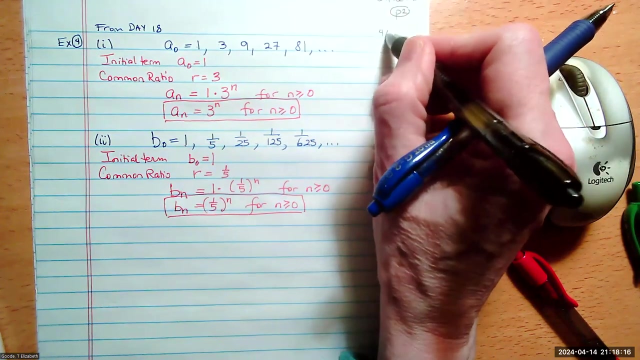 But the initial term doesn't have to be 1.. It could be something else. You need to see another one. No, thank you. All right, Next question: Okay, Professor, Good evening. Good evening, Can I ask a question from the website? 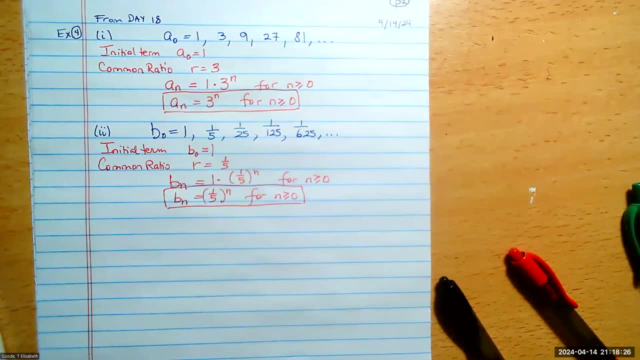 Sure, Okay, So it's number 10 on the website. All right, Section 5.1, obviously All right. So hang on, I'm going to get to that and then I'll share my screen. Okay, Thank you. 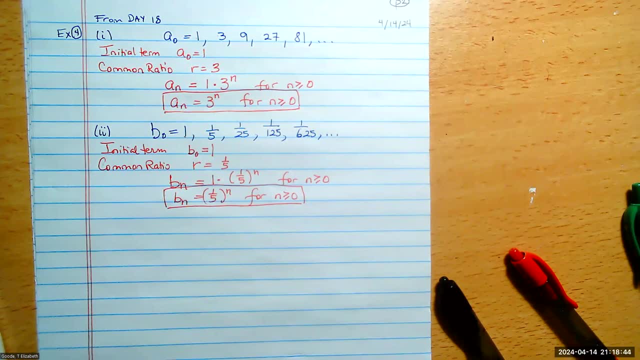 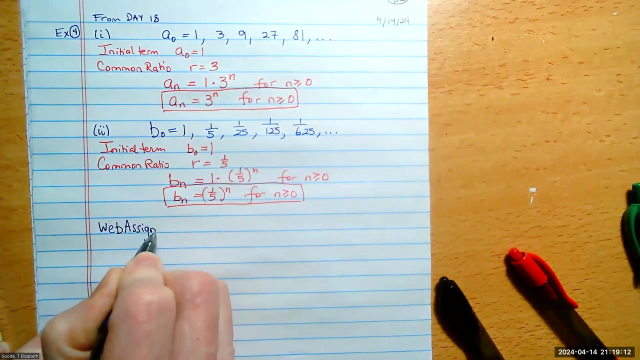 All right, Number 10.. Hang on a second. It's taking a minute for it to log in. Okay, All right, So web assign. Okay, Section 5.1, number 10.. I'm going to write down what it says. 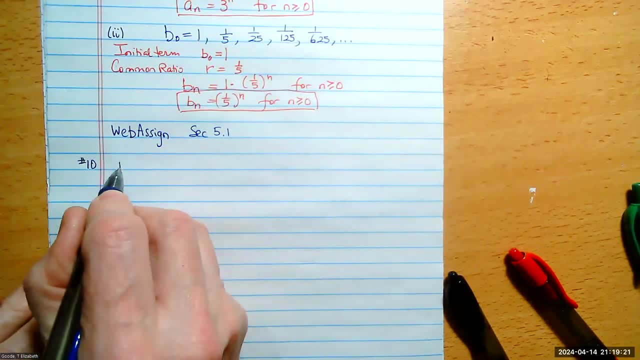 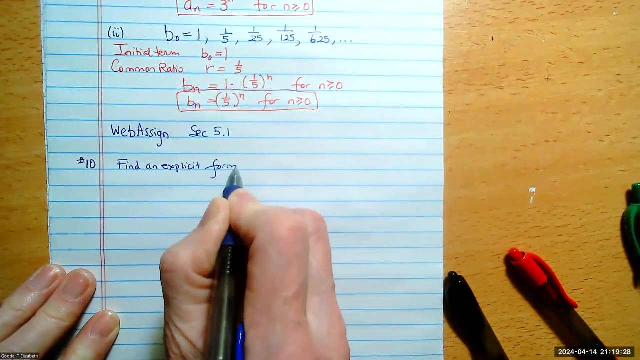 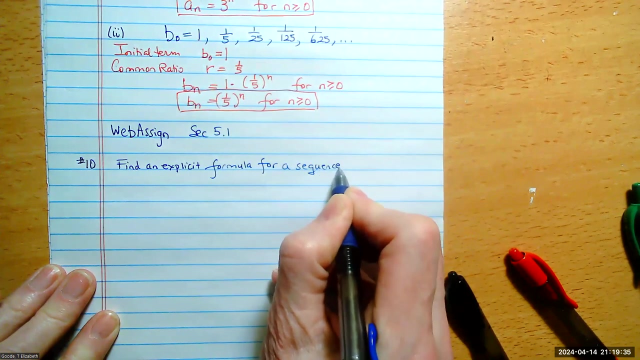 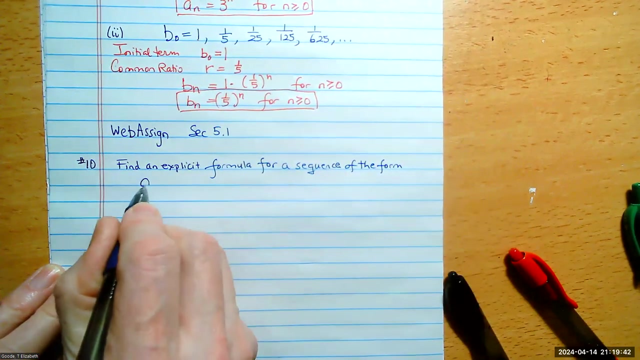 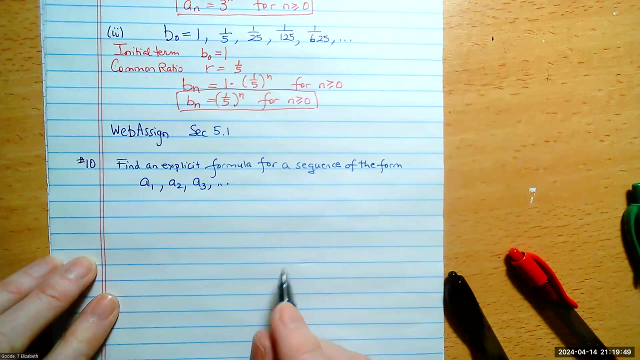 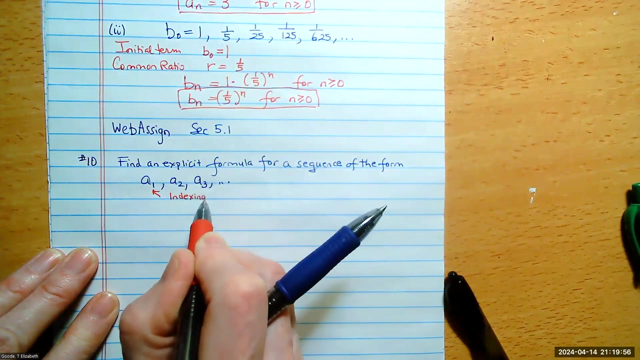 because if I show you my screen, it shows the answer. It says: find an explicit formula for a sequence of the form and it says a1,, a2,, a3, dot, dot, dot. Okay, So we're told that the indexing starts at 1, not 0. 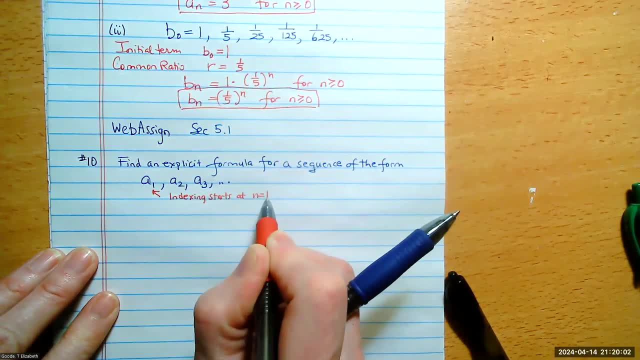 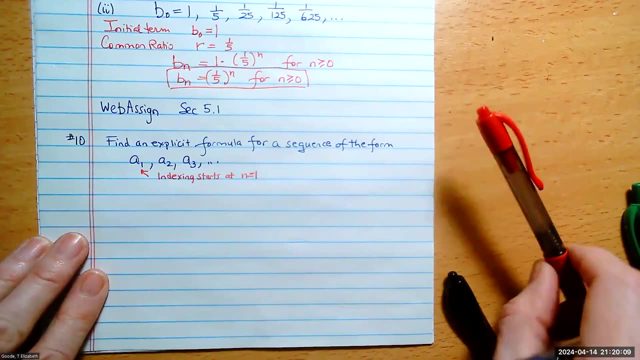 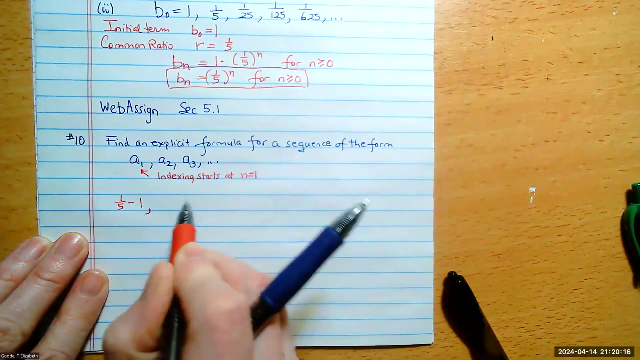 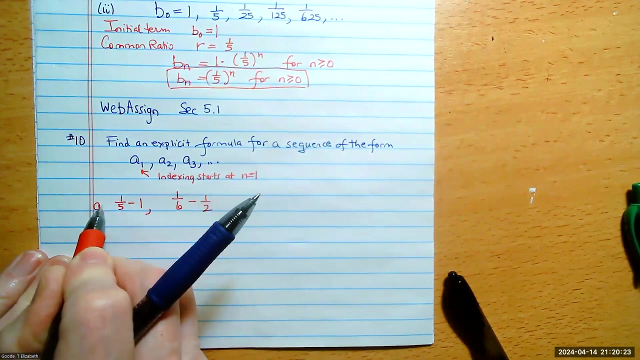 Okay, That's the first thing to understand. Does that make sense? Yes, So the terms are well, the first term is one-fifth minus 1.. The next term is what? One-sixth minus one-half. So the way we write it, this is a1.. 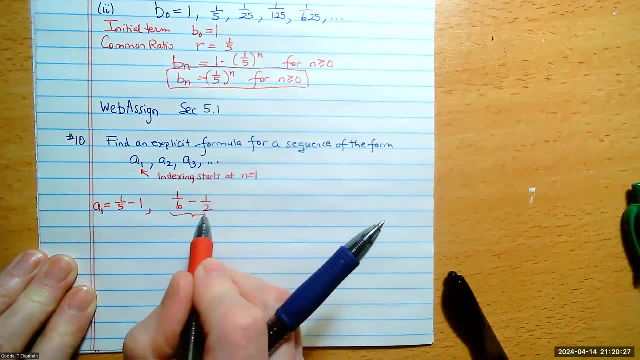 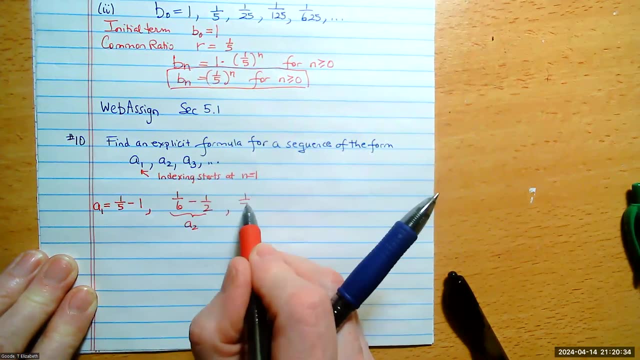 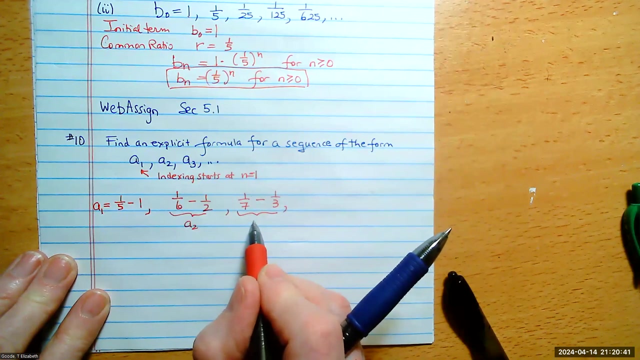 a1 is one-fifth minus 1.. This term is a2, one-sixth minus one-half. The next term is one-seventh minus one-third. Which term is that? What would we call this term, a3? Mm-hmm. 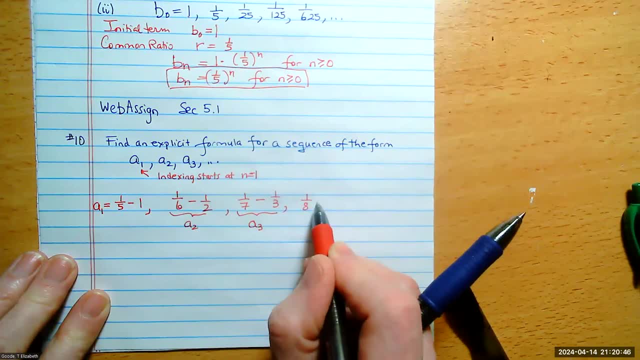 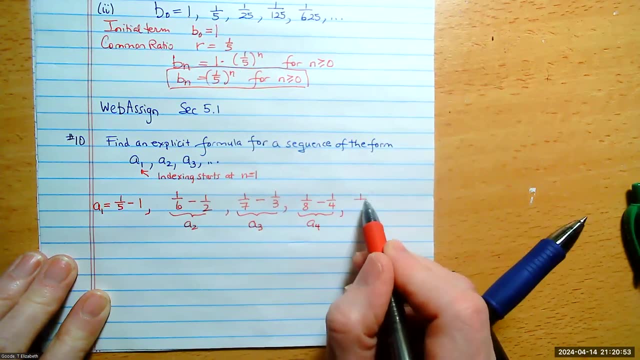 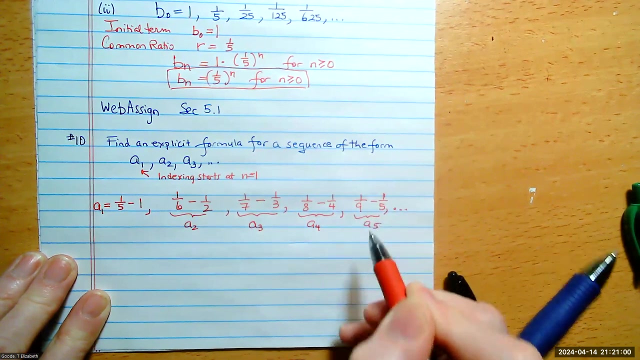 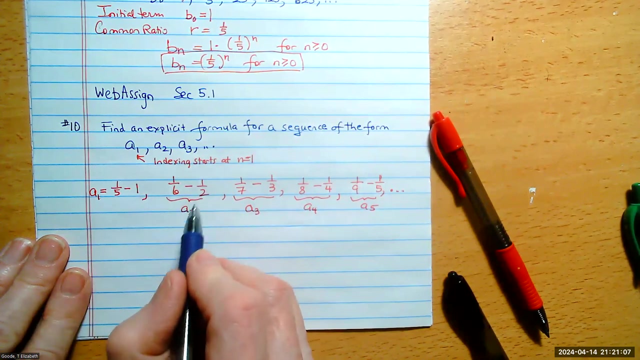 And a4 is one-eighth minus one-fourth. I'll write one more and then I think we see enough to get the drift. Okay, So we want to relate the indexing number to something that we know, To something that we see happening in the sequence. 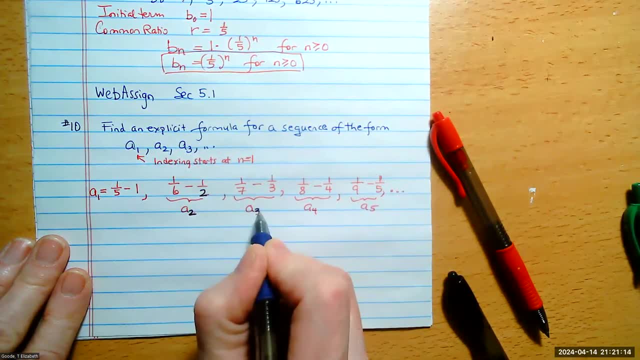 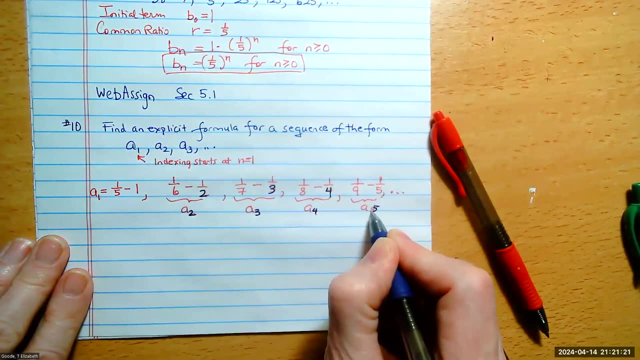 Like this 2, I see a 2 here. This 3, I see a 3 here. You see that. This 4, I see a 4 here. This 5, I see a 5 here. We still have to deal with the first part of each. 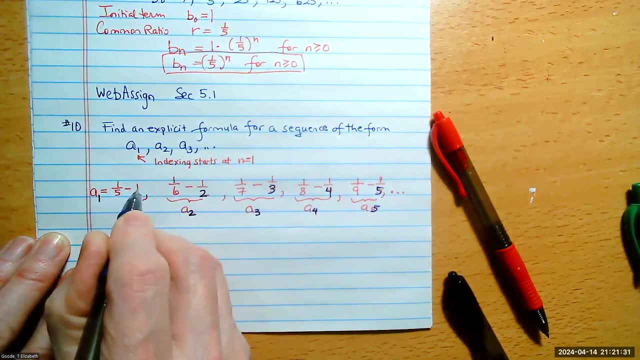 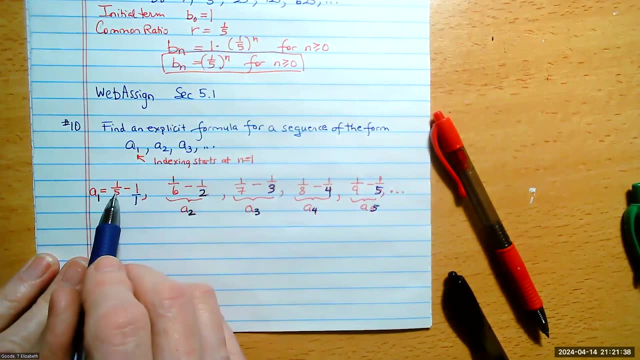 But even a1, we could write this over 1.. 1 over 1, right, Right Now we have to figure out what's going on with this other fraction. Well, they're going up by 1.. This starts at a fifth, then it's a sixth. 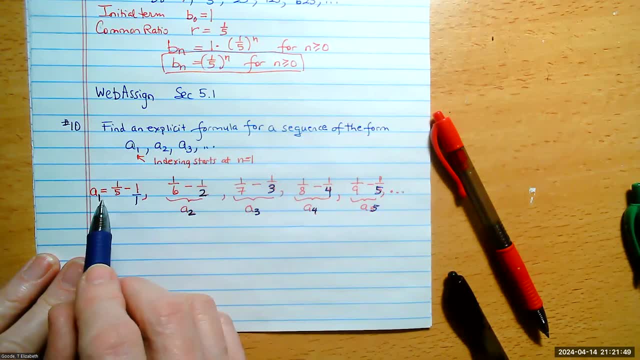 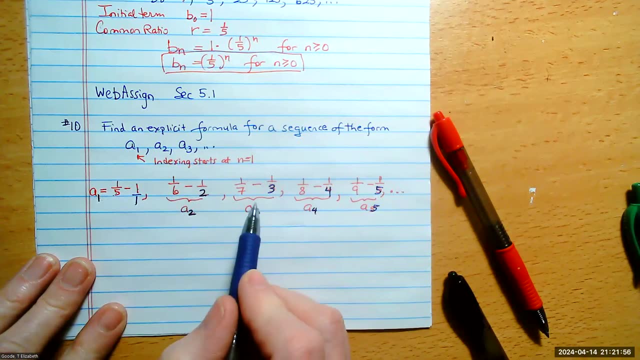 then it's a seventh, then it's an eighth. So we need to relate 1 to 5. But that relationship needs to be the same thing as the relationship between 2 and 6. And it needs to be the same as the relationship. 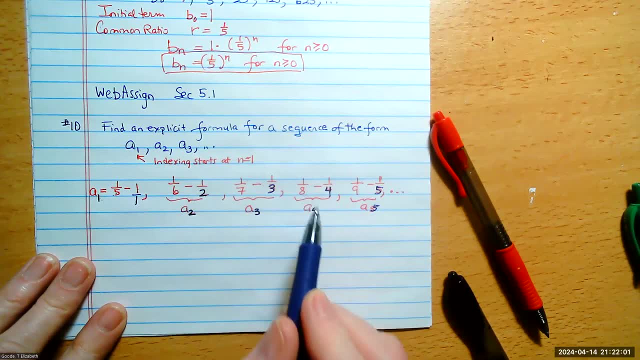 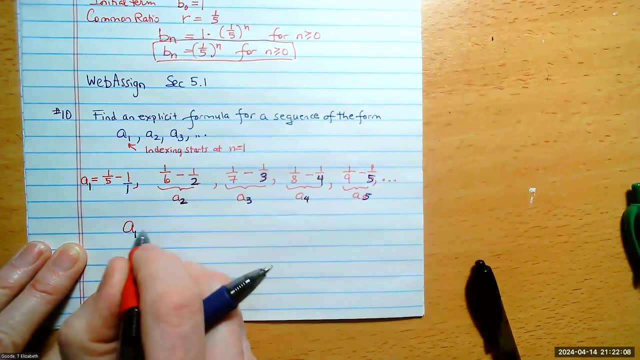 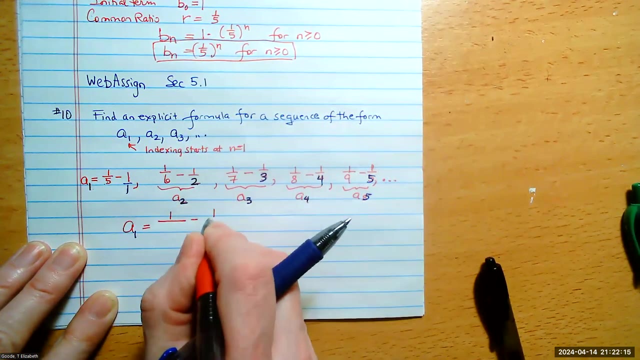 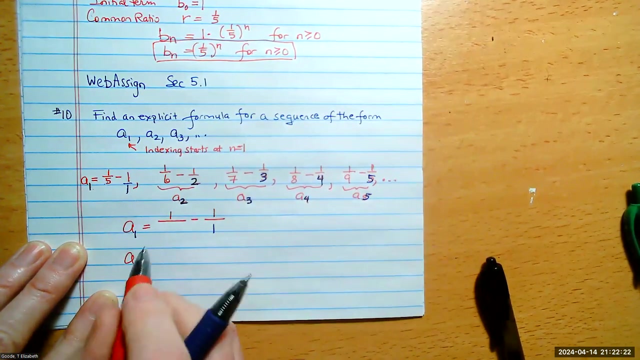 between 3 and 7, and 4 and 8, right. So a1 equals 1 over something. We need to see a 1 in here Minus 1 over the 1. a2 is equal to 1 over something. 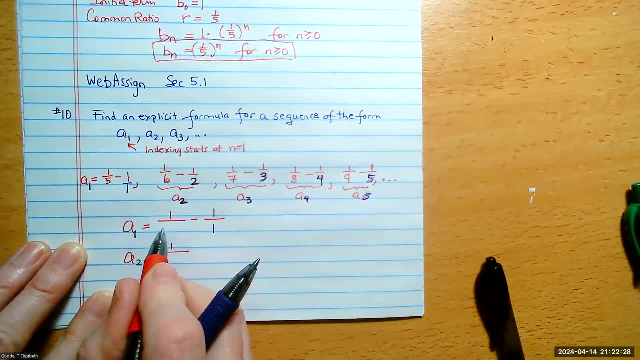 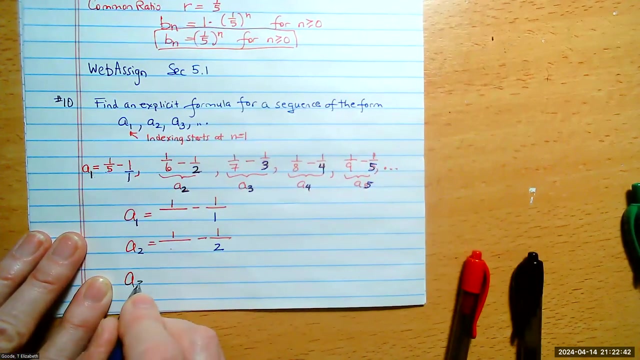 that we have to relate to the 2.. Hopefully, in the same way that we relate the 5 to the 1, is the way we'll relate to the 6 to the 2.. Minus 1 over 2.. All right, so have you figured out yet? 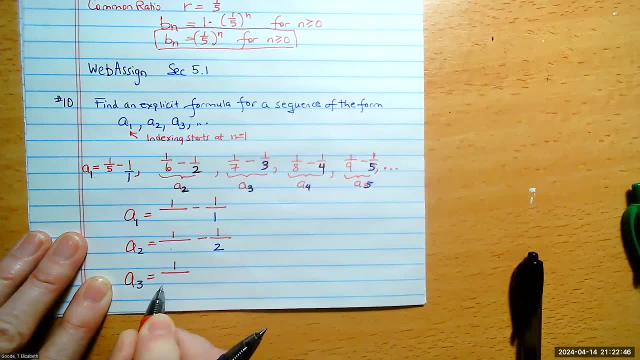 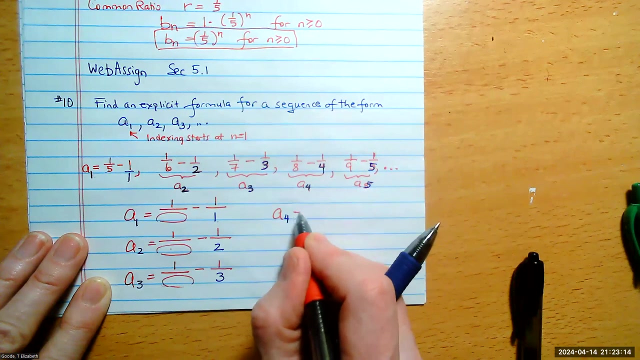 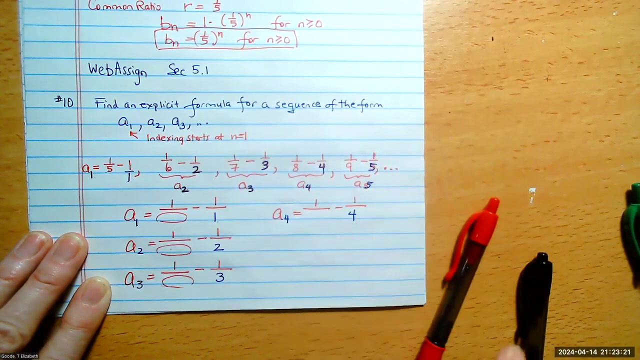 what that relationship is with the denominator that's missing here and here and here, And do you agree that this second denominator is just the indexing number? What is the relationship between these numbers- 5 and 1,, 6 and 2,, 7 and 3,, 8 and 4?? 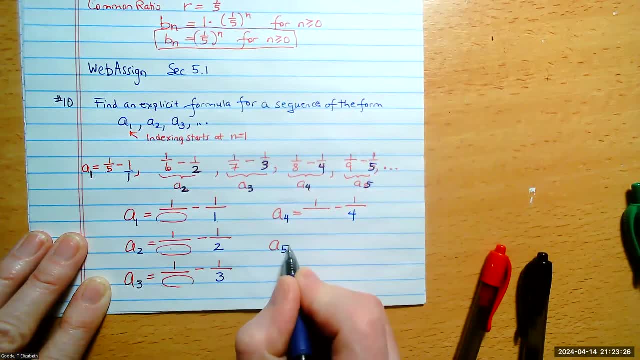 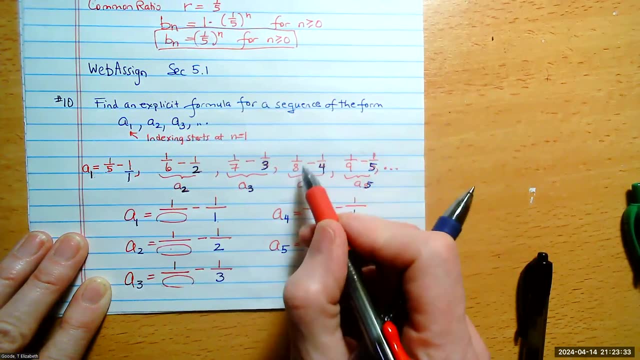 Because we're trying to figure out what's going on with this first fraction right And 9, how is it related to 5?? Hopefully it will be the same way that 8 is related to 4 and 7 is related to 3. 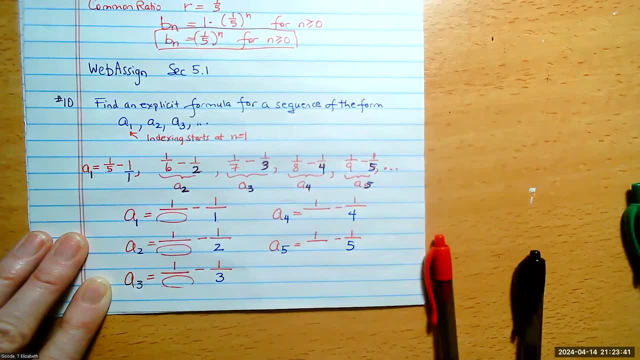 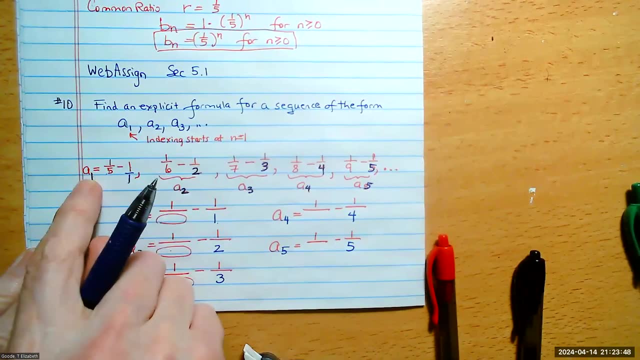 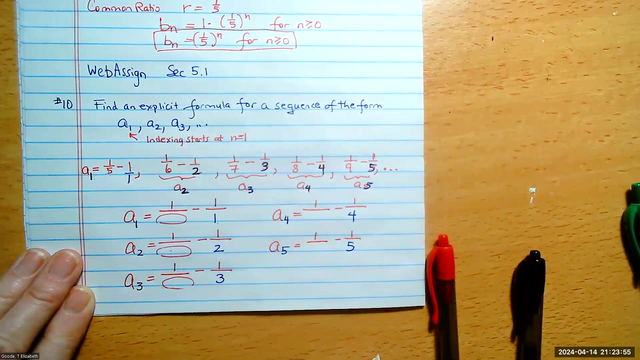 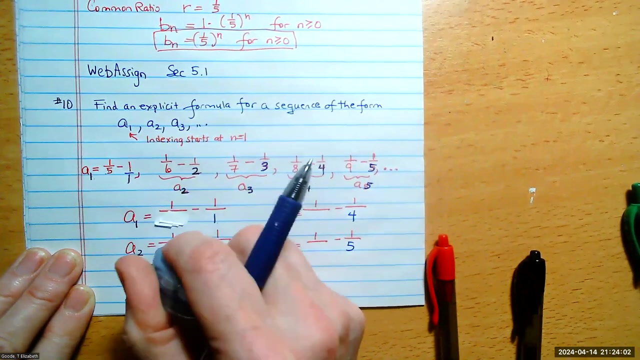 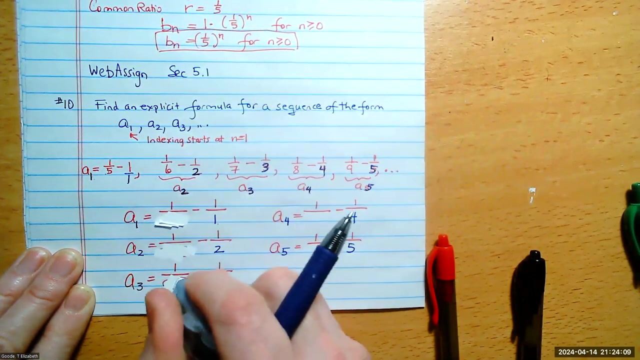 and so on and so forth. What do you think would be a way to describe the relationship between 1 and 5? that's the same as the relationship between 2 and 6 and 3 and 7? You see a pattern there. 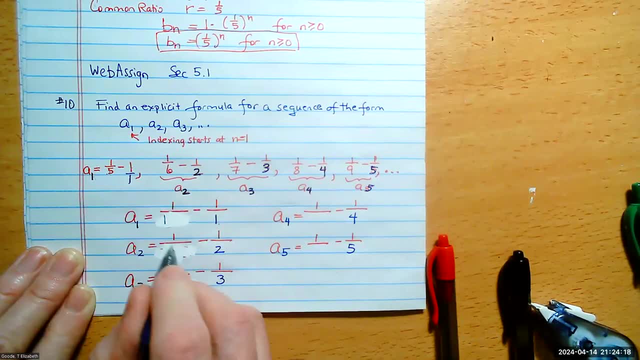 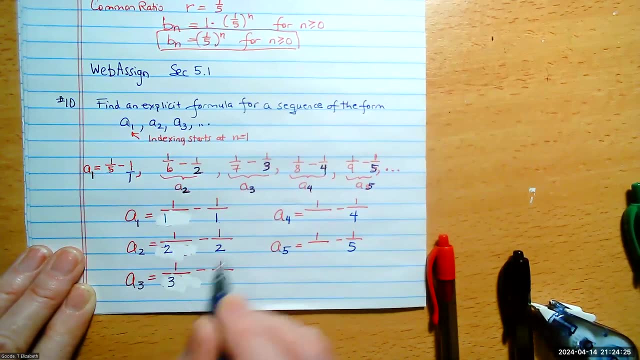 We want to see a 1 in this 5.. We want to see a 2 somehow in this 6.. We want to somehow extract a 3 from the 7., A 4 from the 8., A 5 from the 9.. 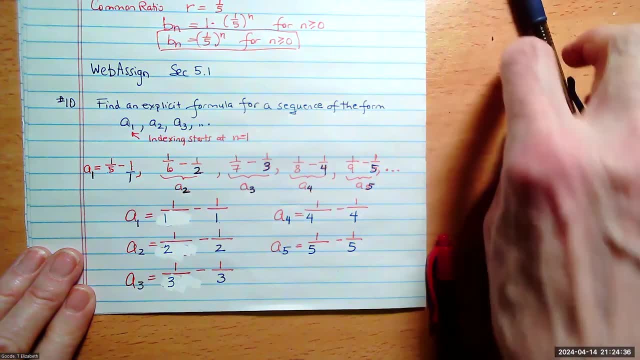 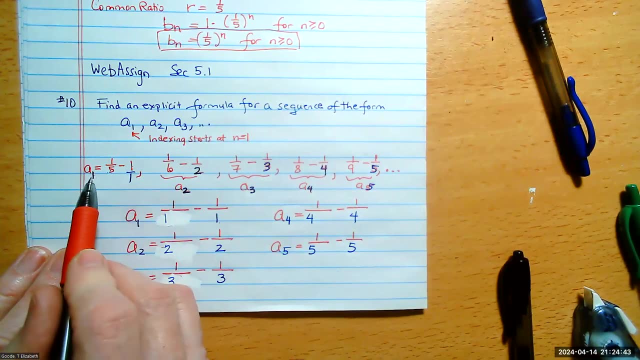 Do you see the relationship? We're looking for a pattern. How do we get from 1 to 5?? How do we get from 2 to 6?? Do we multiply by something? Do we add something? Do we subtract something? 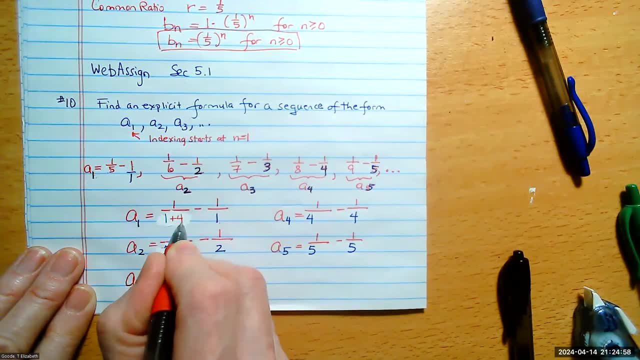 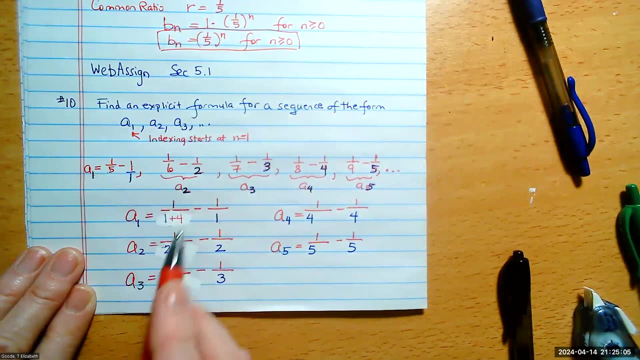 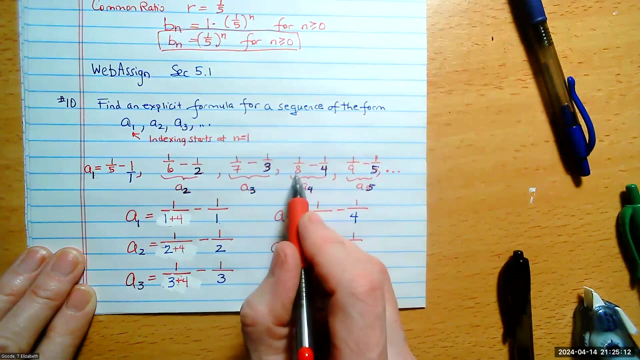 Add 4?? Yeah, add 4.. Isn't 5 equal to 1 plus 4?? Isn't 6 equal to 2 plus 4?? Isn't 7 equal to 3 plus 4?? Isn't 8 equal to 4 plus 4?? 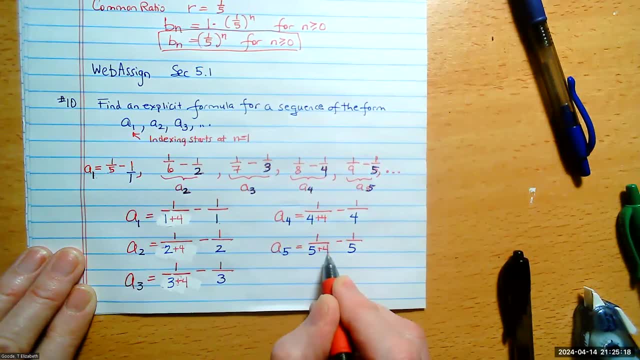 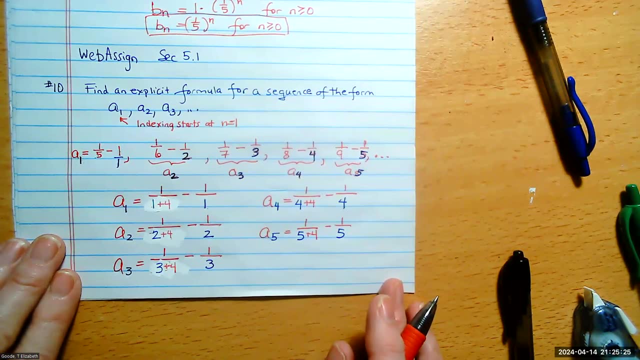 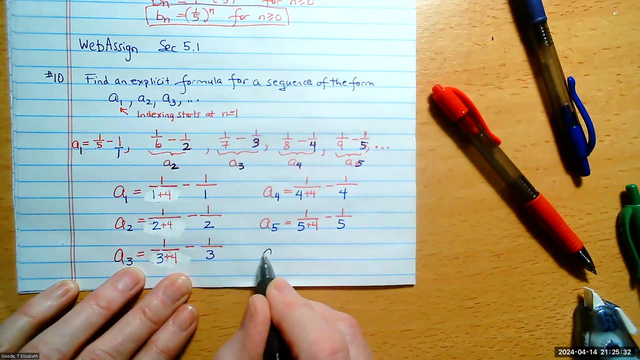 And 9 is 5 plus 4?. Do you see what's going on with that? Oh yeah, yeah, yeah. So let's write the formula for the general term: a sub n, a sub n. What do you think we should write? 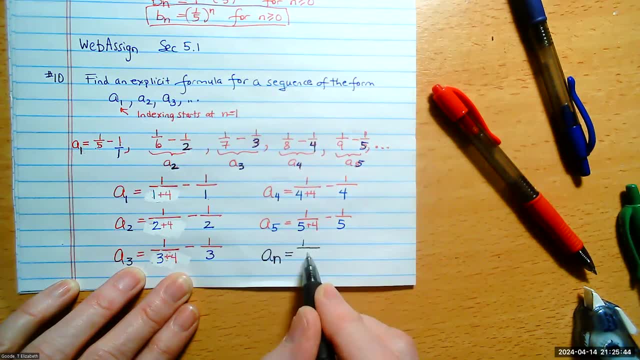 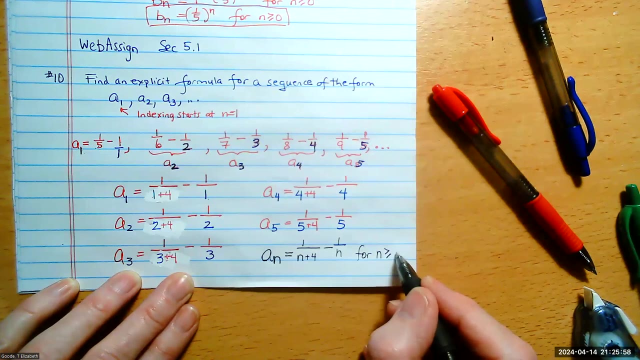 1 over n plus 4 minus 1 over n. Great, And that's 4n greater than or equal to. where did the indexing start? 5. 1. They tell us in the prop they don't write it the way I write it. 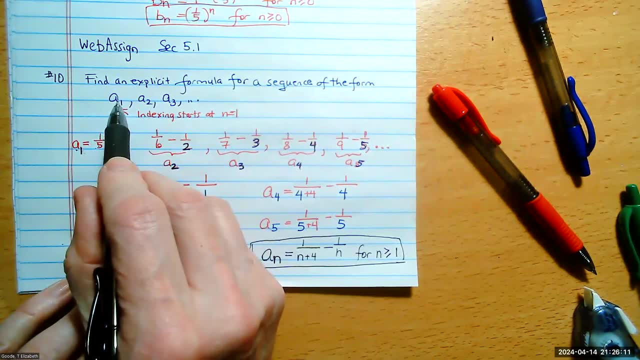 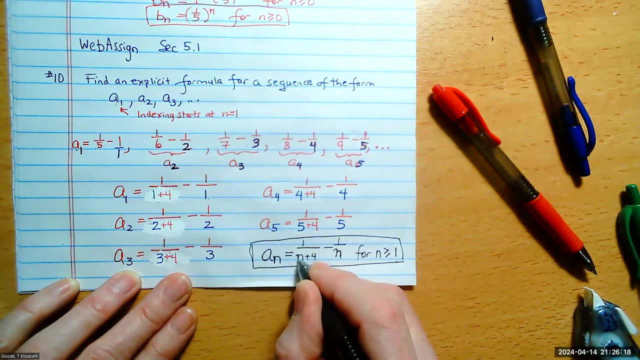 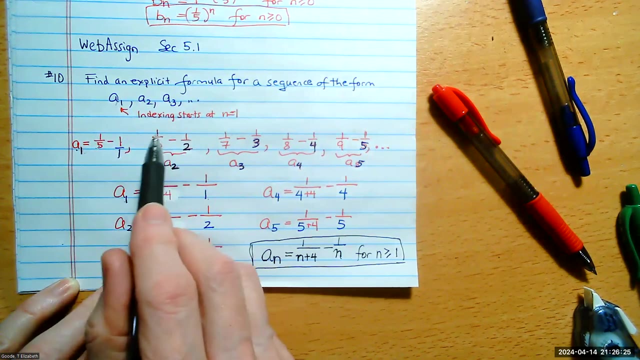 I always write it like this, But they told us here it's going to start at a sub 1.. Does that make sense? Yes, We're always just trying to look for a relationship between the indexing number and the expression. OK, Professor. 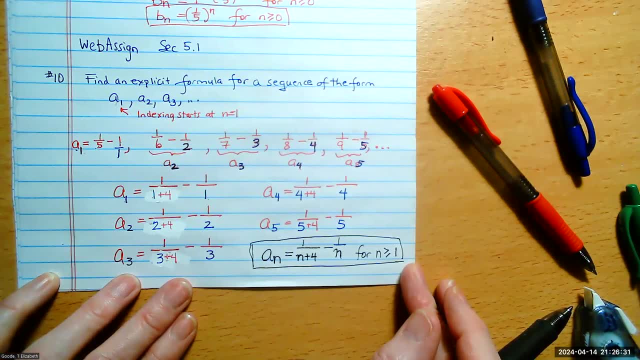 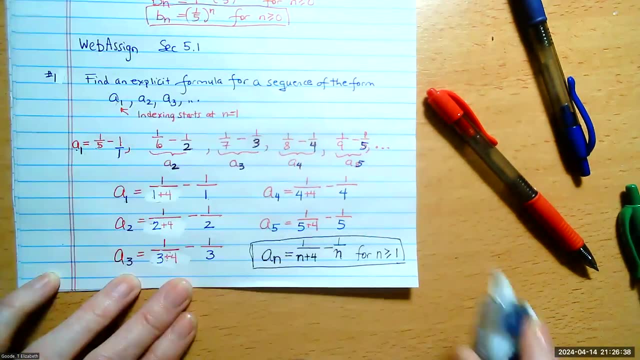 Yeah, OK, So is this for the example 10?? Because I feel like it's not the same thing. Oh, this is example 1.. That's example 10.. That's 1.. Oh my god, Yeah, All right. 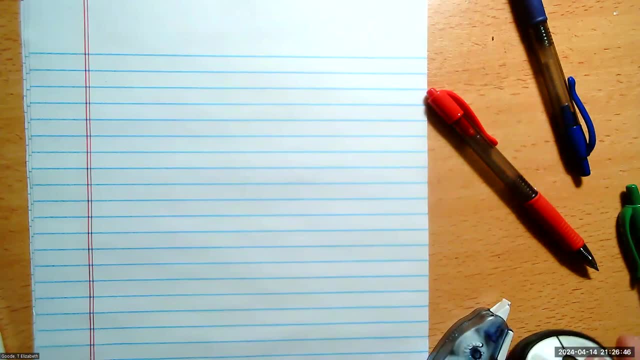 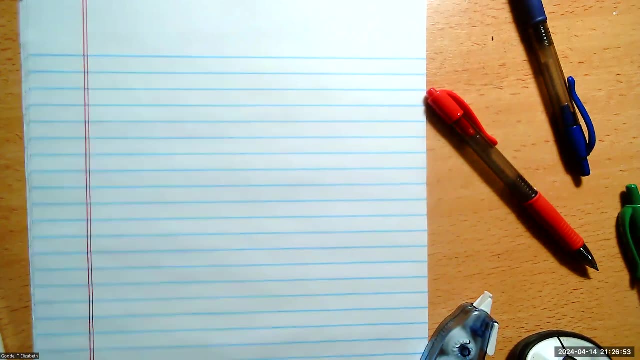 No wonder you were so quiet. Yeah, because I was confused. I stopped while I opened up Webaston. I'm like, oh my gosh, I got to Webaston. I must have been there. OK, Number 10.. 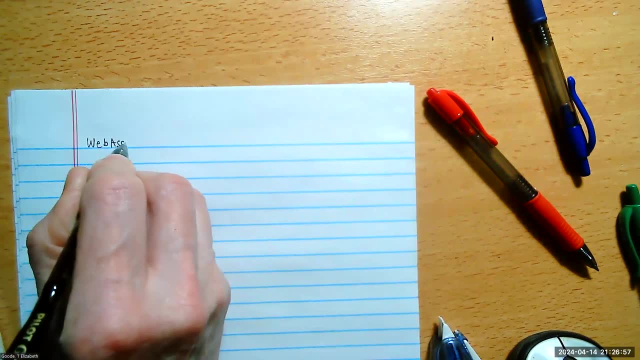 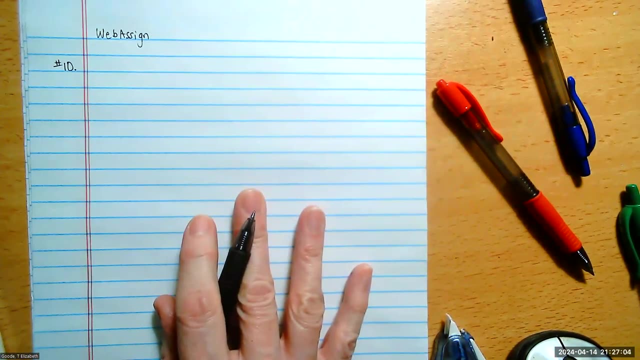 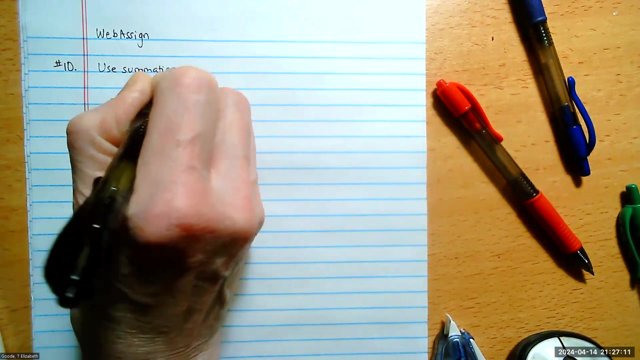 Yeah, number 10.. Thank you, I'm sorry, But that's OK. Somebody needed number 1.. I guarantee it All. right, Number 10.. It says use summation notation. OK, So we played this game in class. 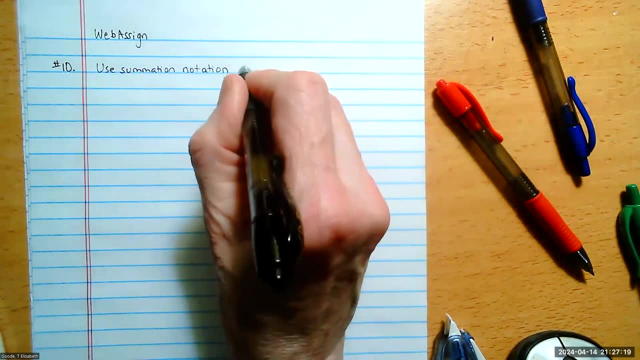 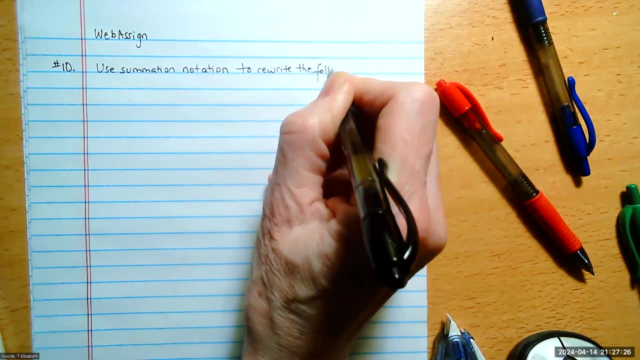 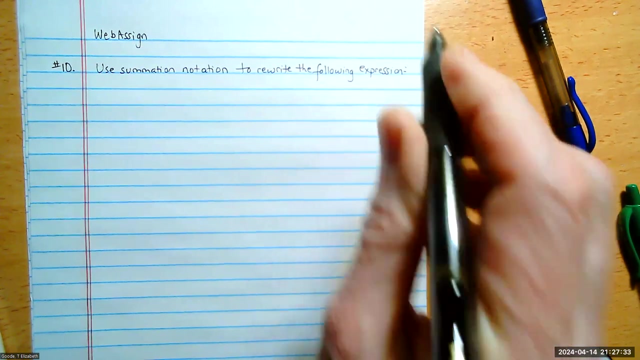 But they're all different, aren't they To rewrite? Is this the correct one? The following expression: OK, I think this is number 10.. I apologize. All right, Let's see what they give us. They give us. 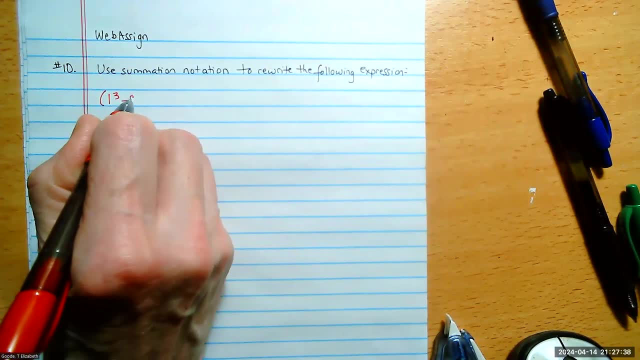 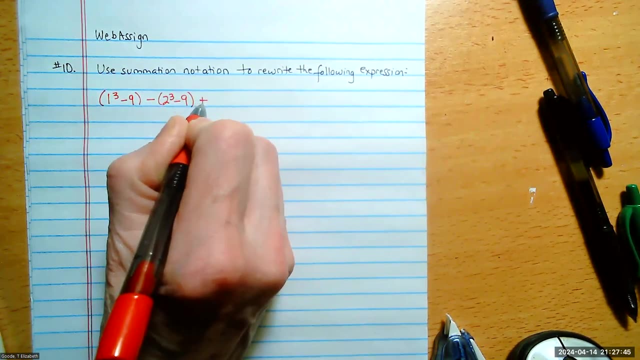 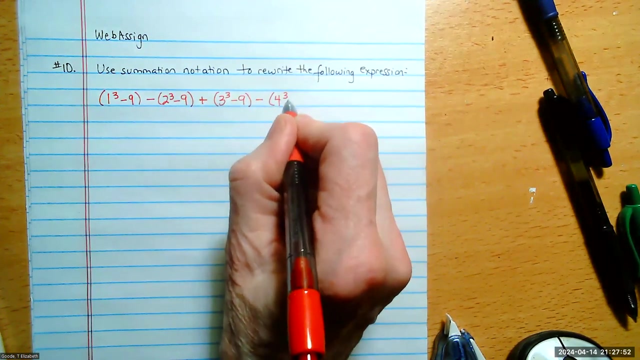 Oh, OK, They give us 1 cubed minus 9 minus 2 cubed minus 9.. Oh, it's alternating Plus 3 cubed minus 9 minus 4 cubed minus 9 plus OK, I think we see enough right. 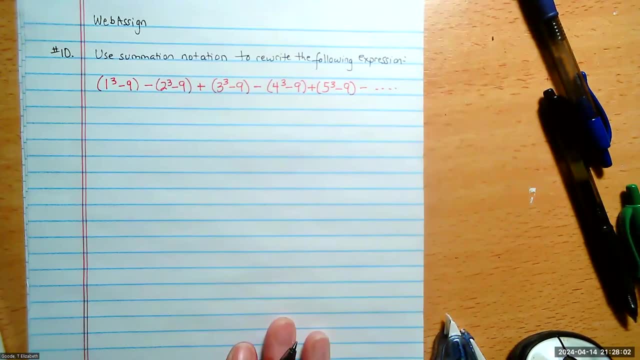 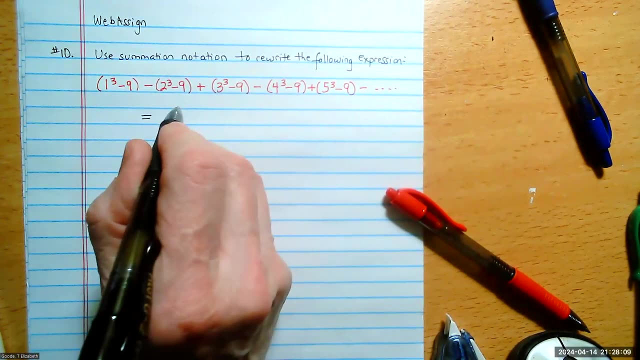 Minus dot, dot, dot, dot. right, OK, Now we have a choice. except they say: They tell us that k starts at 1.. Do you notice that They force us to use k equals 1 for the lower bound? 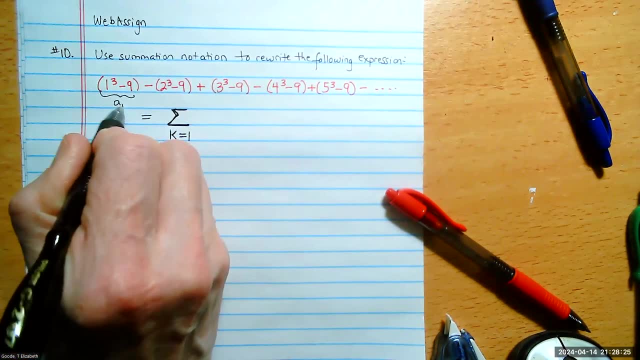 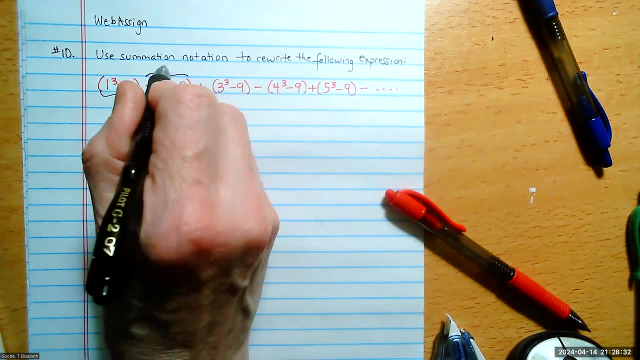 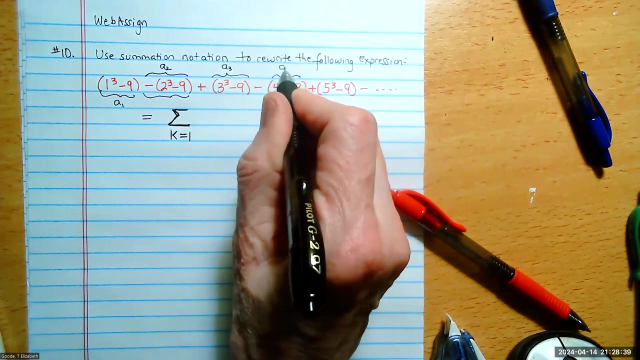 That means this term is the a sub 1 term. This term is the a sub 2 term. I better write it up here. I'm going to be in my own way. Do you understand what I'm saying? Yes, OK. 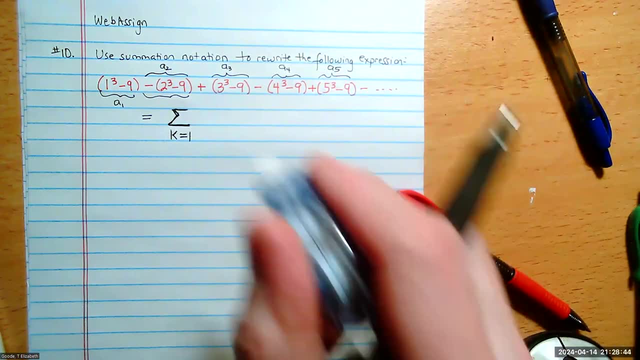 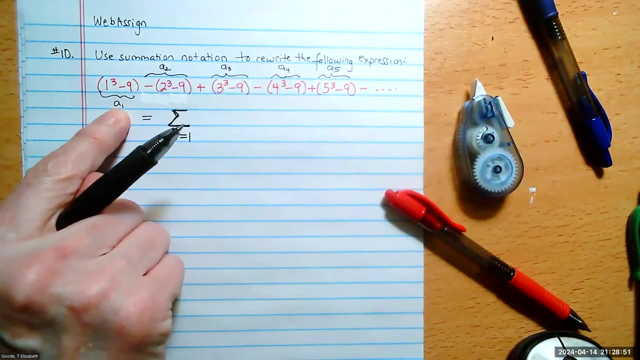 So that they're kind of giving us a clue. there They're saying: we're starting with k equals 1.. Now let's take a look. A1 is positive, See, even though we don't write it. that's really a plus here, isn't it? 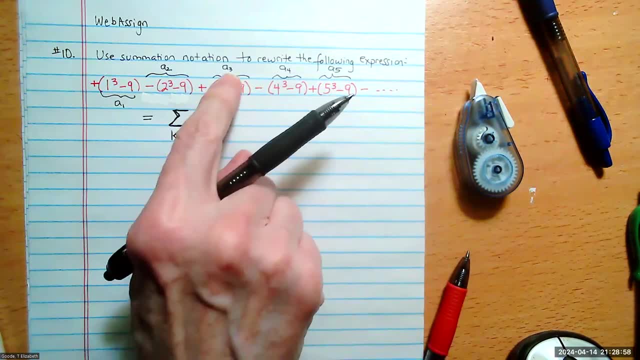 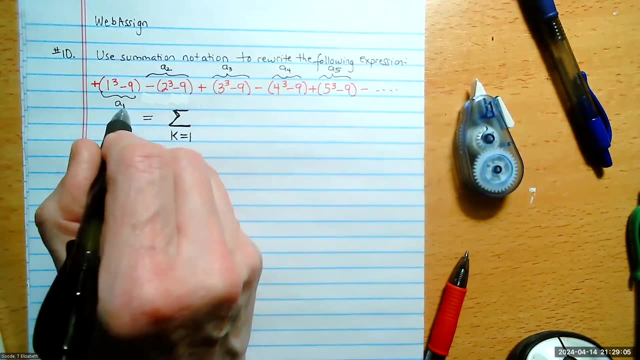 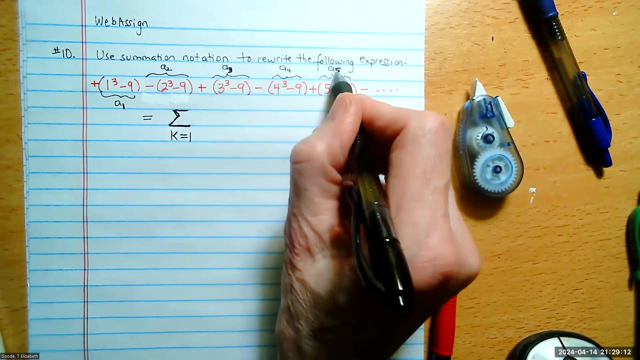 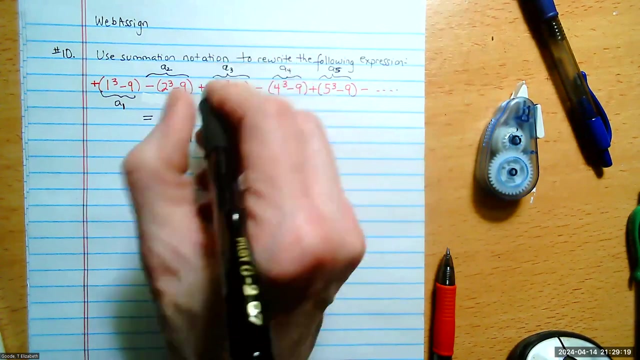 A3 is positive, A5 is positive. So the terms that have the odd indexing numbers 1,, 3,, 5. They're the ones that are the positive terms. So that means when we take negative 1, we're going to raise it either to k. 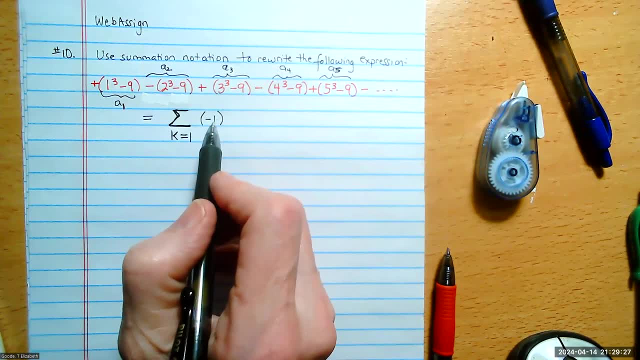 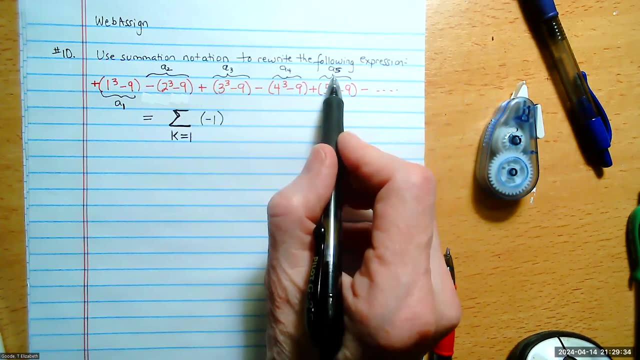 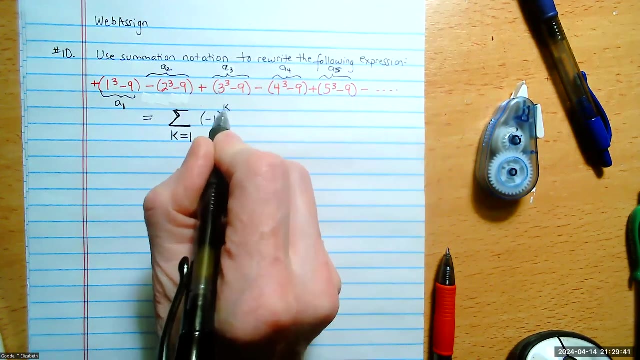 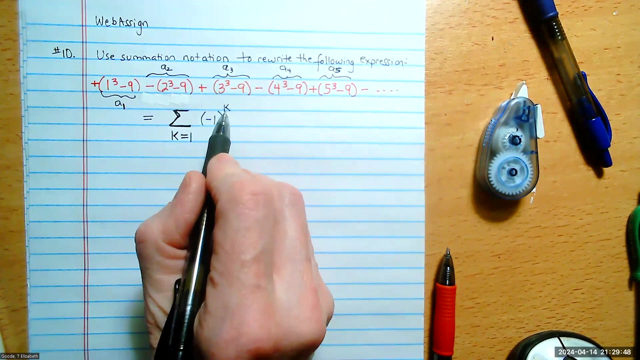 or to k plus 1.. OK Yeah, Which is going to work to make the terms that are odd indexed to be the positive terms. Let's think about it: If we just used k here, right, When k is 1, we raise negative 1 to the 1.. 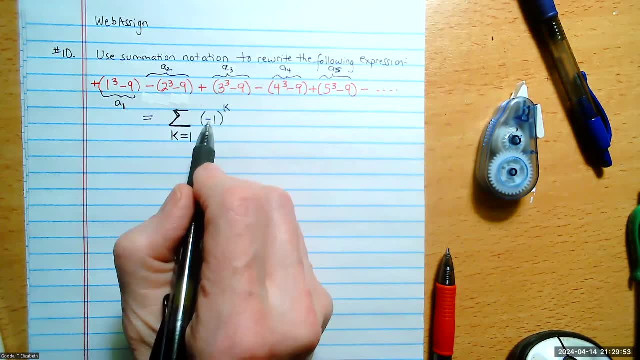 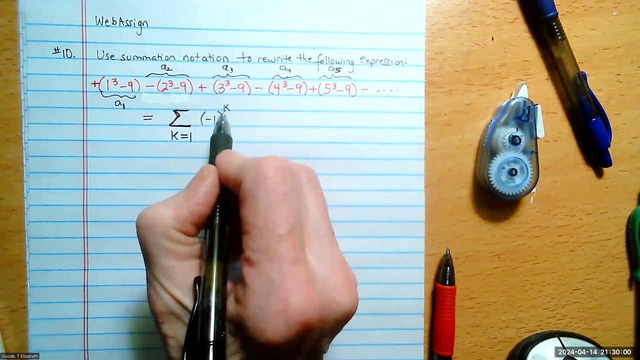 What is that? Is it positive 1 or negative 1?? We raise negative 1 to the 1. It's negative 1.. It'd be negative. And see when k is 3,. if we raise negative 1 to the 3,, would it be positive 1 or negative 1?? 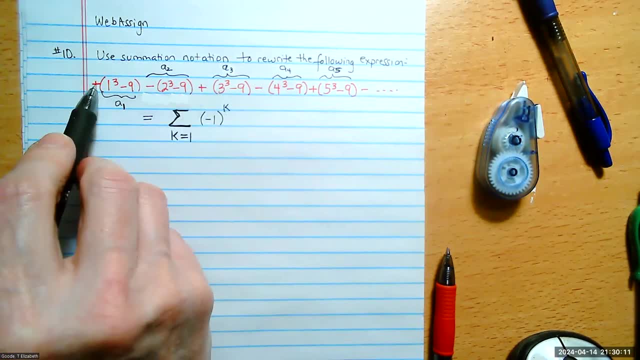 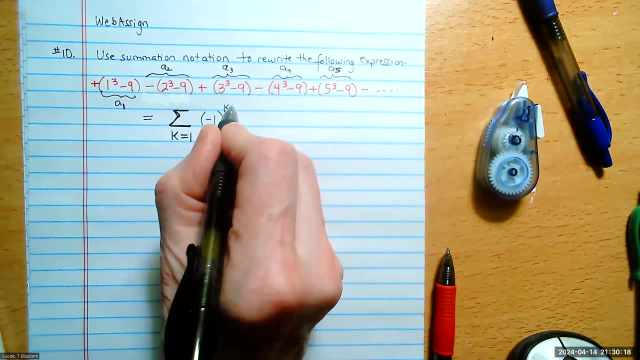 Negative, Yeah, And that's not what we want, is it? Yeah, Because we want the odd indexed terms to be the ones that are positive. So the way we adjust it is: we add 1 to the exponent And that adjusts it right. 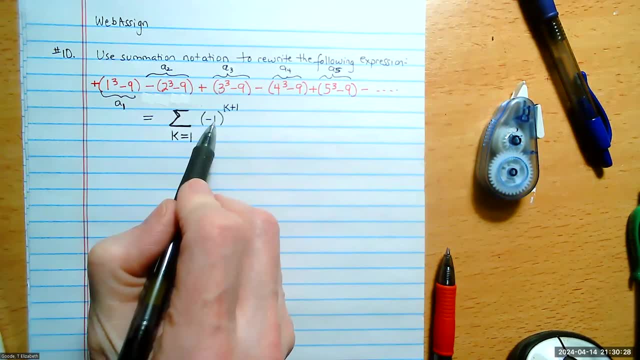 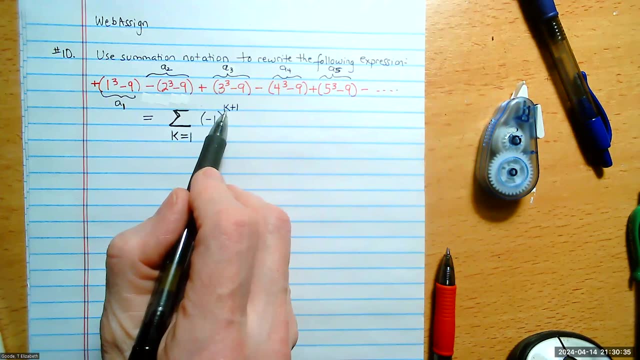 Because now, when k is 1, what is negative? 1 raised to the 1 plus 1? It's negative, 1. It's positive. Yeah, So when the odd indexed terms are the ones that are the positive terms we know we have. 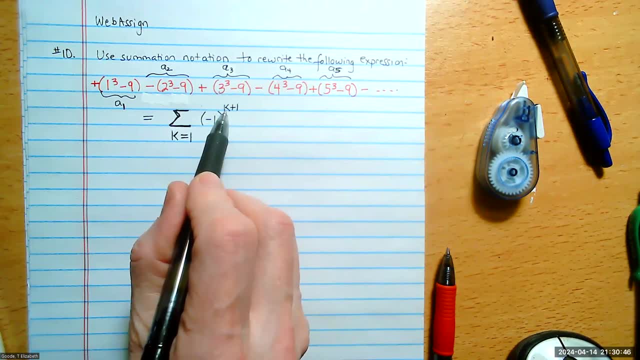 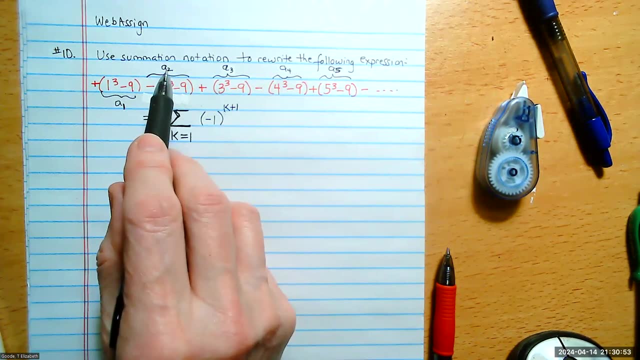 to raise the negative 1 to the indexing number plus 1.. OK, So we've got the sign right. It works for the evens too, Because, like when k is 2, we raise negative 1 to the 2 plus 1.. 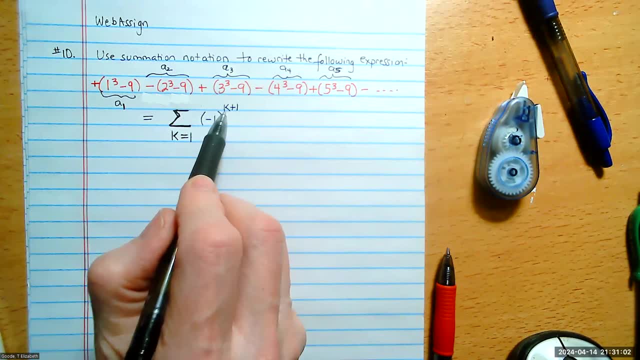 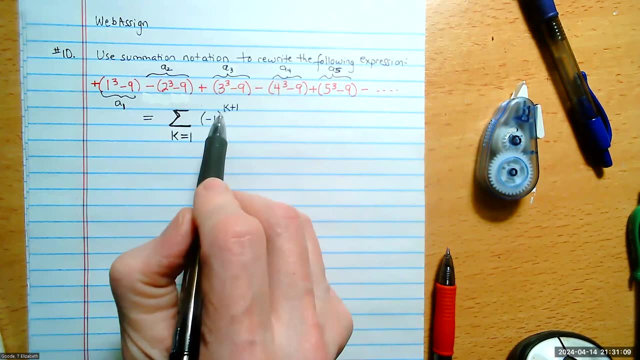 We're raising negative 1 to the 3.. And what is that Negative? Yeah, See, And it works for 4.. When k is 4, then we're raising negative 1 to the 4 plus 1.. We're raising negative 1 to the 5.. 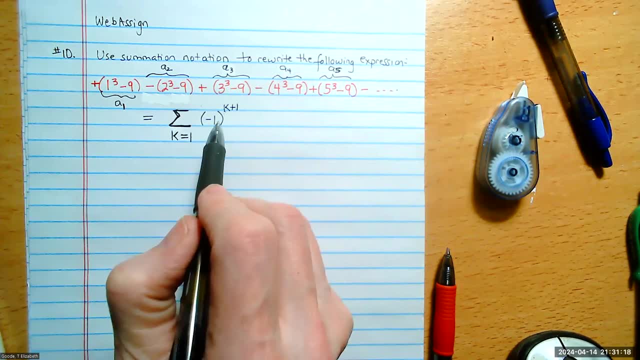 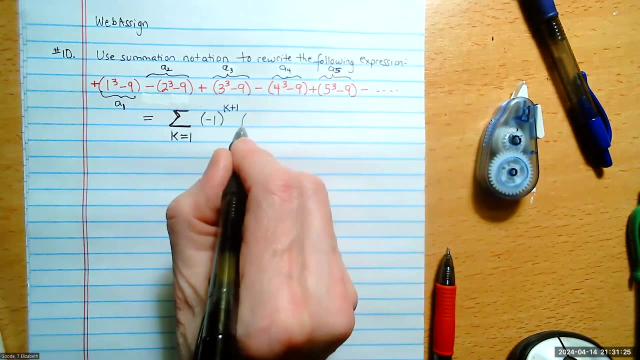 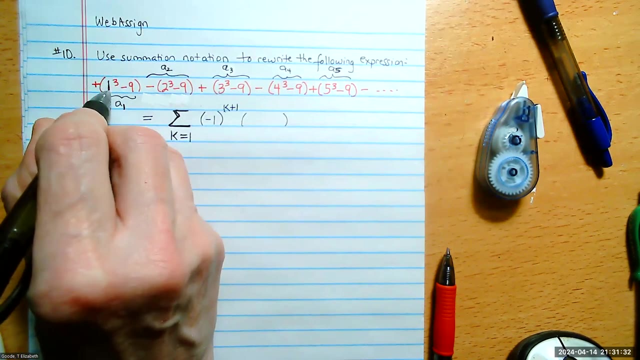 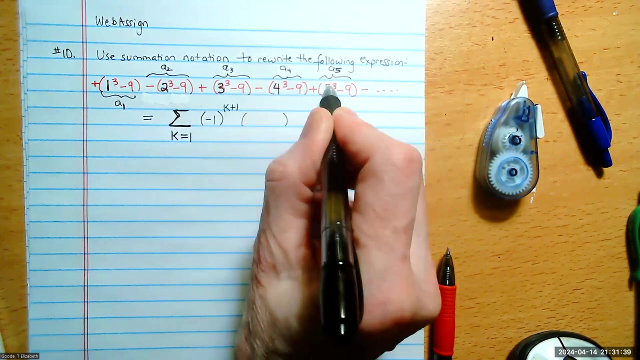 And we get the negative. Yeah, So we got the sign right. Awesome. So how do we get this expression? Well, that's pretty easy. Yeah, What does the expression look like? See, the indexing number shows up here as the base. that's getting cubed right. 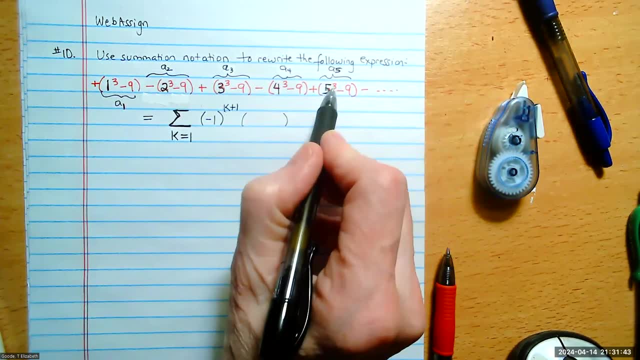 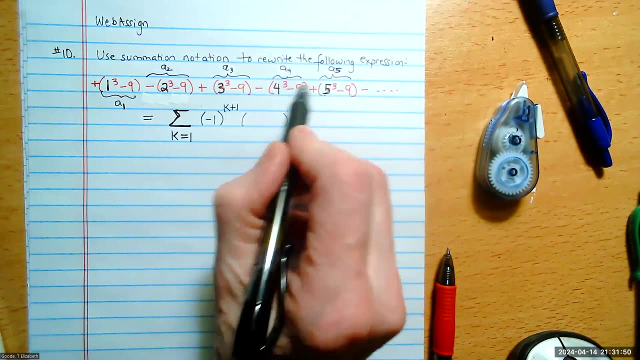 See the indexing number showing up here. This is called the base. The thing that gets raised to a power is called the base. When k is 4, it's 4 cubed. When k is 5, it's 5 cubed. 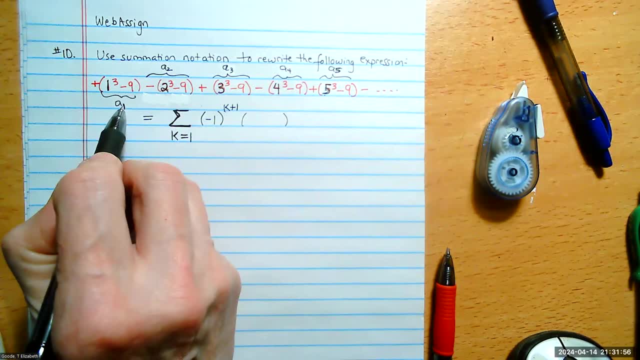 When k is 3, it's 3 cubed. When k is 2, it's 2 cubed. right, When k was 1, it's 1 cubed. So what would be the expression we want to put inside the parentheses? 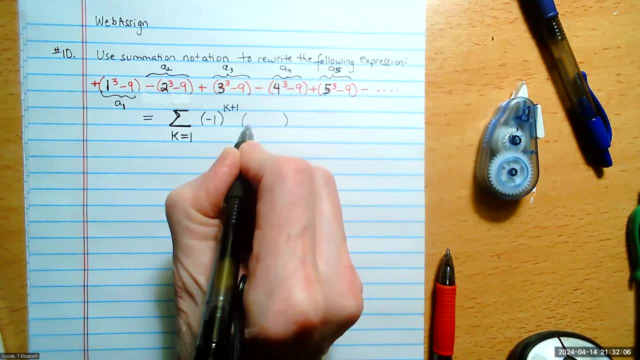 Probably n raised to the power 3 minus 9.. I think we better use a k because k Oh k, My bad. Yeah, I mean they picked it. They told us right. We're going to use k. 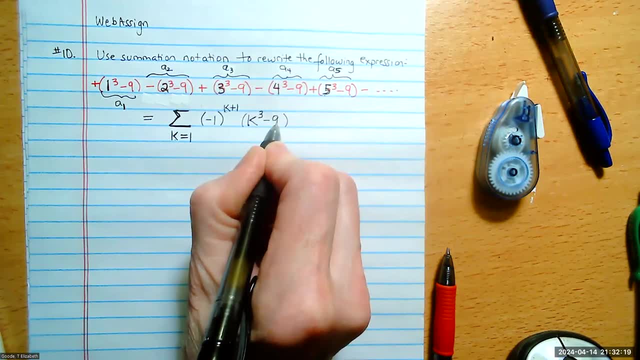 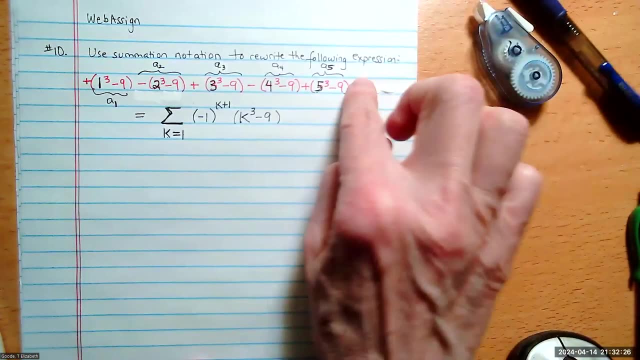 So k raised to the 3. Yeah Minus 9.. Great, Now, oh, this thing actually ends. Oh yeah, This is finite, right, Because they end it. Let me go ahead and write the rest of the terms. 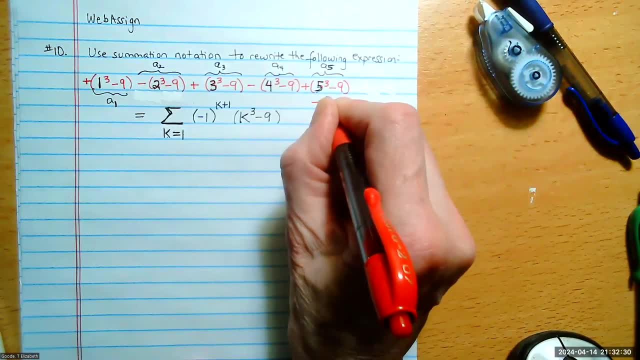 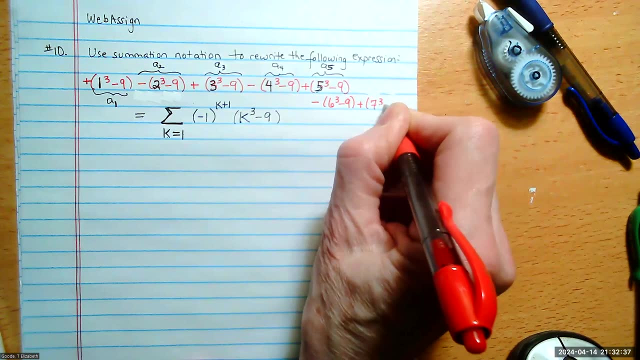 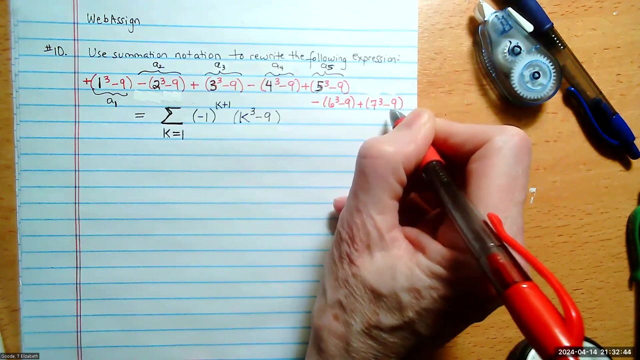 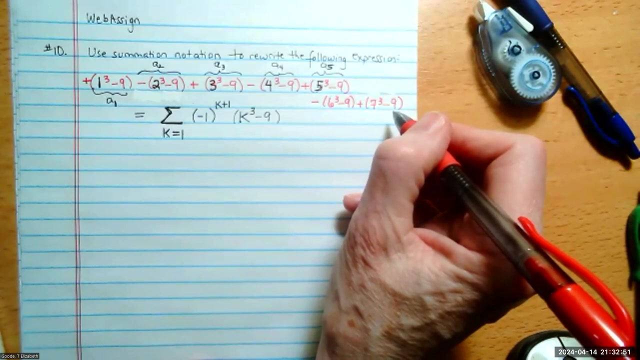 It's not infinite, It doesn't go on forever. It's like minus 6 cubed minus 9 plus 7 cubed. Is that the last term, 7 cubed minus 9? I think it is. You know, I think minus is different, but it's 6.. 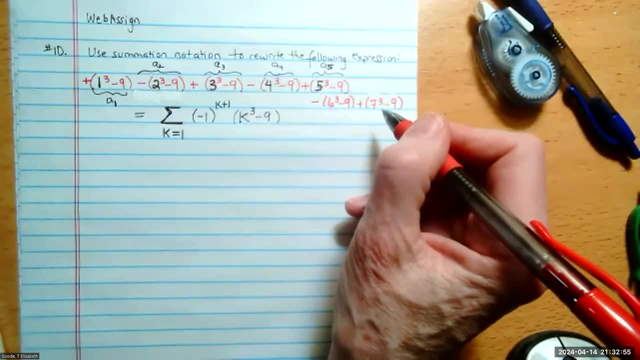 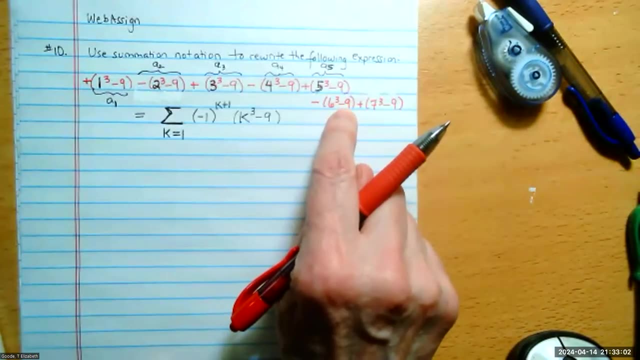 Oh yeah, You know what. This might be, one of those problems where everybody gets a little bit different, right? Does yours end at 6 cubed minus 9?? Are these signs right for you? Because some of these signs are different. 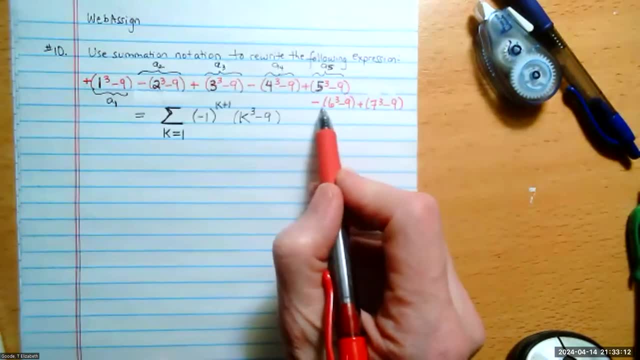 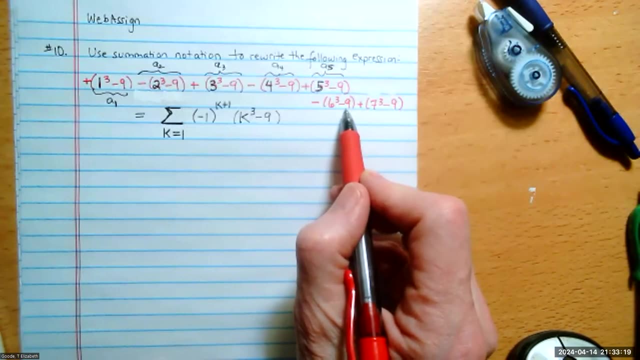 All right, Does your start. The last sign is minus, though, But it's okay. What's the last term? Is the last term 6 cubed minus 9?? The last sign is 4 minus 6 cubed, All right. 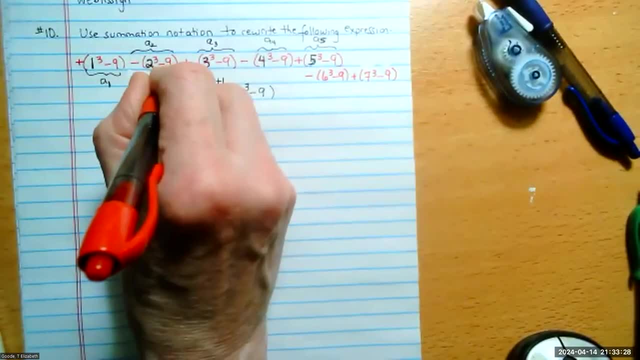 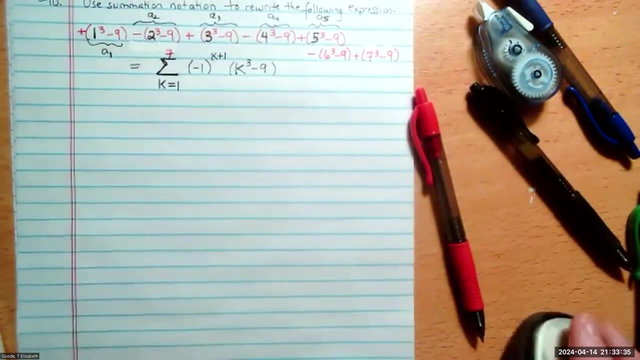 See mine looks like this And see mine ends at 7.. Mine ends at k equals 7.. Can you tell me what you want Here? I can make you the co-host and you can share yours if you want. 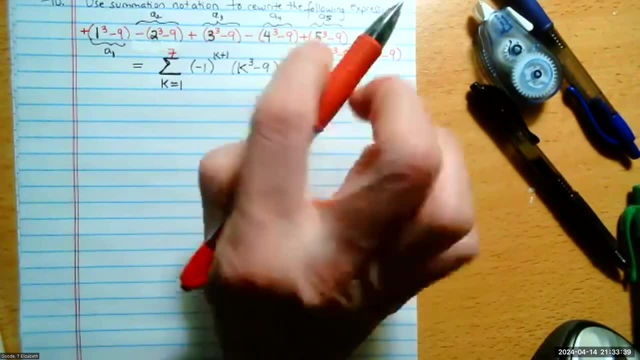 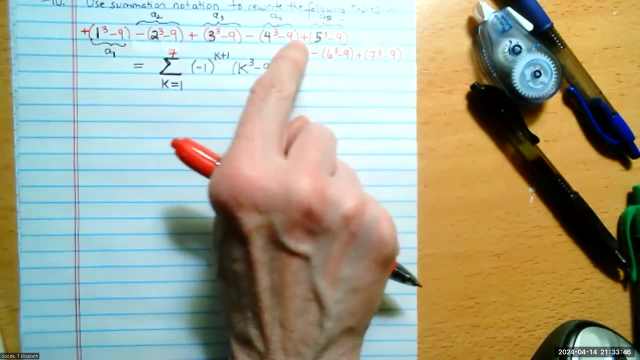 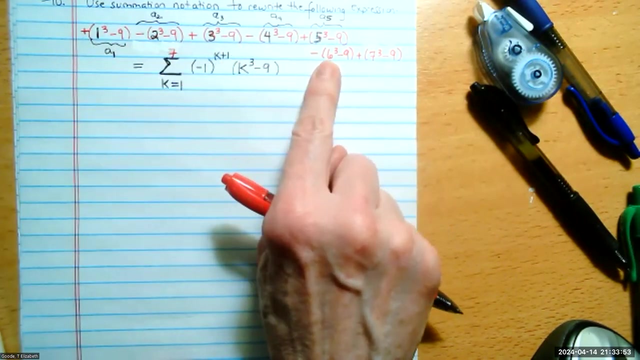 Mine ends at 6.. 1,, 2,, 3,, 4,, 5,, 6,. yeah, Yours ends at 6?. Yeah, Mine ends the same as mine. Let me see: Minus, minus, plus, minus, plus, minus. 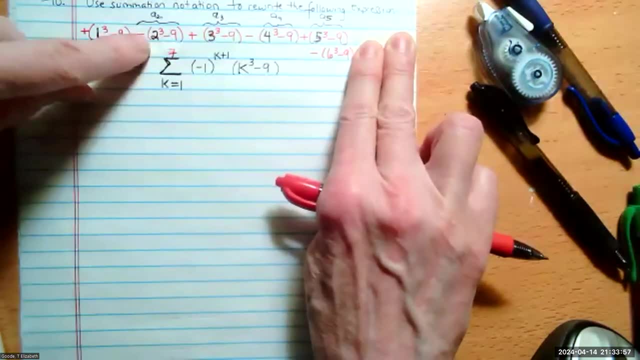 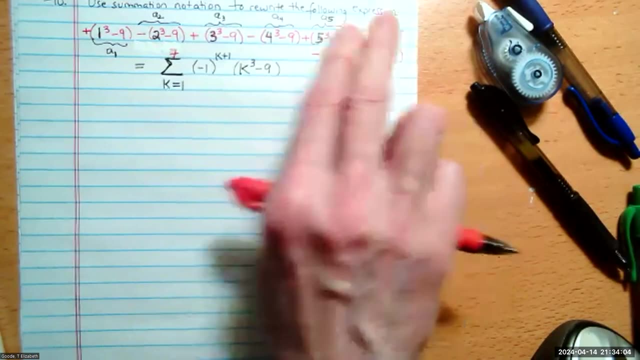 Yeah, So it's the same thing without the last one. Yes, So what? would the upper bound of your sum be 6. 6. It'd be 6.. Okay, All right. So Emmanuel and Joshua, does your problem? 10 and Webison look like this, but maybe it. 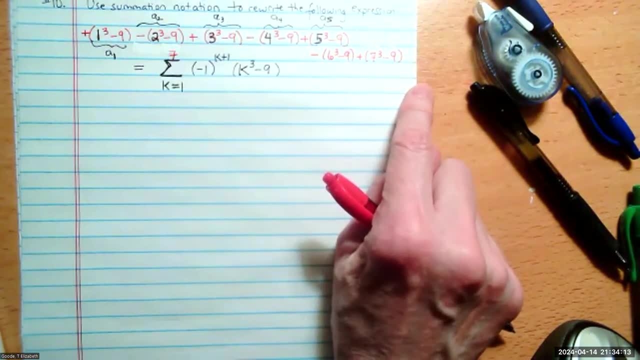 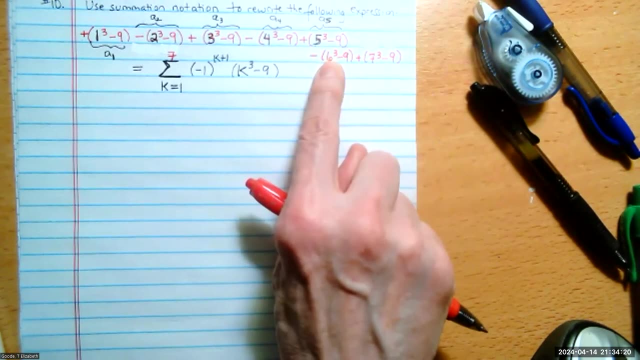 ends somewhere different. Mine looks like yours. All right, So yours goes to 7.. How about yours, Emmanuel? 6.. Yours ends at 6.. Okay, So you know these people that make up these Webisign problems. you know they try to make. 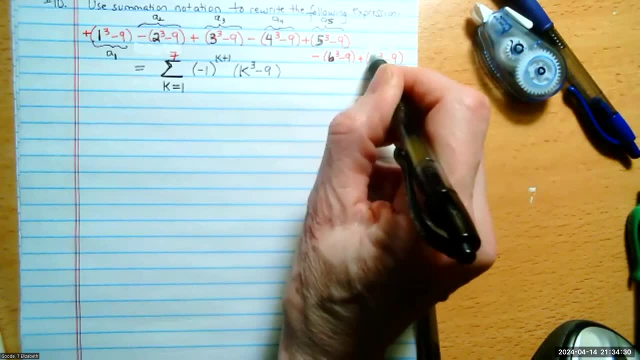 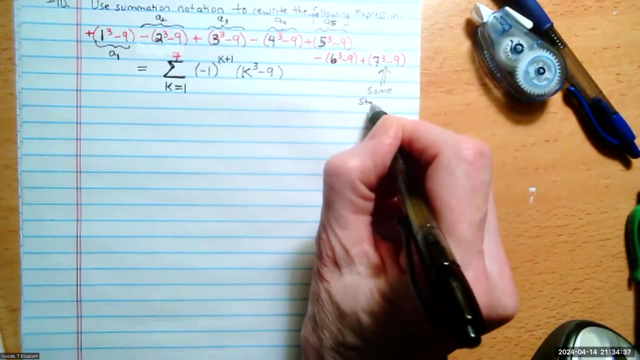 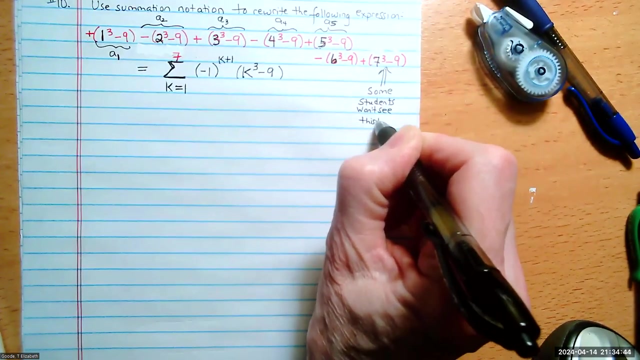 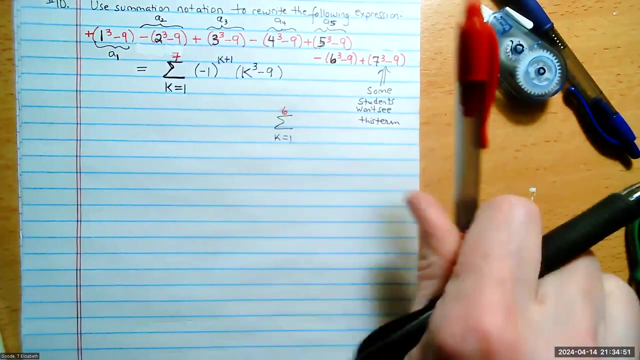 them sometimes so that they're a little different for different students, but it looks like they just gave two choices. You know some people don't have this term, Some students won't see this, In which case it's: the sum from k equals 1 to 6.. 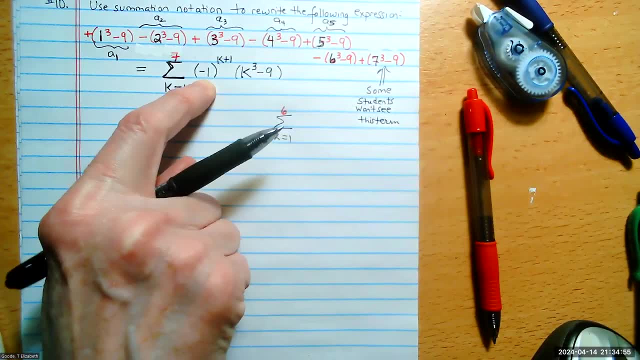 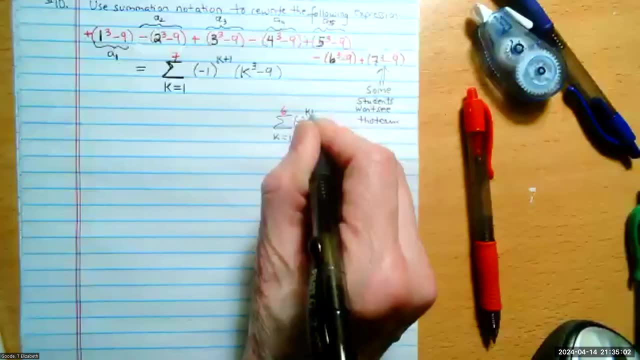 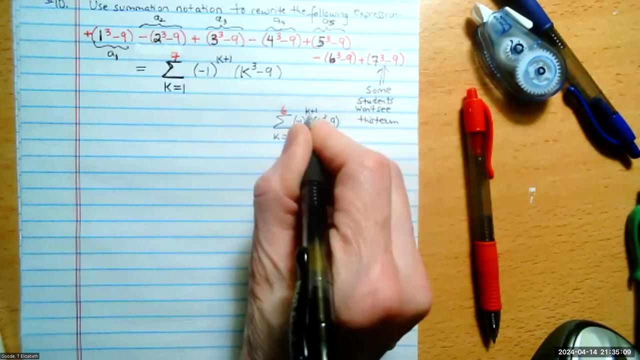 But are your signs the same way as mine are, where you have to raise negative 1 to the k plus 1? Yeah, Okay, And you could raise it to the k minus 1, but you know, I'll just say plus 1.. 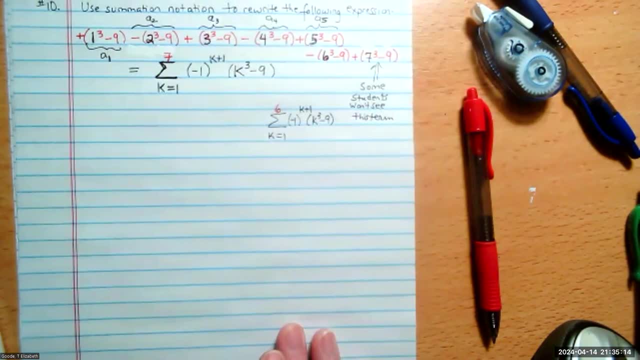 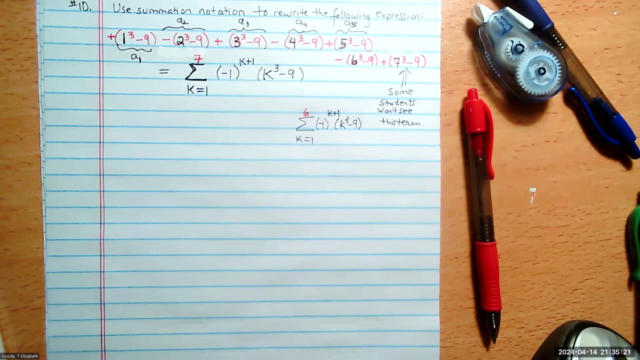 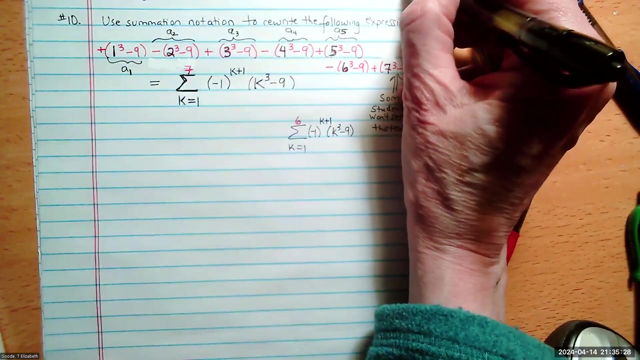 That way I never have to worry about it. Okay, Good, Did that answer your question, Uche? Oh, yes, Good. Other questions: I wonder if someone else wants to ask, but I have another one On number okay. 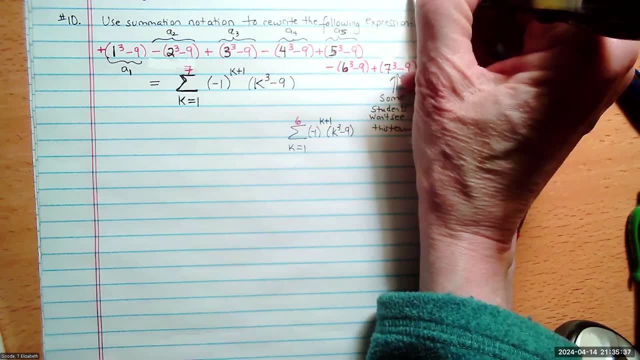 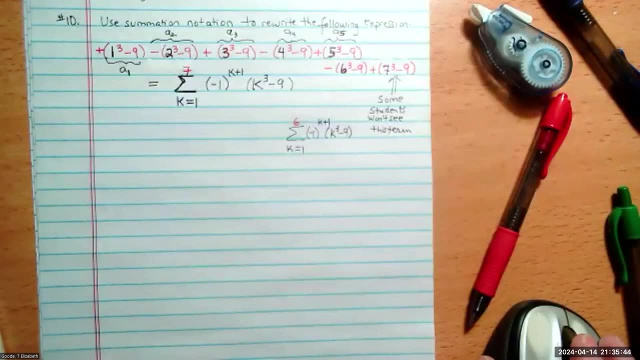 Yeah, Number 17.. Also, Webisign: Yeah, All right, I don't know. I feel like the answer I got it, but it keeps on saying it's bad. So I just really want to know if I'm making a mistake. 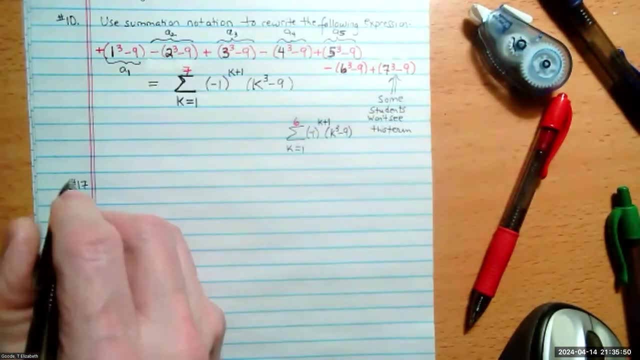 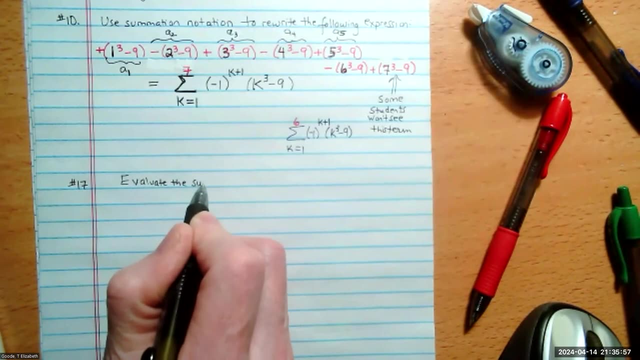 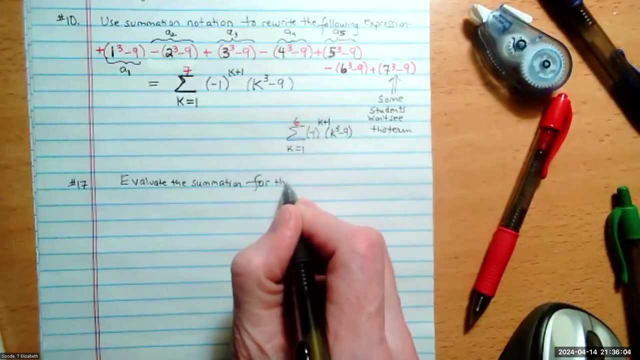 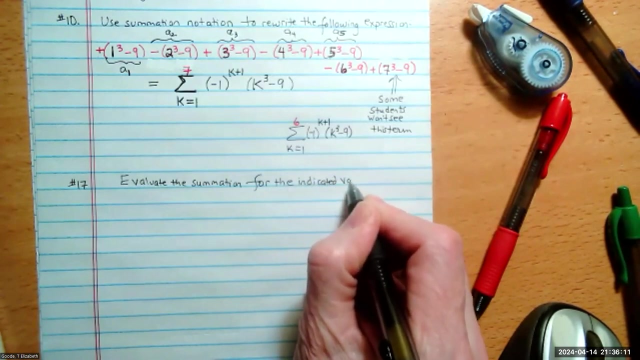 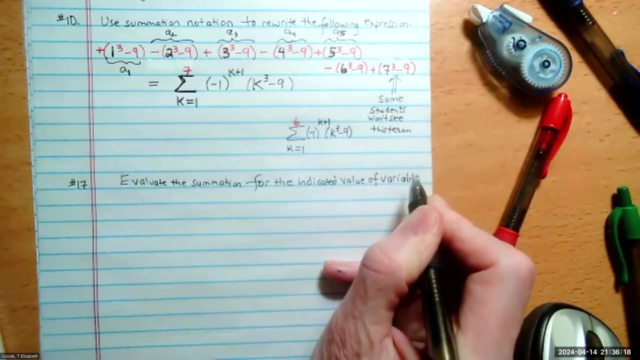 All right, Let me write down what I see. Okay, I see it says evaluate the summation For the indicated variable of for the indicated value of the variable. Okay, So I'm going to write down what I see. Now. my variable is an M. Is your variable an M? 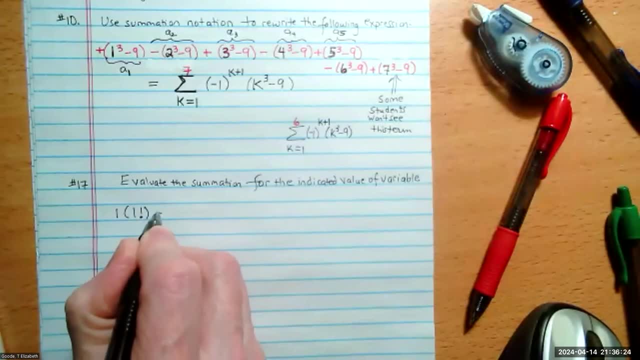 Yeah, It's an M. yeah, All right. So mine looks like this: 1 times 1: factorial. Yeah, Keep going. Plus 2, bracket 2, factorial addition, Plus 3,, you know, bracket 3, with the factorial addition and then plus 4.. 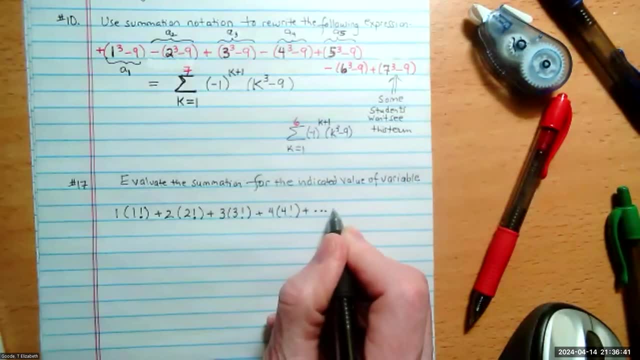 And then it goes: Dot, dot, dot, dot dot And M equals to 3. M times M factorial, Yes, And then you say, oh, it's going to go to M equals 3.. Well, this is when M is 1, right. 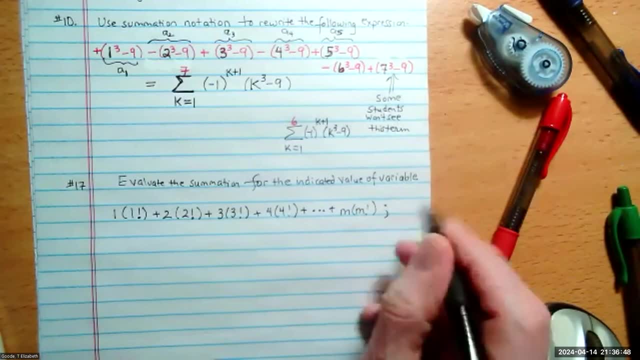 This looks like M is 2 to me. This looks like M is 3 to me. Like that would be the natural way, Right? 1, 2, 3.. Yeah, So we're just going to. it's just, it's just going to be the natural way, right? 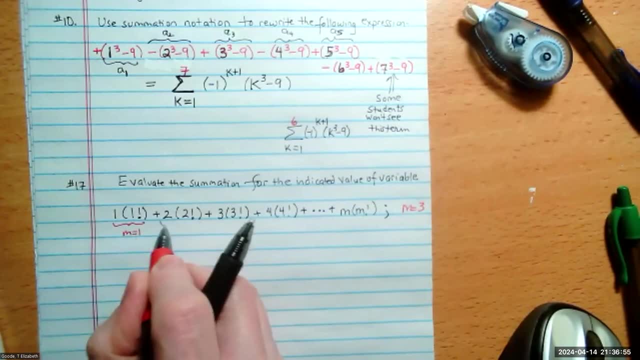 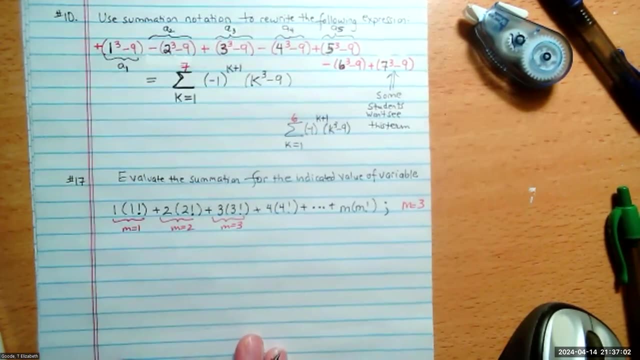 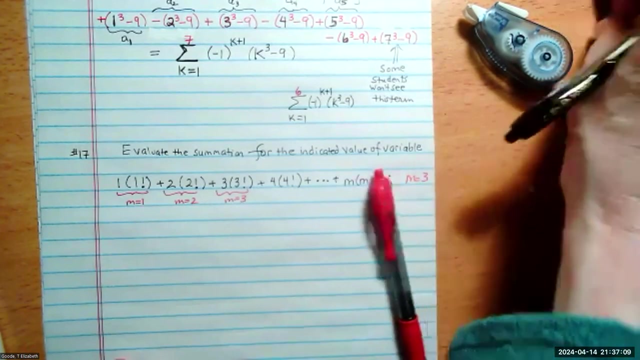 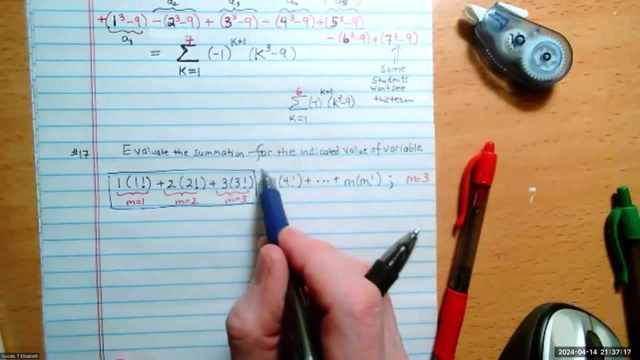 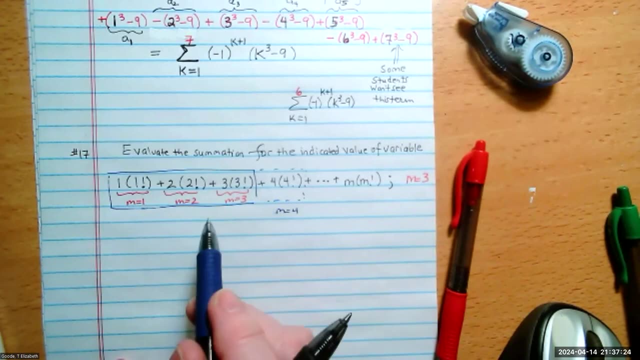 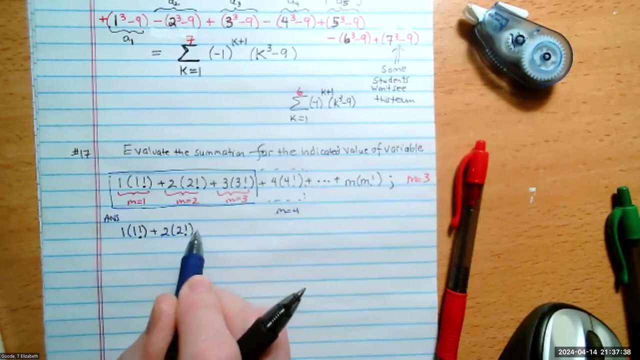 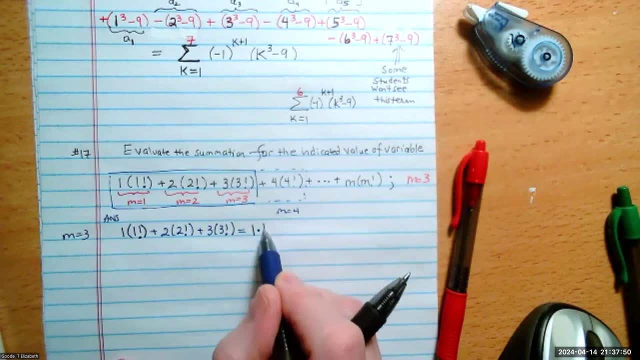 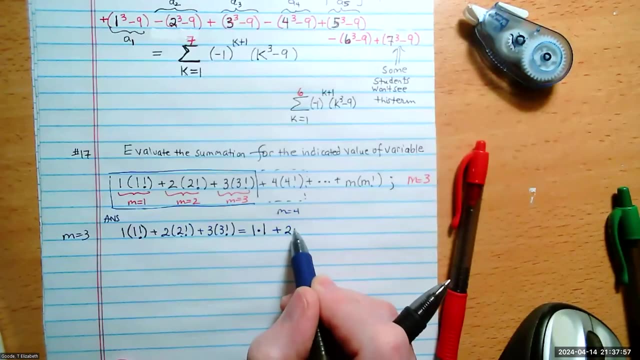 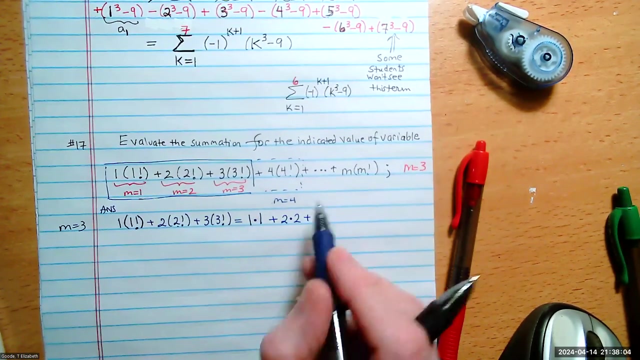 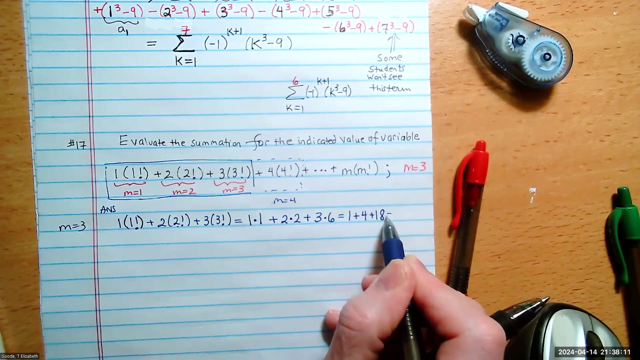 that's one, all right. so the first term is one times one. what is two factorial two? okay. so the next term is plus two times two, plus what is three factorial two, that's six. okay. so it's one plus four plus 18, i'm getting 23. 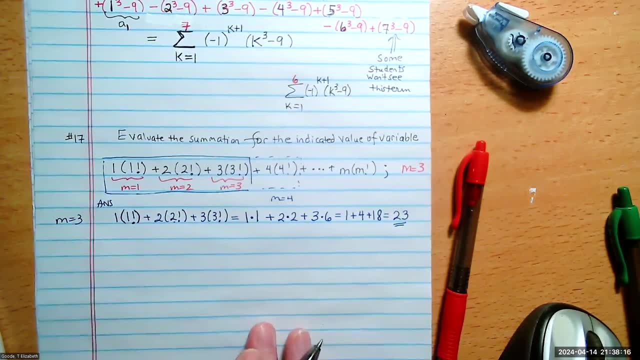 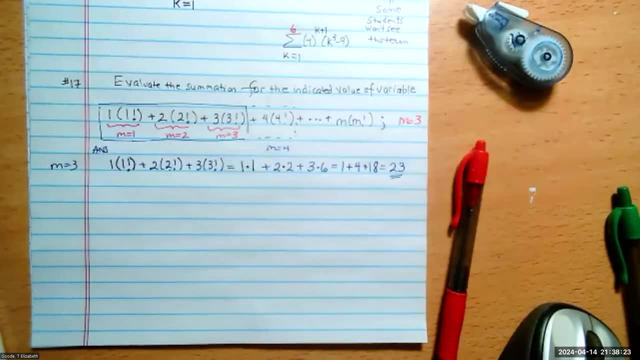 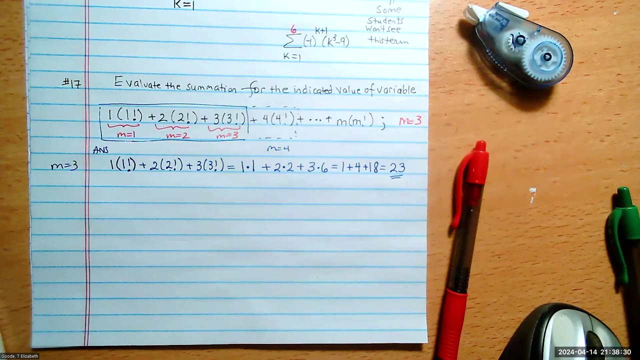 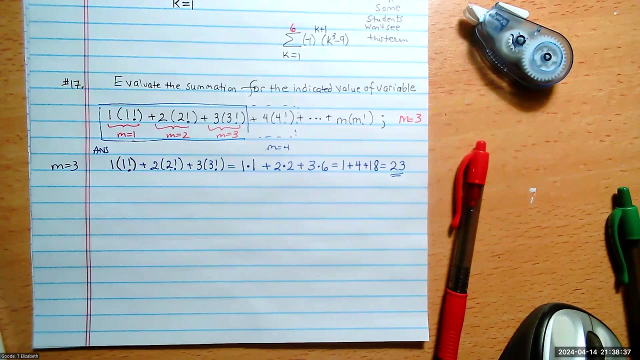 you see it, you got it. yeah, all right, sometimes it's just a silly arithmetic thing. yeah, yeah, that's it okay, cool, yeah, thank you, you're so wonderful welcome. oh, i'm so glad y'all are here tonight. um, joshua or emmanuel, do you have a problem you want to look at? 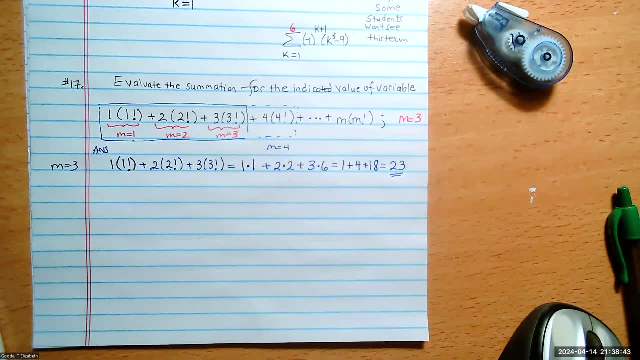 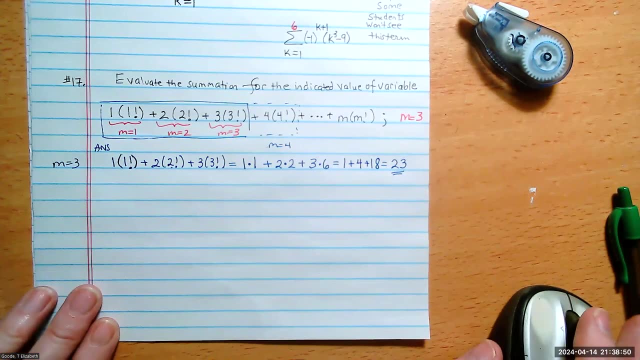 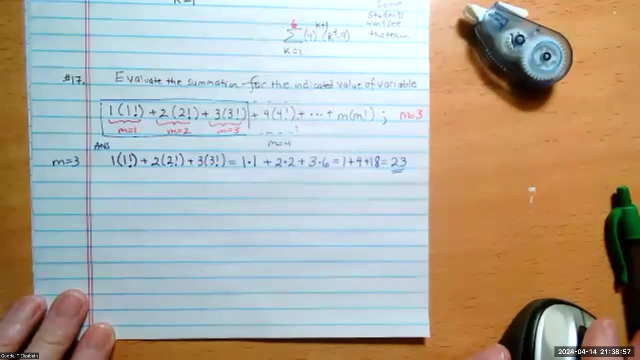 uche, you got another. oh, oh yeah, number 18. let's go, let's, let's do it. you're prepared? yeah, i wrote them all down. oh, that's awesome. yeah, so they're number 18, number 18 still on website. i love it. i love how prepared you are. 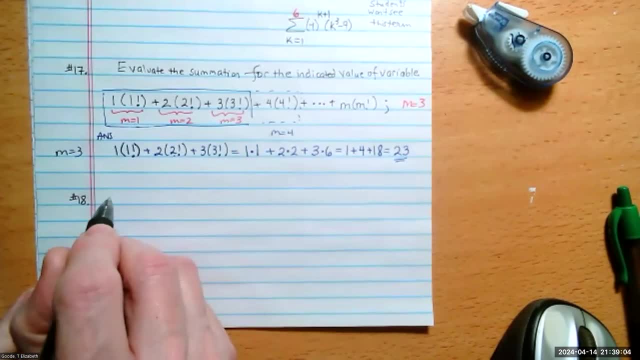 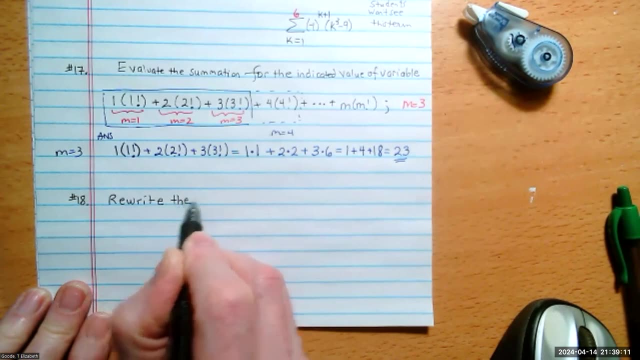 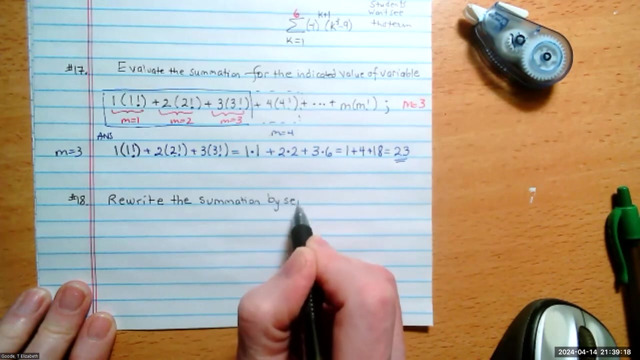 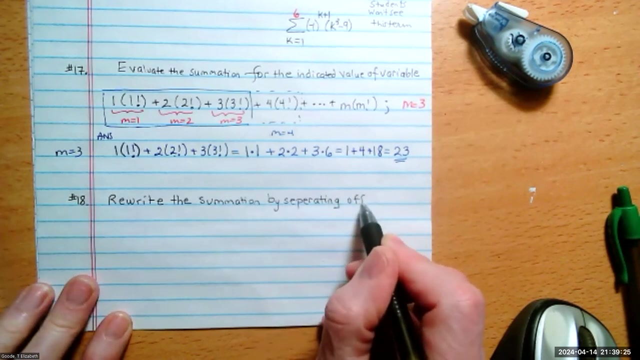 but all right, here we go now again. sometimes they look different, so let's just see what mine says. mine says: rewrite the sum- oh, this is a good one. the summation by separating off. and this is the first thing we're going to practice on in day 20 when we do lecture: separating off the final term. 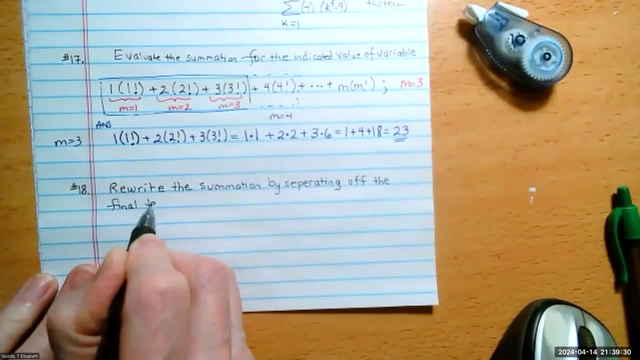 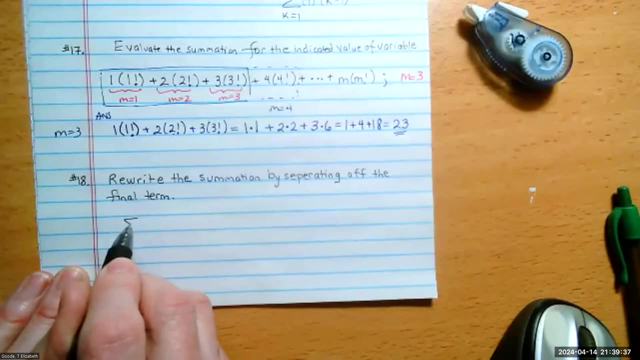 there's actually a reason why we need to learn to do this. so i'm yeah because i'm i yeah. i tried to find it in the note. i didn't think so. no, no, we haven't done this yet. this is think of on your own, all right. so does your say? the sum from k equals one to m plus one. 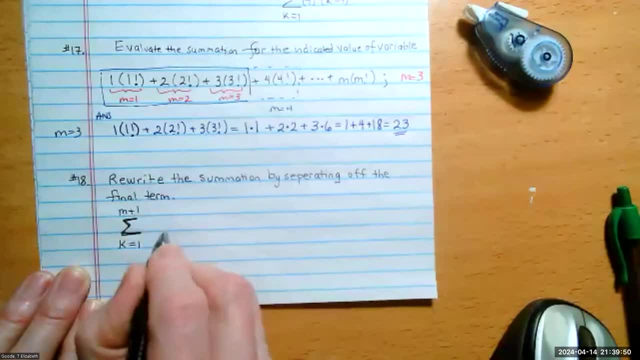 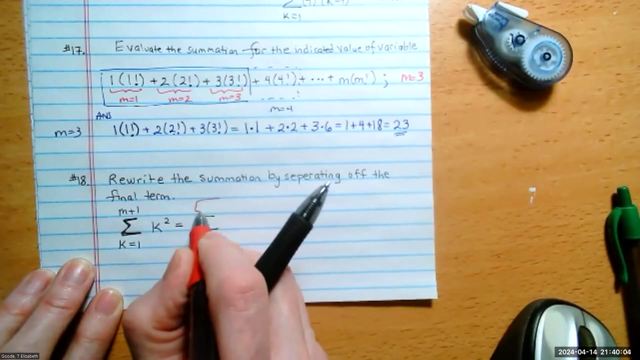 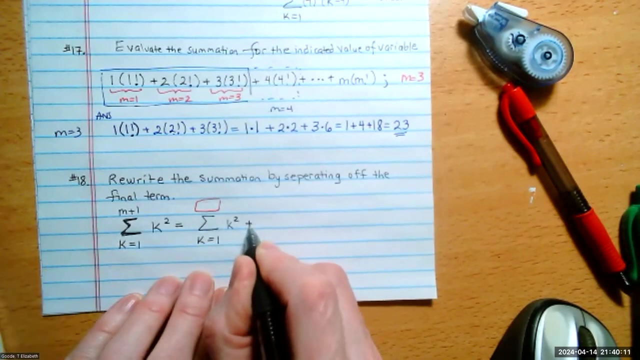 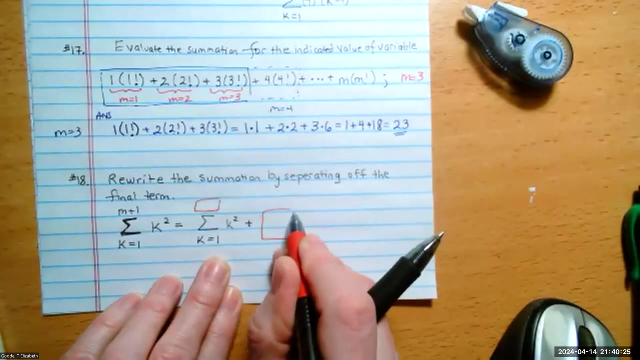 yes, m plus one, and then the term is k squared and it's supposed to equal. okay, the sum from k equals one to something of k squared plus m plus one square, yeah, plus here here. see, here you're supposed to put in the summation symbol and they: 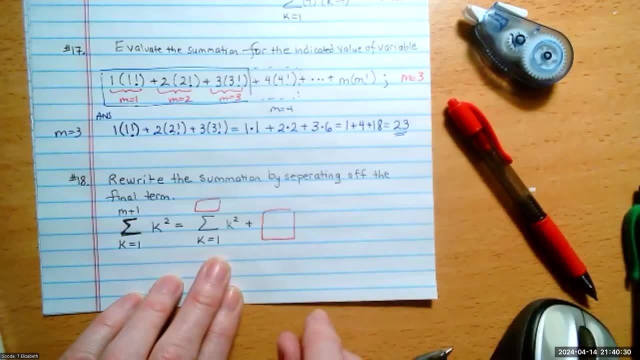 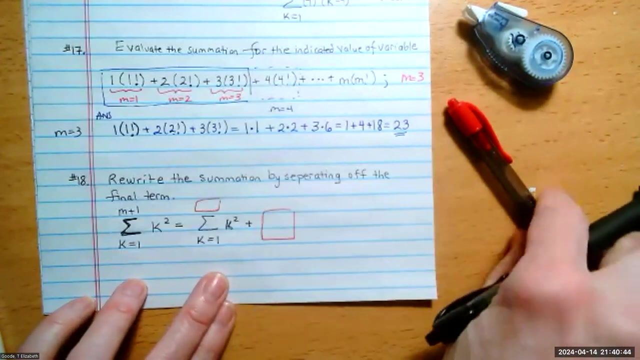 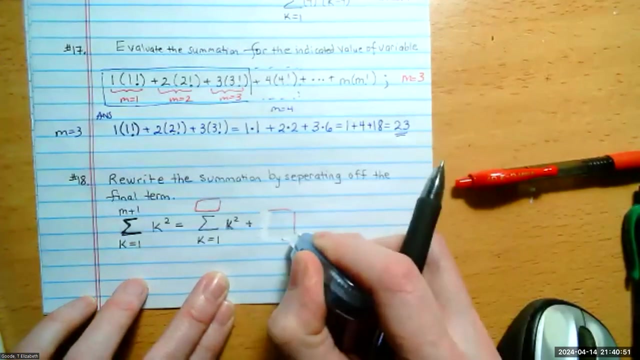 oh, not the summit, but but the last term. yeah, because the term is: you put the indexing value in for k, all right. so how did you know that this is m plus one squared? well, i'll show you, okay, what we're really going to do, breaking off the last term in the summation. well, let's think: 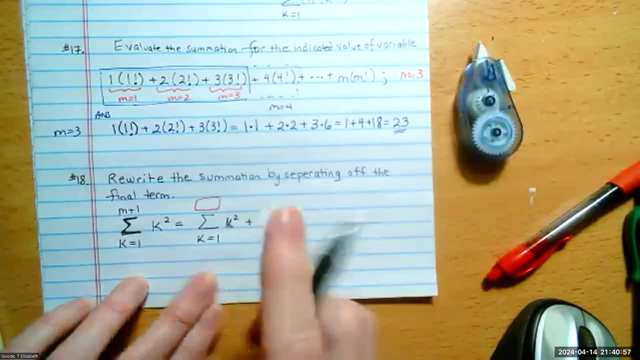 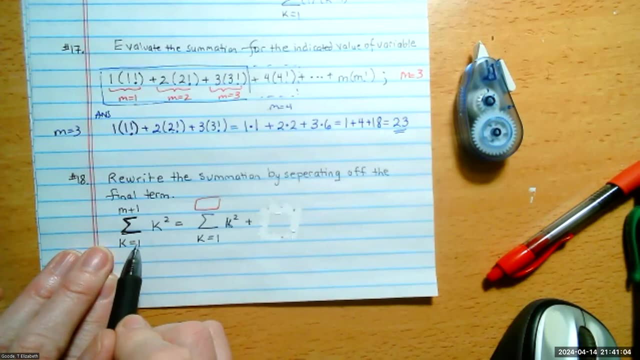 about these terms. okay, look, this starts at: k equals one, then the next k value is two, and the next k value would be three, and you keep going. what is the k value right before we get to the m plus one upper bound for k? what's the integer right before that? 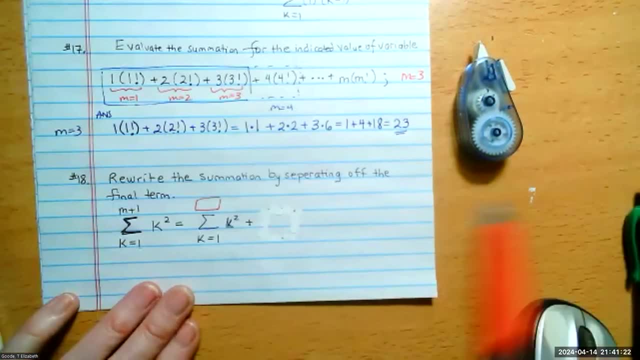 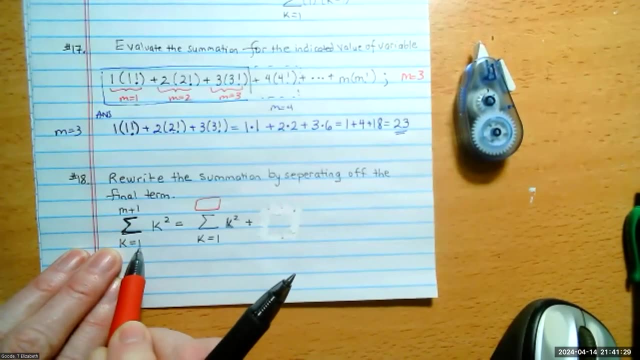 actually the question again. all right, let's think about these indexing values. we're starting with the lower bound. k equals one, right? yeah? then the next k value would be two, then the next k value is three. you with me? all right, so we're keeping on going. what is the k? 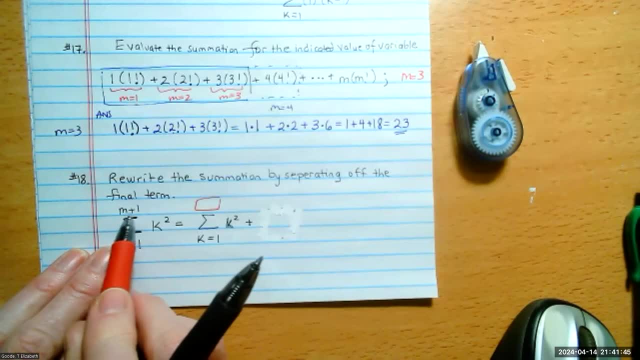 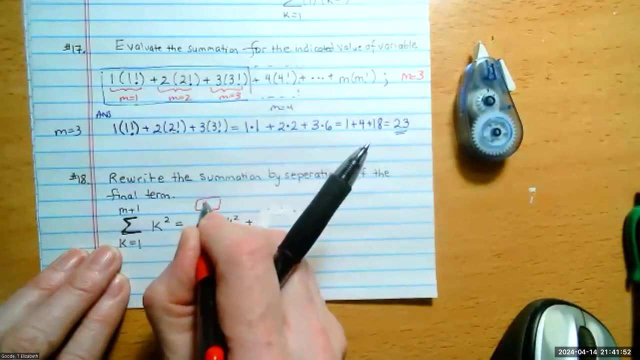 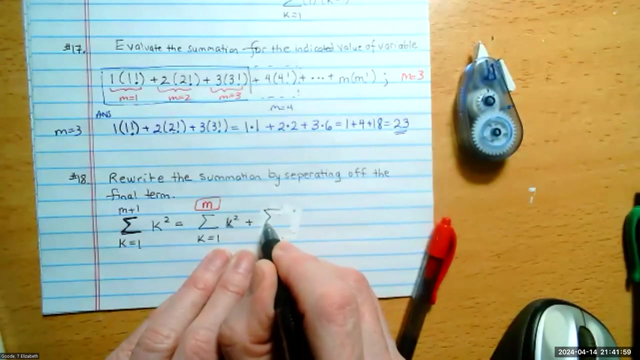 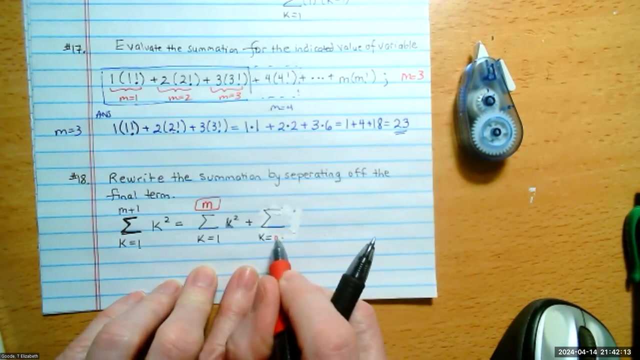 value right before we get to: k equals m plus one. that's k plus m, yeah, it's. it's. k is equal to m. yeah, and then what's really going on is we can write this as the sum from k equals one to m of k squared plus, and then we pick up where one bigger than this, where k starts at m plus one. 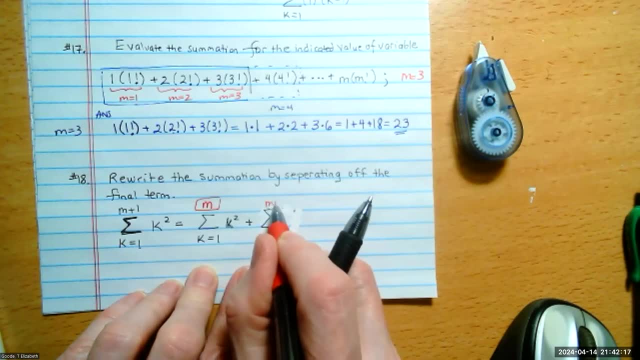 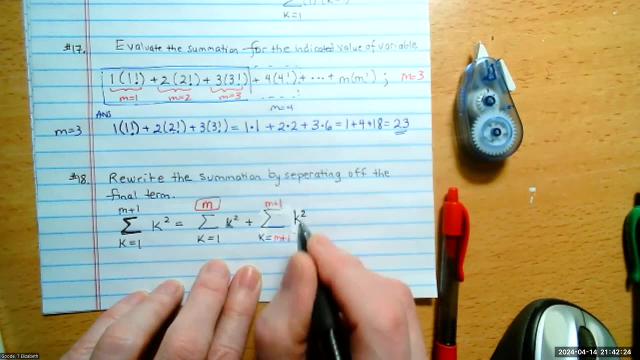 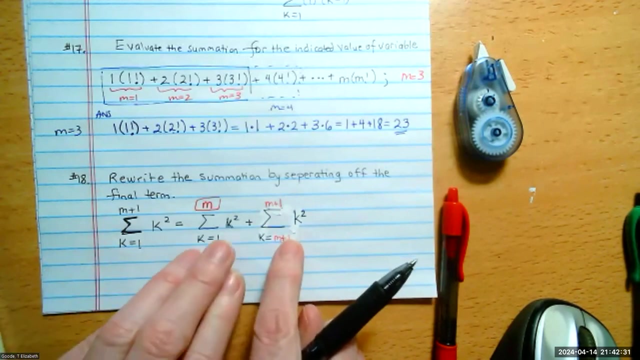 and ends at m plus one. you actually had to do some reading. you had to go to the book and read a little bit, all right. so what's happened here is we've just broken off the last term, the m plus first term. the k squared is still the same for both of these. but you see, see, think about it. 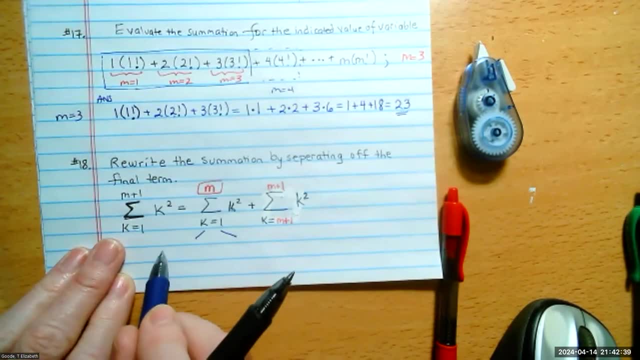 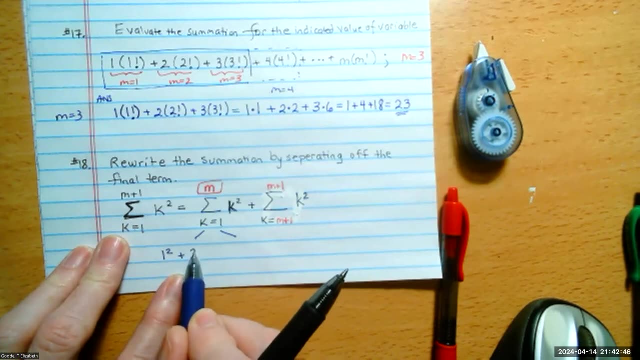 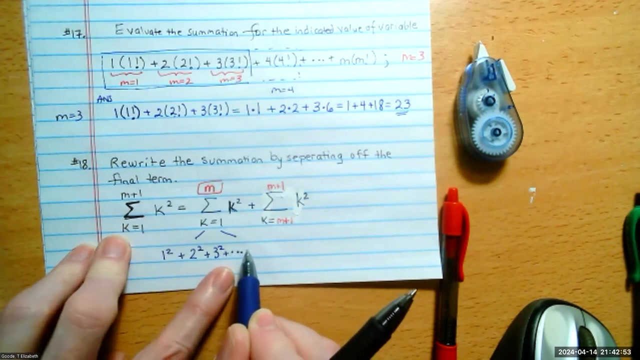 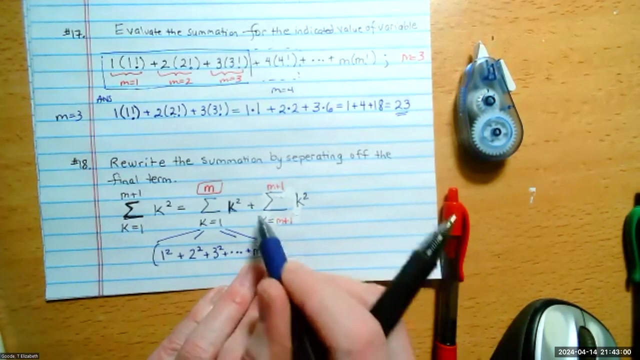 what does this really mean? this means one squared plus- because k just gets plugged in here for k, right plus. then k is two, two squared plus three squared plus. keep on going up to m squared. that's what this means. and then plus. oh well, this says k starts at m plus one. 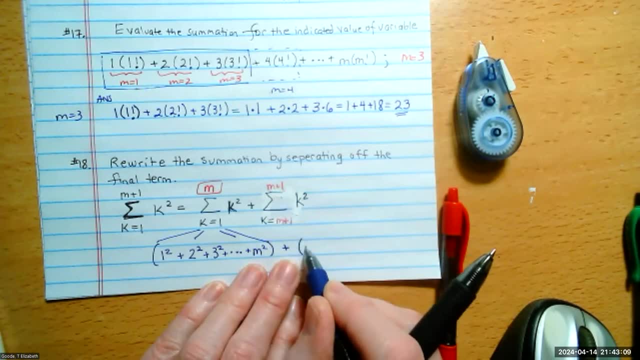 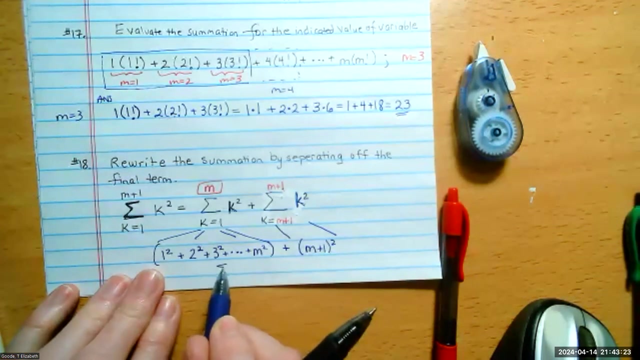 and ends at m plus one. so this term is just m plus one squared. see, that's all this one is. it's just a single term where k is m plus one. so that's what they're trying to show you. it's: the sum from i equals one to m. 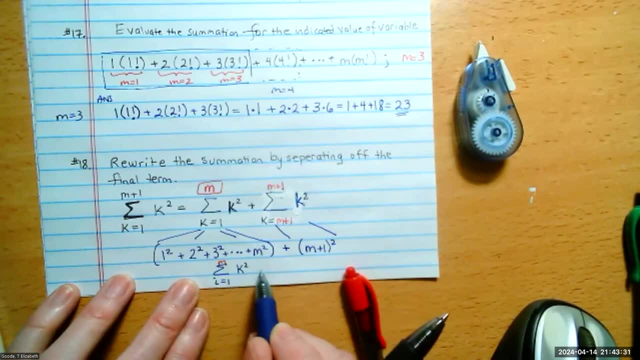 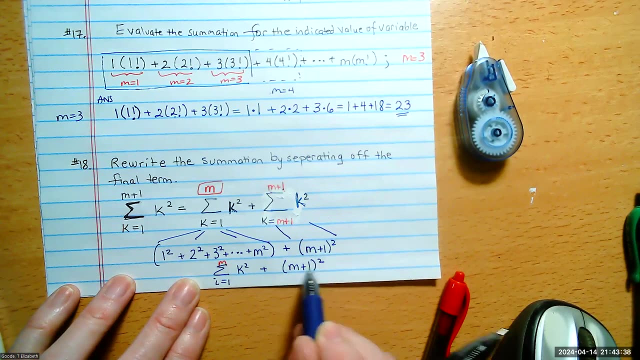 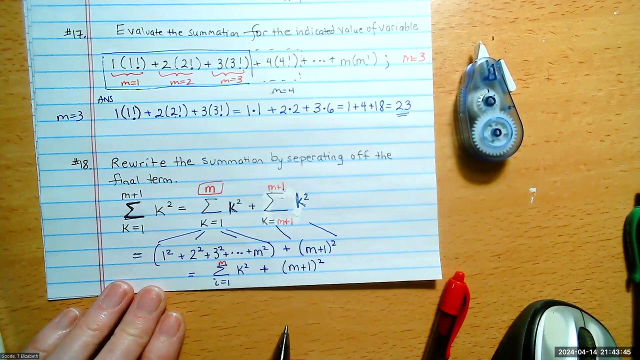 of k squared plus, and then this term is just a single broken off last term, which is the m plus first term. yeah, and that's that's what's really going on here. that's the same thing for the 19 and for the 20. yeah, yeah, for the 22. so i don't know if you want to. 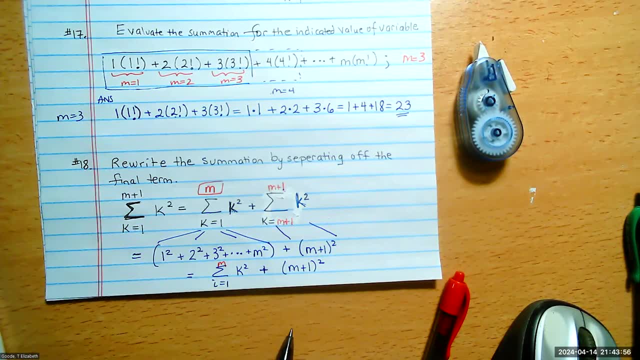 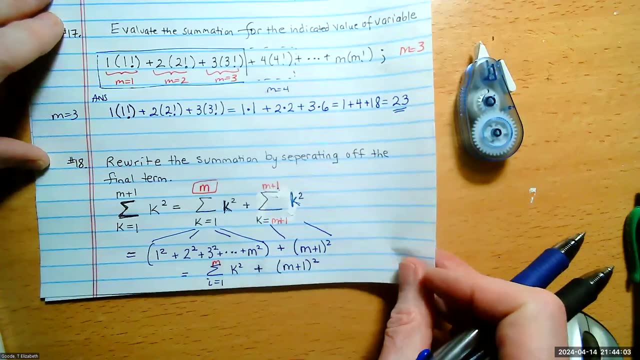 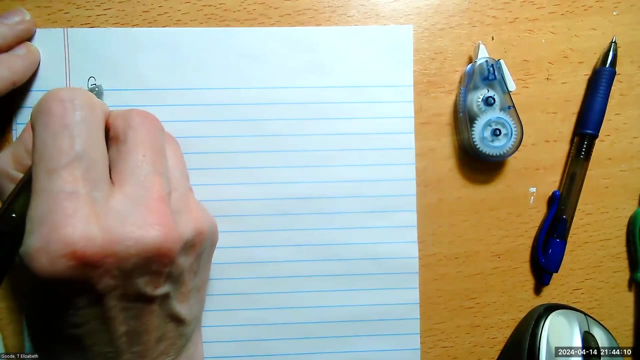 touch them now, or you want to do it when we come to class, but if we can do all of them now, it will still be good, so it just well. why don't we? let's go ahead and look at number 19, okay, and we can look at the general idea. let me give you the general idea, the general idea of breaking off. 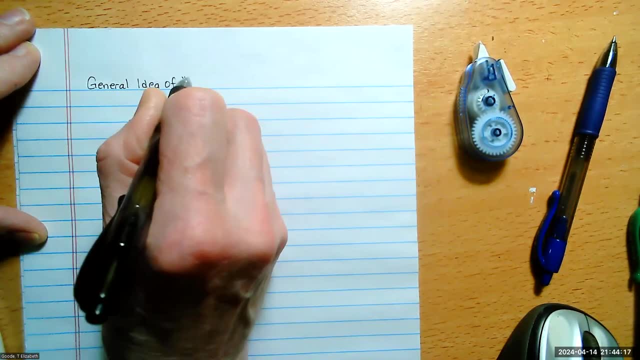 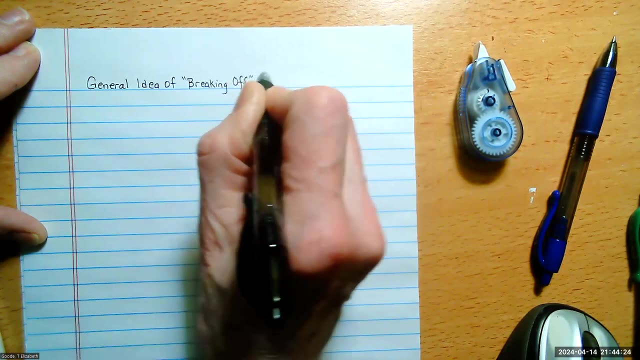 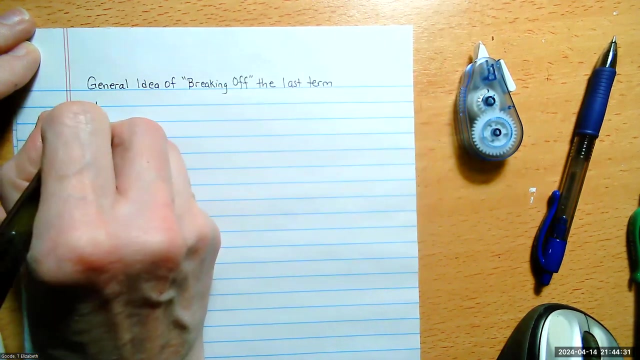 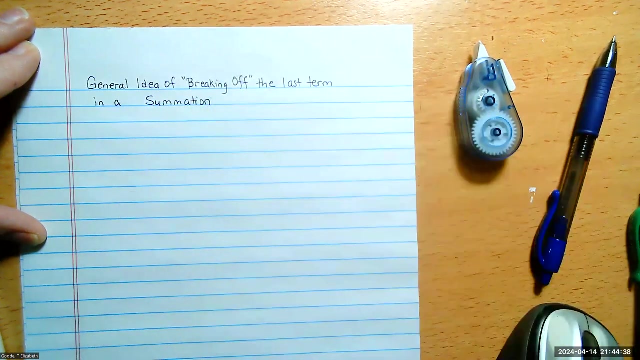 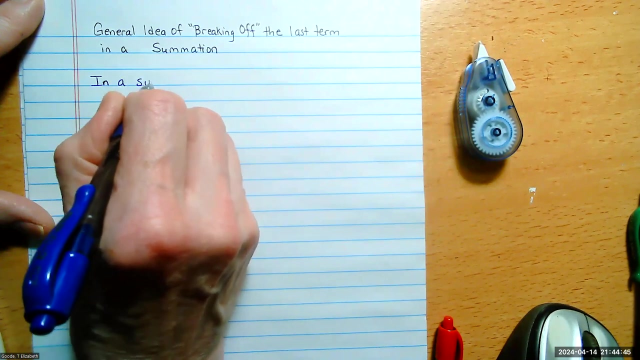 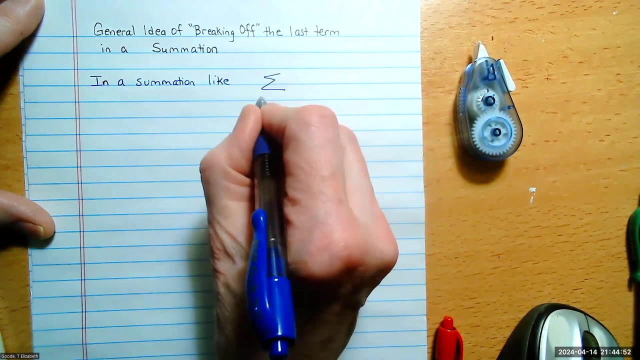 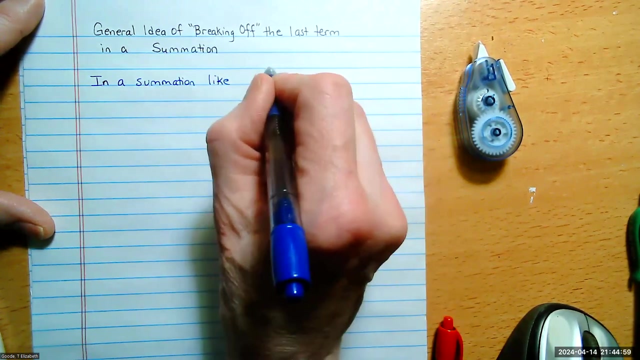 the last term in a summation, in a summation. so in a summation like the sum from k, k equals. I don't care where we start. let's say 1 up to some value, m of some term. You know it can be different things. 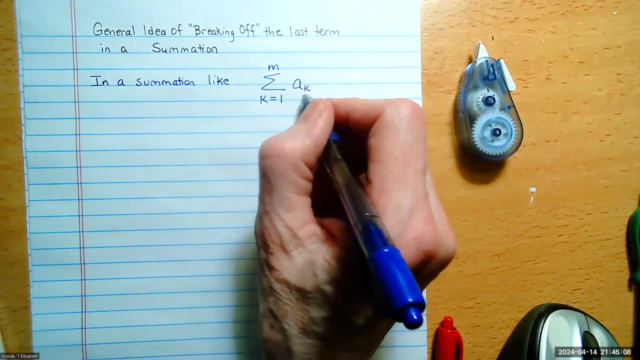 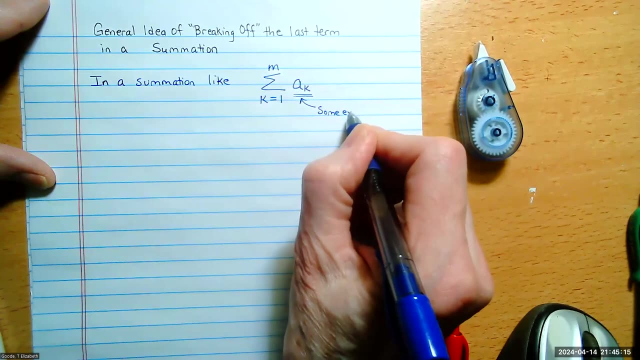 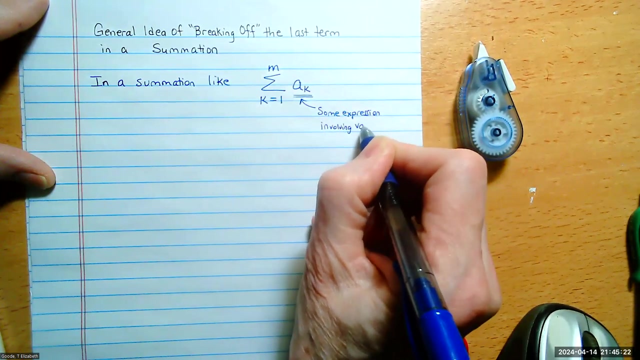 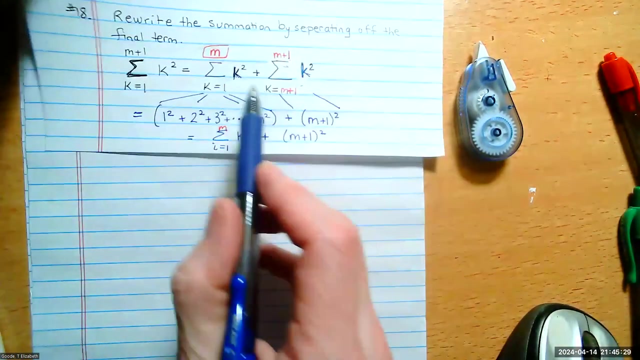 It could be k squared, It could be k plus 1 times k plus 2.. I mean, the point is, this is just you know, some expression involving k And, like I said, we just looked at an expression where, you know, the term was actually just k squared. 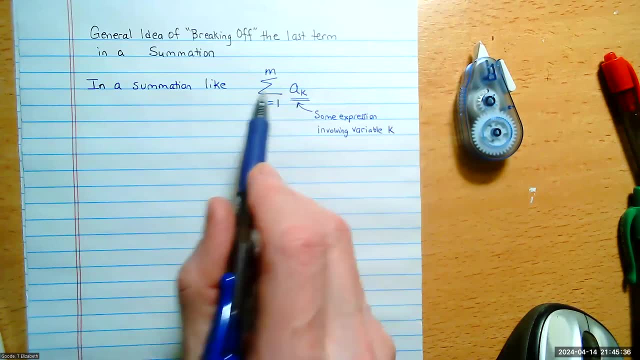 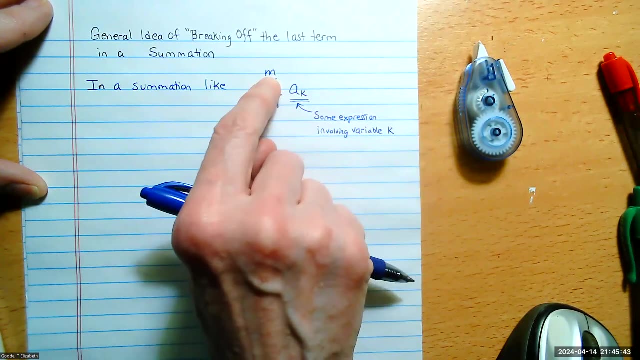 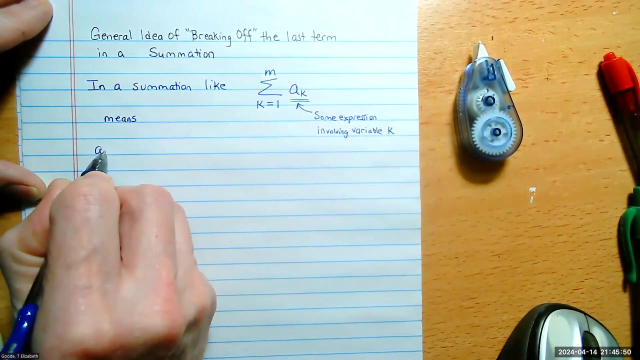 That was the a sub k, But in general, this idea: if you have a summation like this, where you're starting at a lower bound, like 1, and you're going up to an upper bound, like m, this really means a sub 1,. 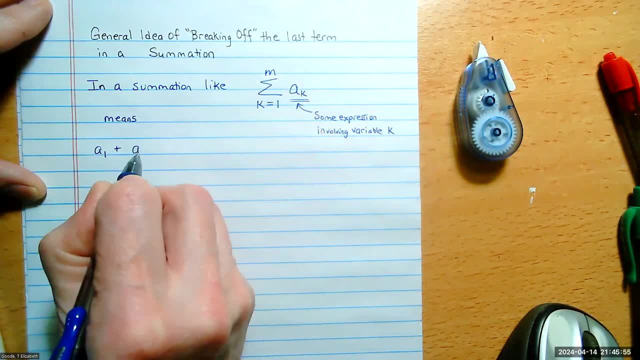 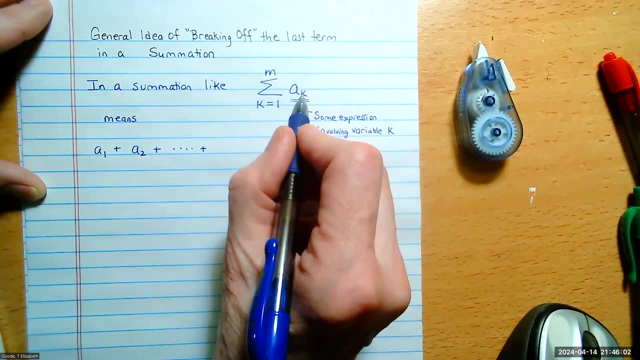 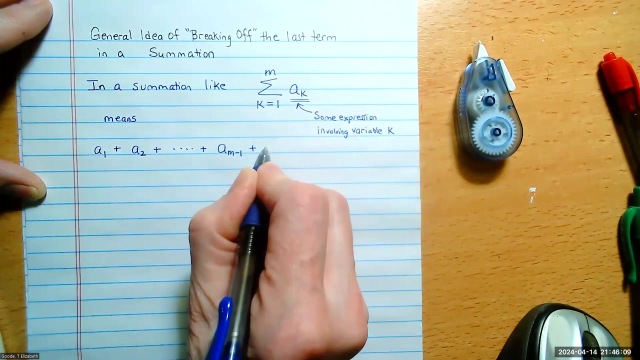 because when k is 1, you just put in the 1. 1, wherever it goes, plus a sub 2,. plus keep on going plus. well, the last term is when k is m, But the term right before that is when k is m minus 1.. 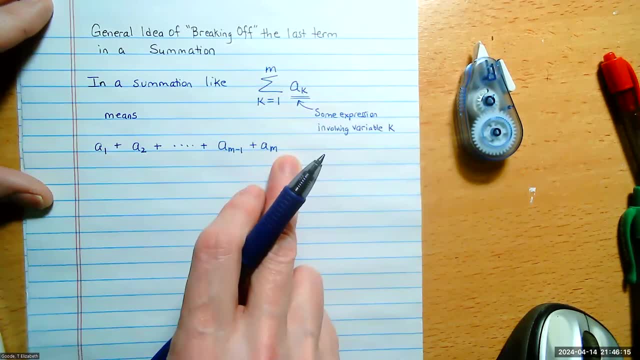 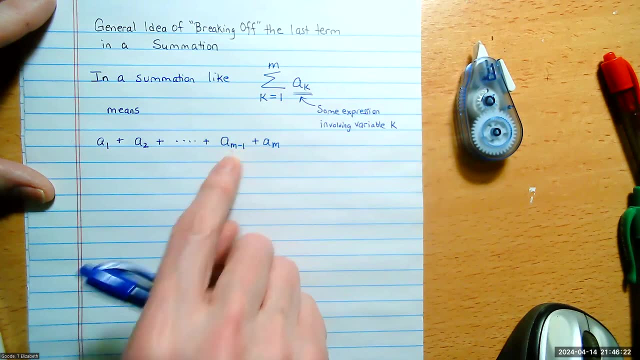 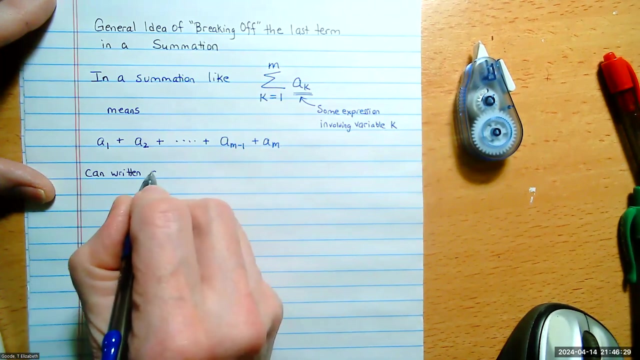 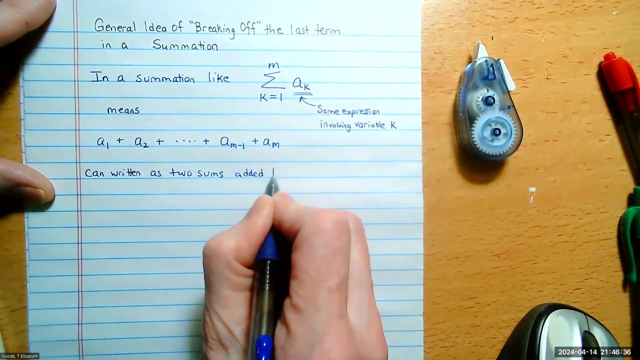 Okay, See what I mean. You with me, You understand why I said this here. Yes, All right, So this, This can be written as two sums added together, Because we can group them. We can group these together and then have this one sort of broken off. 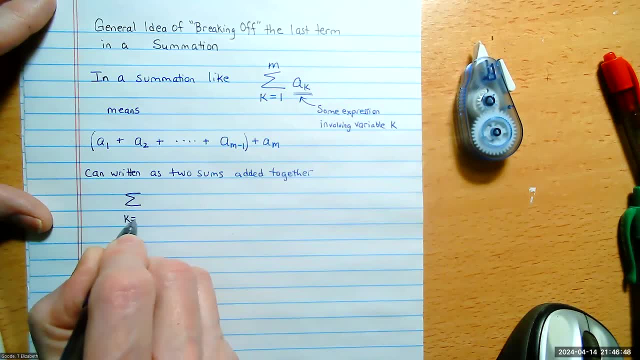 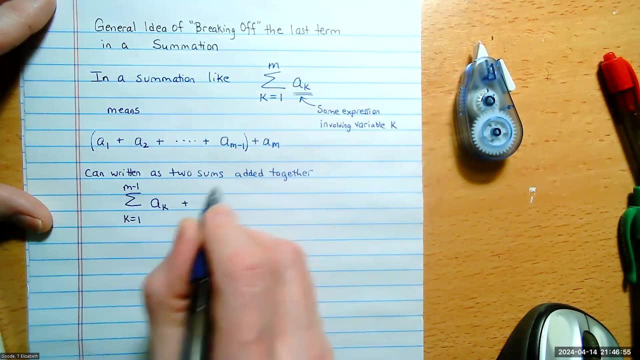 It can be the sum from k equals 1 up to m minus 1 of whatever this thing is. So this is a sub k plus and then this broken off term. we could write it like this: K starts at m and ends at m. 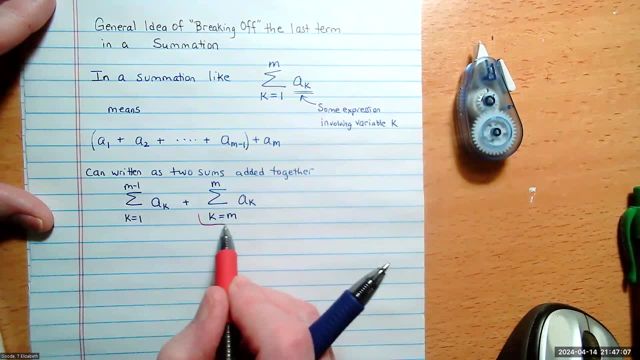 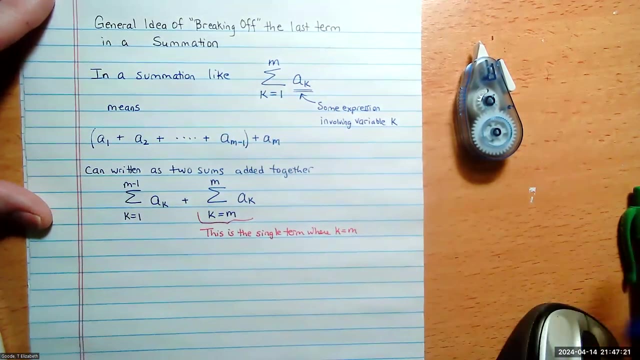 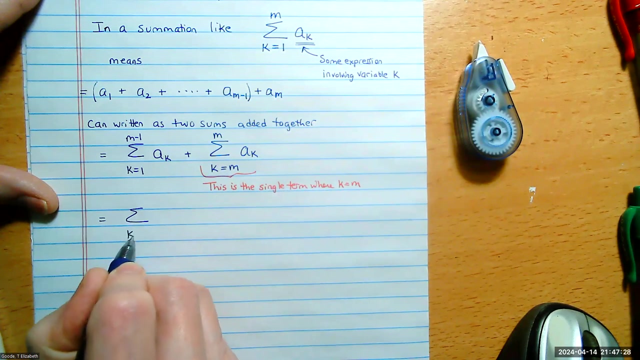 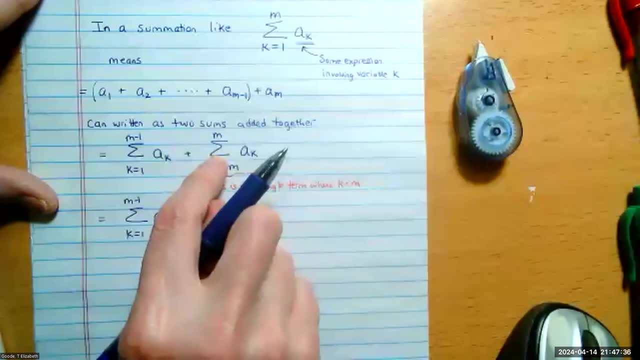 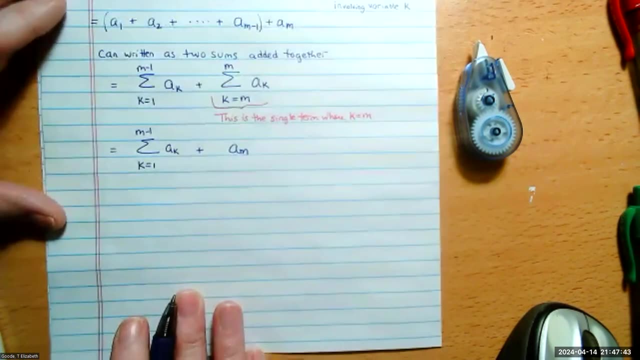 And since this is just a single term when k is m, we don't even need a summation symbol. We could just write this as the term a sub m. All right, So now let's look at number 19.. All right, 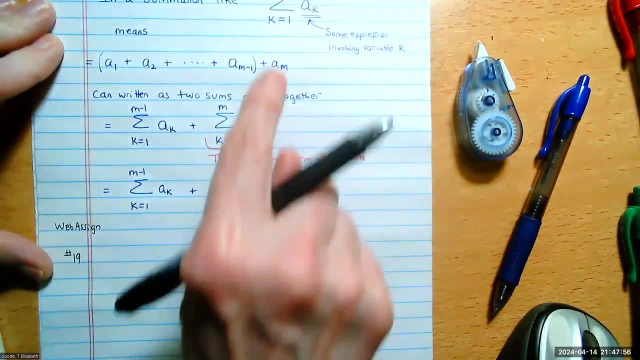 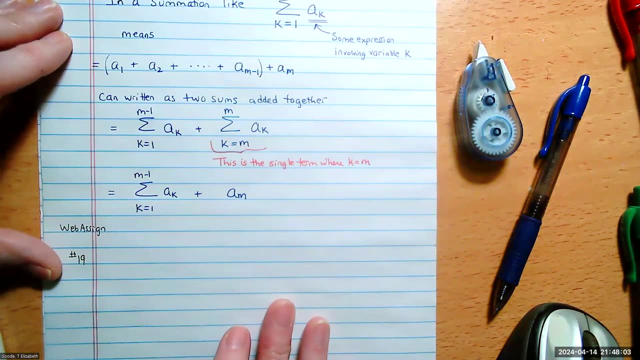 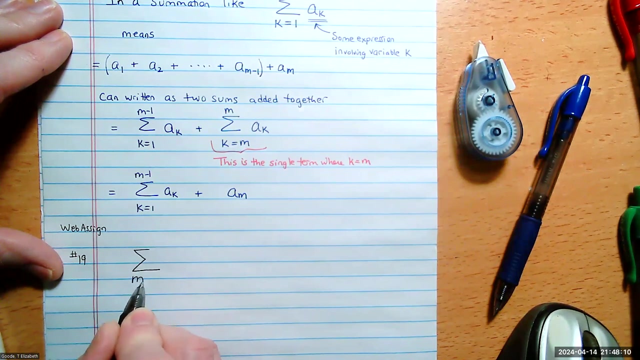 And this top number can look different. It can be an m or, you know, it can be an n, or it can be an m plus 1, or The point is there's always one right before it. So here in number 19,. we have the sum from m- okay, equals 1 up to n plus 1.. 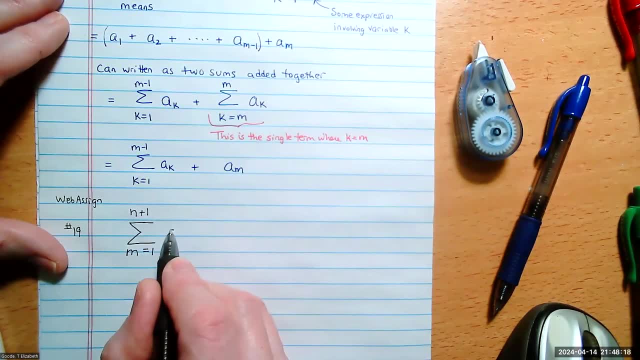 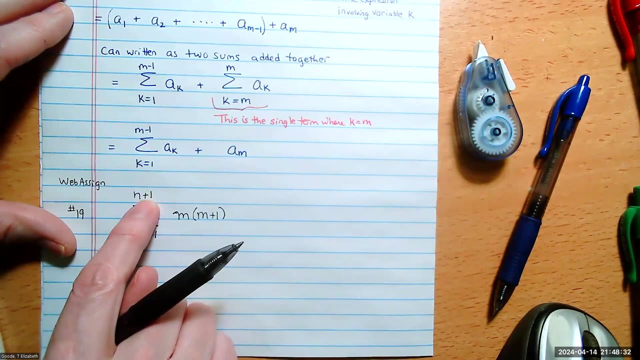 And the term a sub m looks like m times m plus 1.. So we're supposed to separate off the final term. So we need to understand this starts with m equals 1 and it ends with m equals to n plus 1.. But what's the term right before n plus 1?? 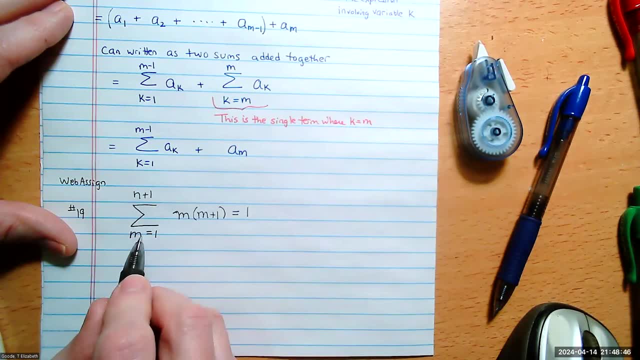 I mean, let's just think about it, It's 1.. All right, When m is 1, we plug in a 1 here and we plug in a 1 here, It's 1 times 1 plus 1.. 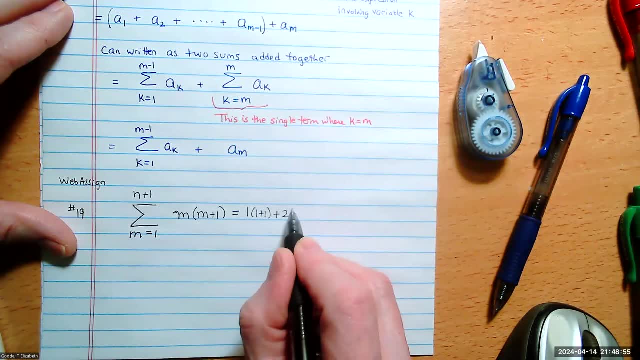 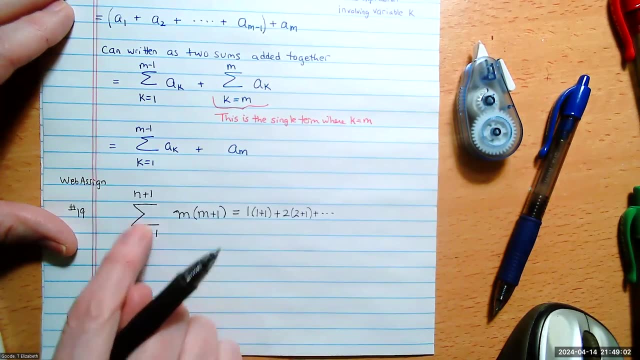 Plus, Then m is 2.. 2 times 2 plus 1 plus dot, dot, dot. right, See what I'm doing. And now the last term- I'm going to put it way over here- is when m is equal to n plus 1.. 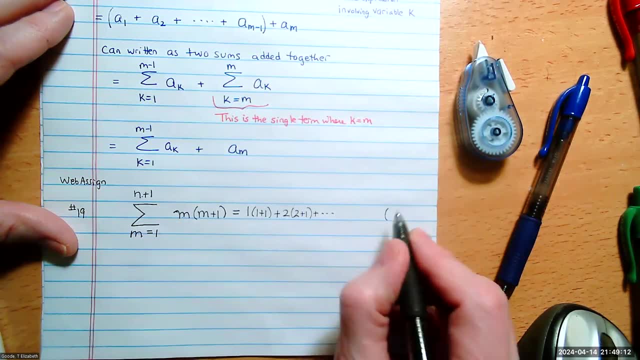 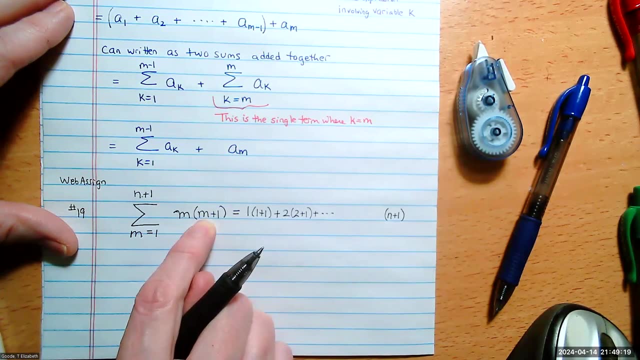 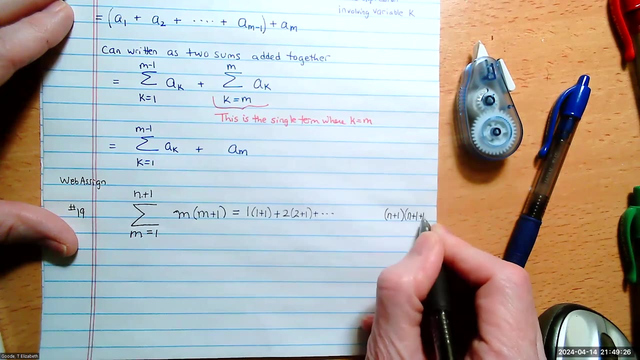 So the very last term is when we plug in an n plus 1 for m there, And then we plug in an n plus 1 for m, but it's n plus 1.. Plus 1.. Okay, so that'd be the last term. 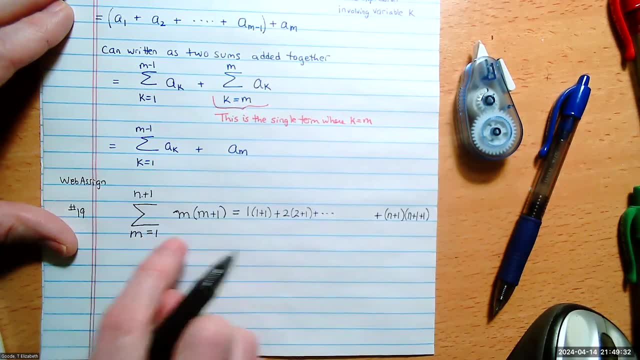 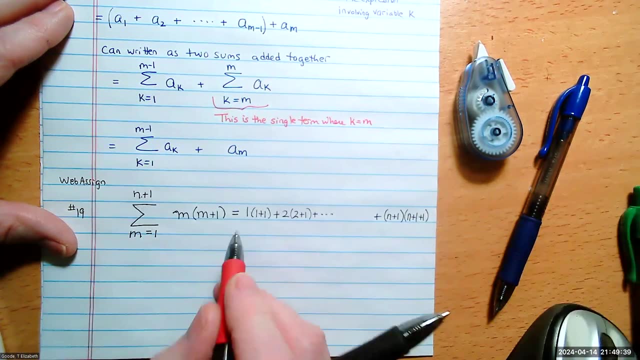 What's the term right before, What's the value of m right before? when m is n plus 1?? See, this is when m is equal to 1.. This is when m is equal to 2.. This one is the last one. 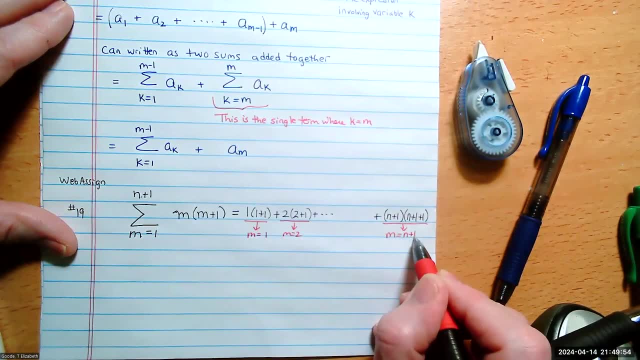 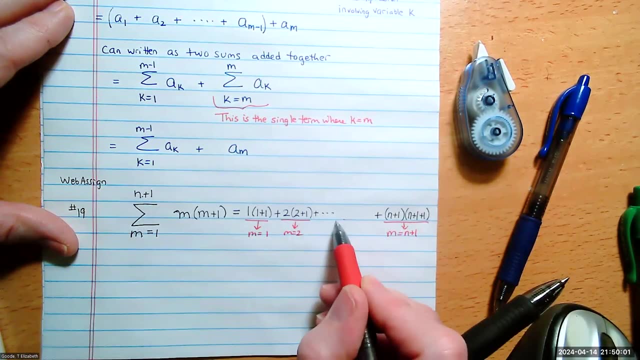 When m Is equal to n plus 1.. What's the one right before it? What would m be right before m hits n plus 1?? Probably m minus. No, it wouldn't be n minus 1.. What's 1 less than n plus 1?? 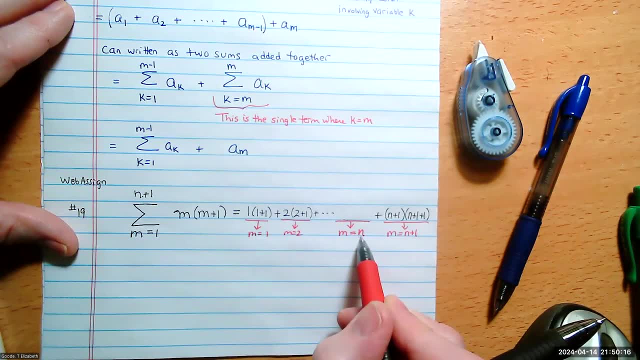 n minus 1? How about n? We'd hit n first. The one before that would be n minus 1, right, Yeah, No, that's okay. I mean, this is the first one. This is the first time you've seen this. 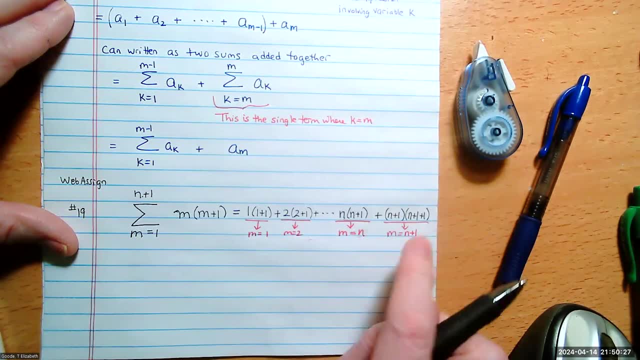 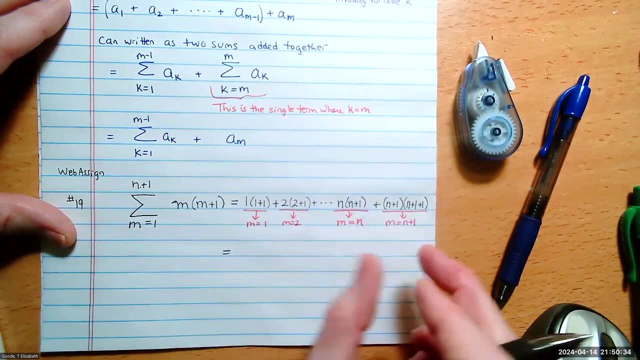 n times n plus 1.. Okay, so that would be the one right before this last one, Do you agree? Yes, All right, So if we want to write, We want to break this term off. okay, So we have to write this as a sum. 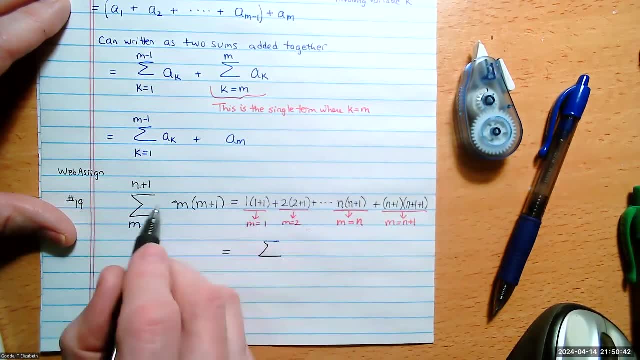 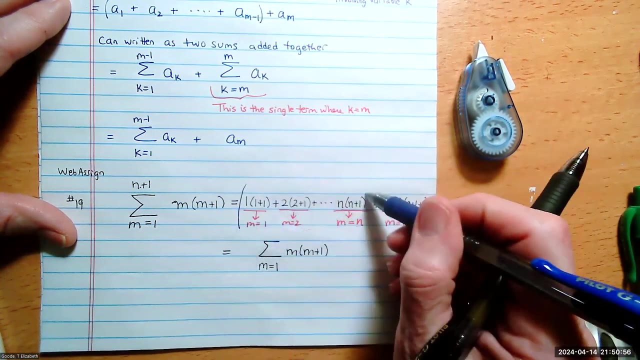 Oh well, okay, So it's the sum and the a sub. m looks like m times m plus 1.. We know that goes there All right, So m still starts at 1.. But when we're going just to here we're trying to collect that as a sum. 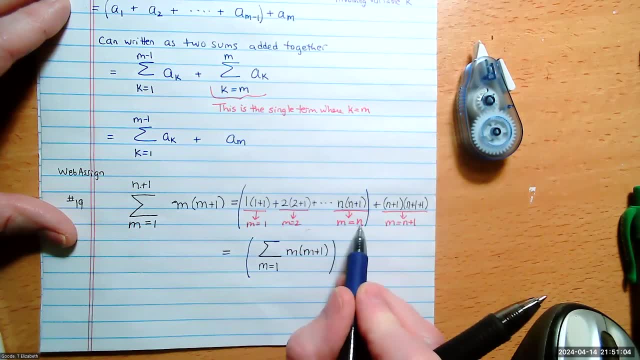 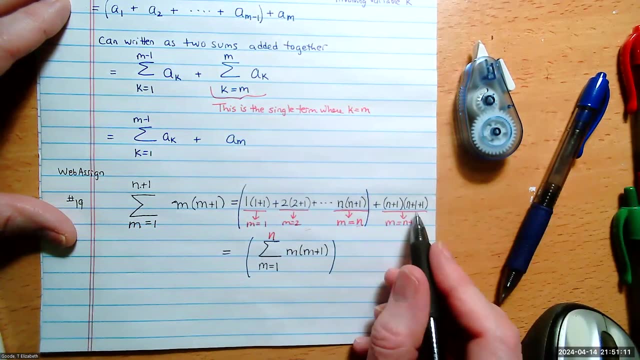 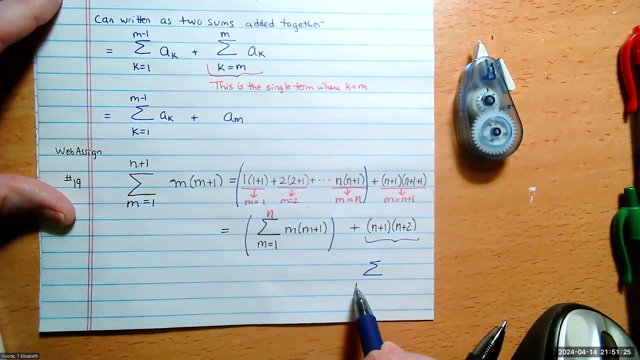 What's the top value for m? Oh it's n. And then this term is n plus 1 times. Oh well, n plus 1 plus 1 is just n plus 2.. The thing to understand is we could write that, as the sum from m equals n plus 1 to n plus 1 of m times n plus 1.. 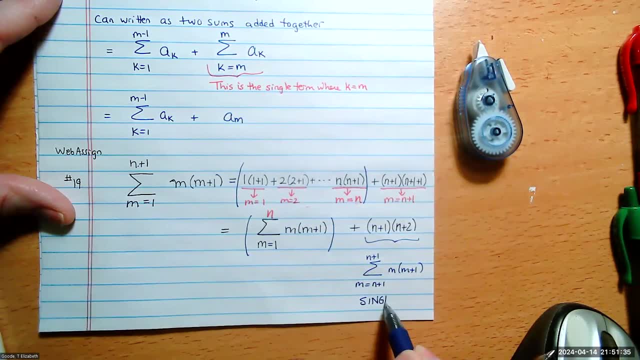 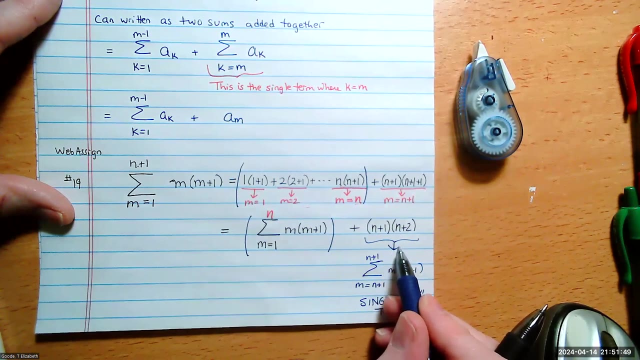 Because it's just a single term, But we don't, you know, we don't usually write it, you know, as a sum, but we can. Usually, if it's just a single term, we can write it as a sum. 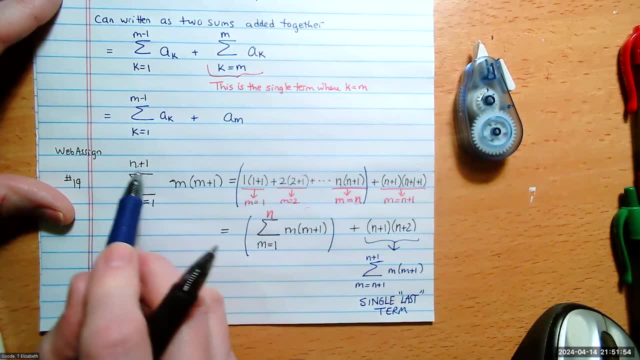 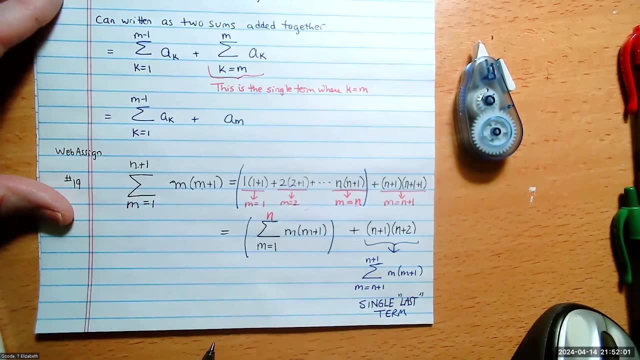 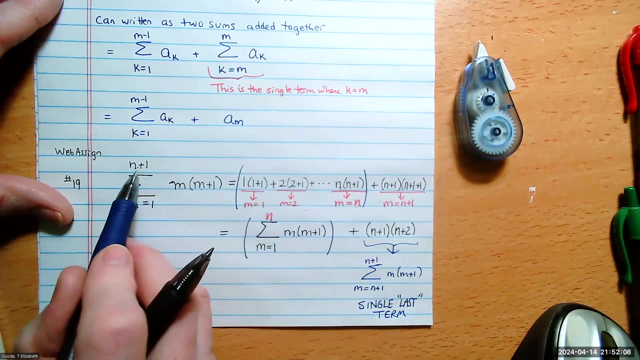 But if it's just a single term, we just evaluate it and plug in the value n plus 1 for m here and here. Does that make sense? How did you get the n on top again? Yeah, okay, Because what's the integer right before the integer n plus 1?? 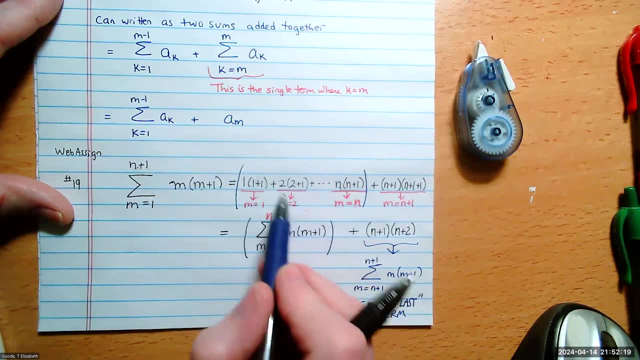 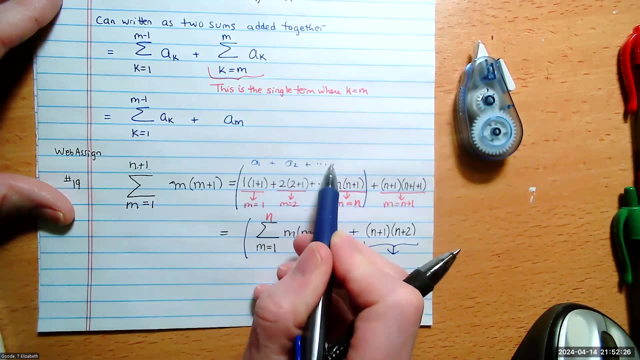 It's the integer n. See what I mean. So this is like a 1.. 1 plus a 2 plus dot dot, dot plus. See this term right here. this last term is a sub n plus 1.. 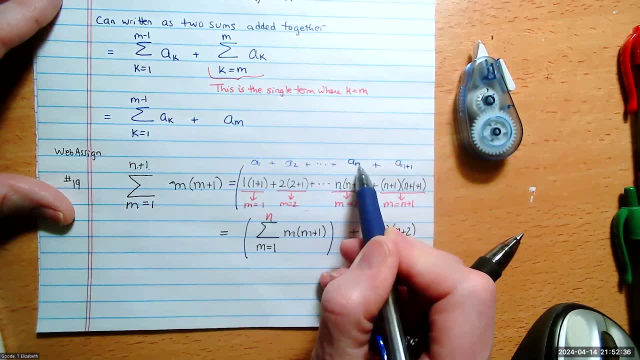 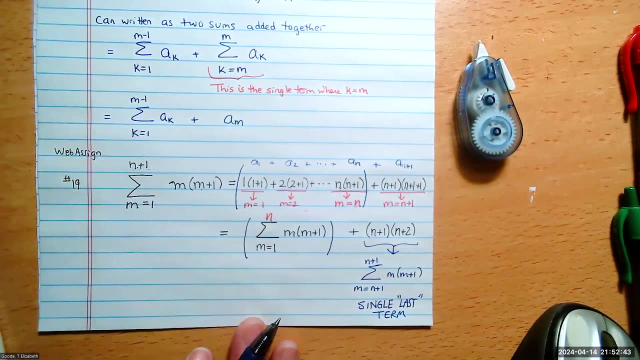 But the term right before that is a sub n, When m is actually equal to n. I know it's confusing, It is. It really is. I get that it's confusing. Wait, Did I answer your question, though? I mean, I'll still go back and look at it. 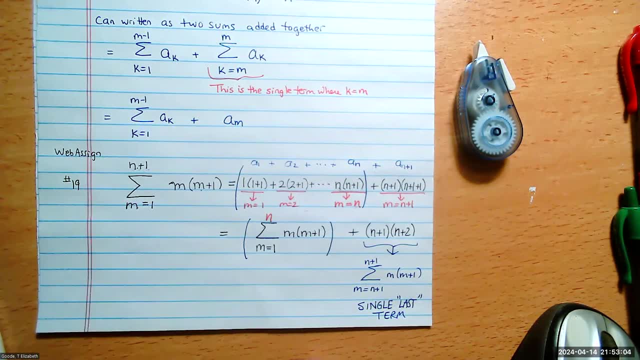 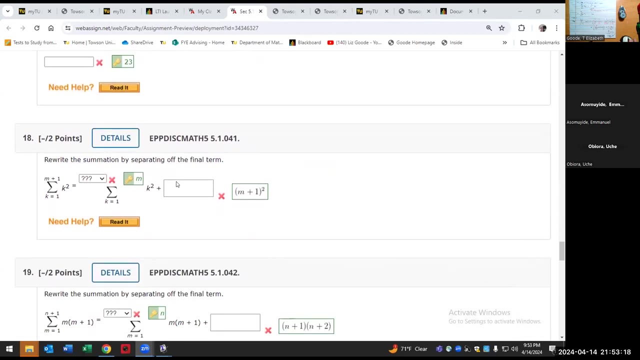 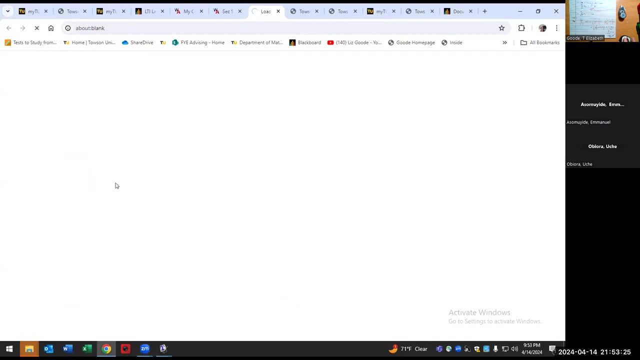 So, but at least now. And you should read in the book. Yeah Right, Because you know I'm going to share my screen. Don't underestimate this. Read it And it'll take you to the book where you can read about. 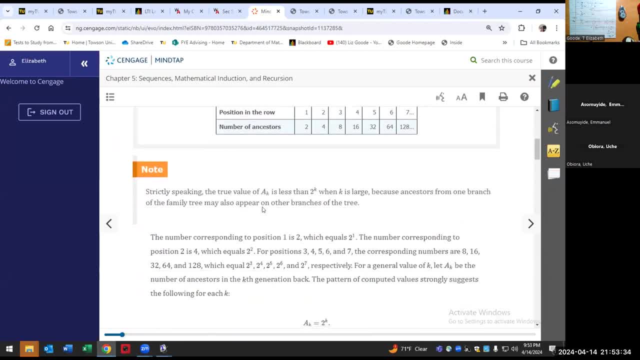 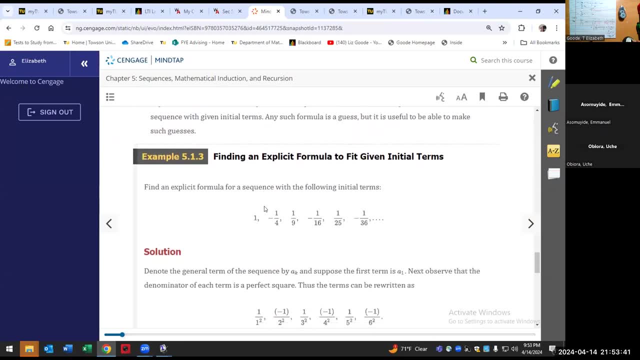 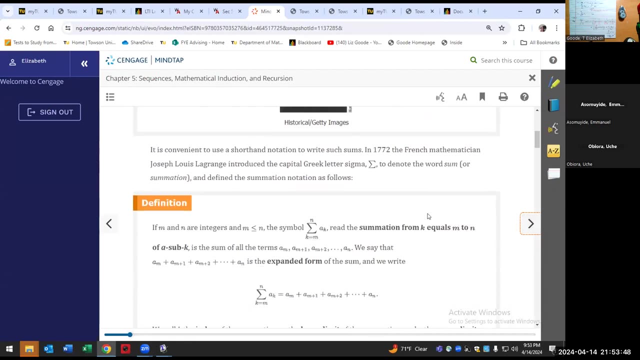 Well, that wasn't a very good pointer. Here we find explicit formulas, summation: Let's keep going until it talks about breaking off the final term. Okay, Okay, So this is going from. Okay, So this is going from m to n. just kind of in general. 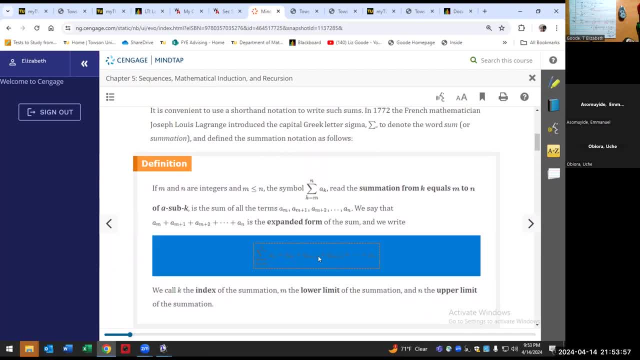 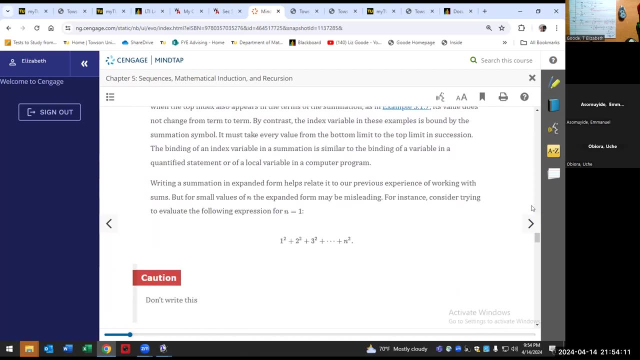 Start it with m. The next number is m plus 1.. The next number is m plus 2.. The next number All the way up to where k gets to be n. Okay, That's very, very general, But somewhere in here they're going to talk about separating off the final term. 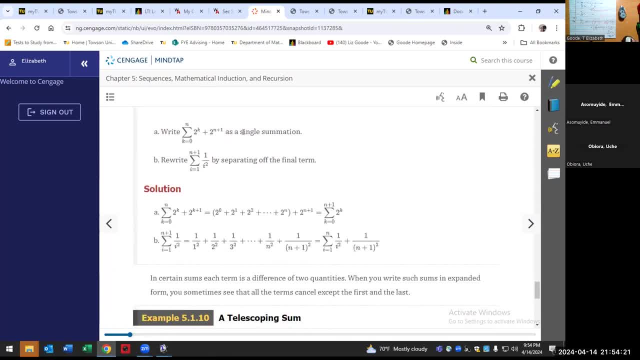 Okay, Okay. So it says: Well, this is where that final term is already separated off to See what it is. It's 2 raised to the k. Okay. So k starts at 0 and goes to n. 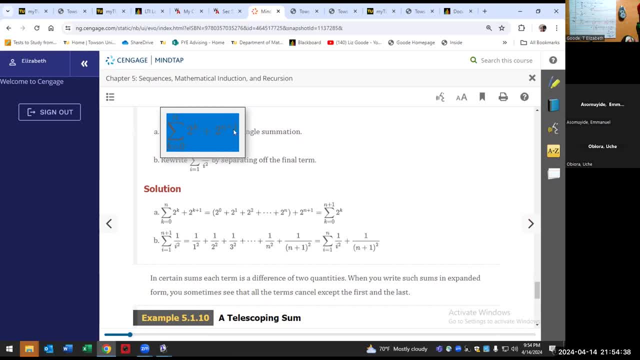 But then they have this other term, plus 2, to the n plus 1.. You see, n plus 1 is 1 bigger than n. So what they're saying is, if you look here, they're saying, oh, you've got the sum from. 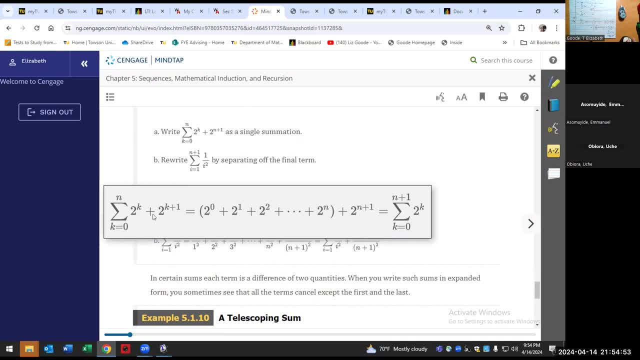 k equals 0.. 0 to n, of 2 to the k plus. they've got this extra term. What the heck is that? Oh, It's the term when you could let k equal n plus 1.. This is actually a typo. 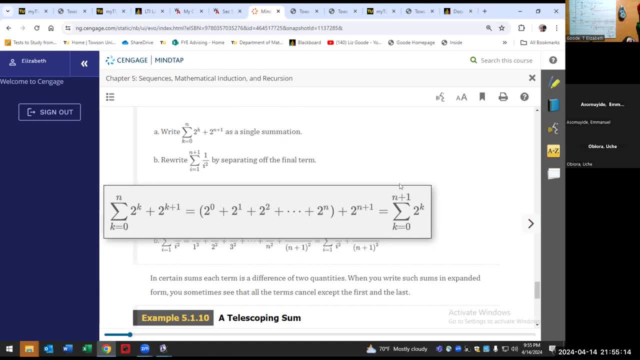 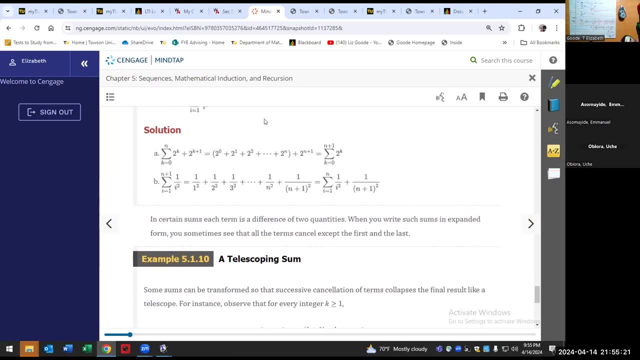 This should be 2 to the n plus 1.. That's actually a typo there. Darn it. They made a typo. All right, Let's see if they did it right here Here The second one. All right, They said: rewrite this by separating off the final term. 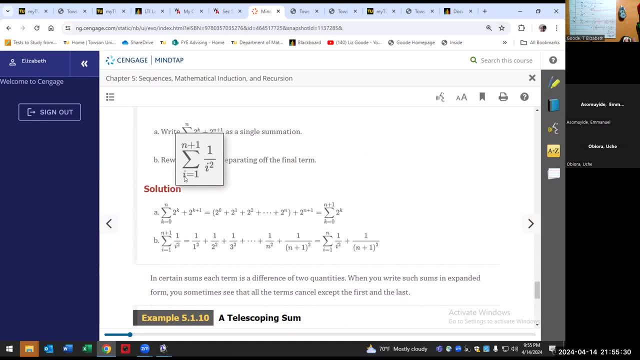 See, when you think about it, what are the terms? Well, the terms start when i is 1.. So the first term is 1 over 1 squared. What would the next term be After i equals 1,? what's the next value of i? 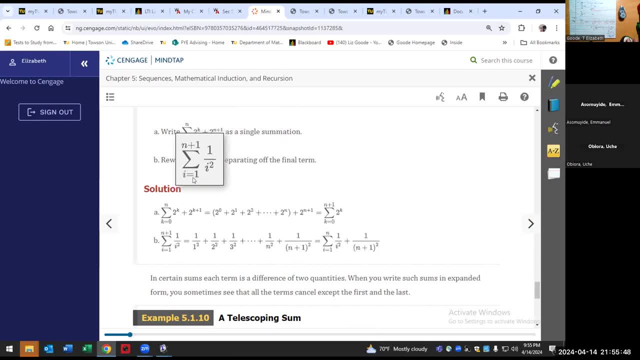 2., 2., 2.. So the next term- and there's a plus between the terms 1 over 2 squared. See, they've got that here- The next term is 1 over 3 squared. When you think about it, it keeps going and going and going until i has this value: n plus 1.. 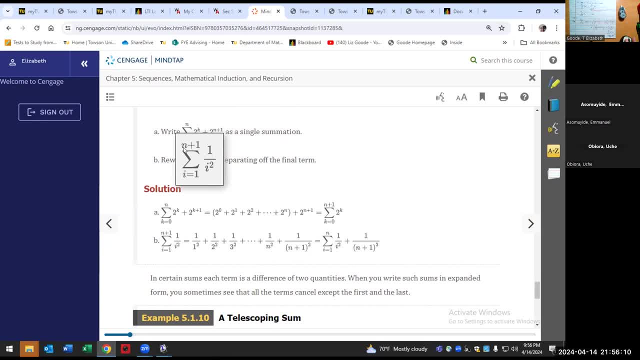 But what is the integer that comes right before n plus 1? n, right? I mean the integer right before 8 is 7.. The integer before 39 is 38.. The integer before n plus 1 is 1 less than that. 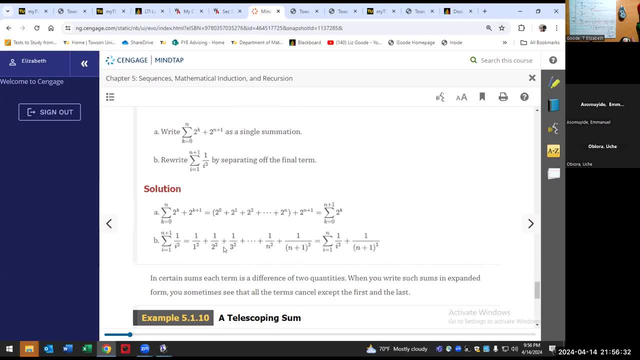 It's just n. So they're saying, hey, you can write this: sum from i equals 1 to n plus 1, like this right. And they're showing that the term before is when i is equal to n. And then they're showing that, hey, you can write the sum of these first n terms. 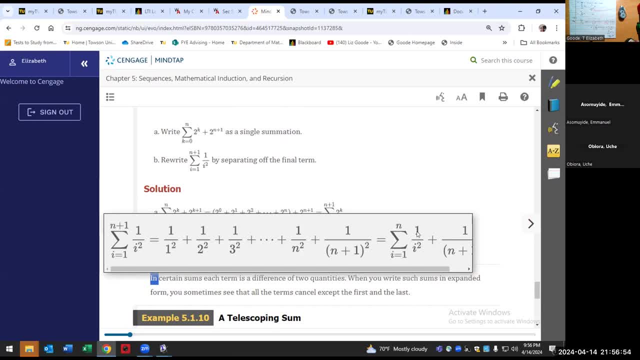 As the sum from i equals 1 to n of 1 over i squared, And then plus this last term which they've broken off. The n plus first term has been broken off, But these two sums they mean the same thing. 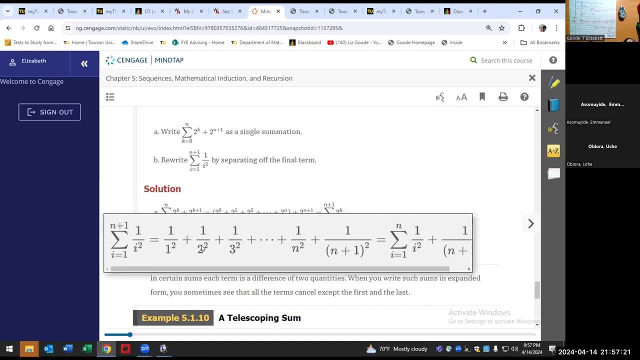 We've just written 1 over n, 1 over 1, squared, plus 1 over 2 squared, plus 1 over 3 squared, plus dot, dot, dot, Plus 1 over n, squared as a single sum. with this expression, The sum as i goes from 1 to n. 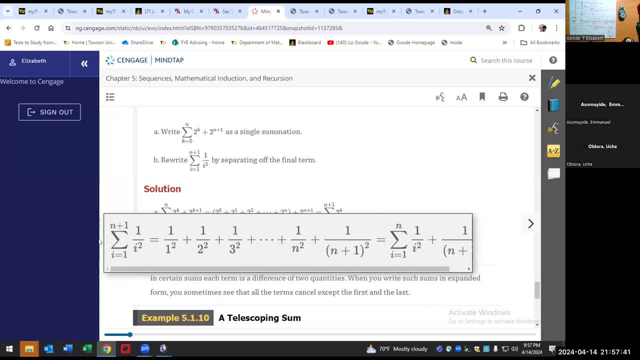 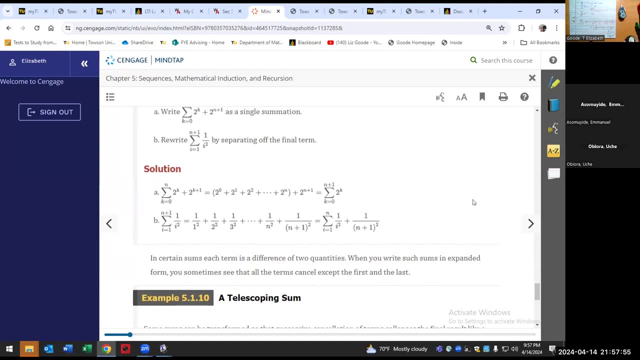 And then this last term, which used to be part of this sum that we started with, is being left out and just hanging off the n by itself, But it's perfectly legal. They all mean the same thing. Does that make sense? All right? 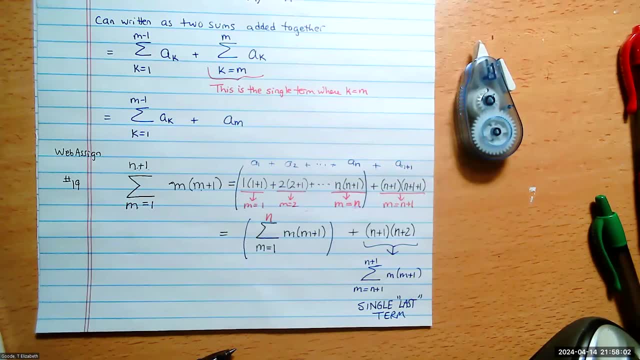 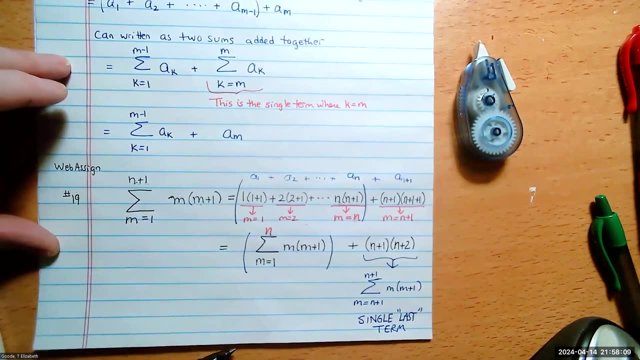 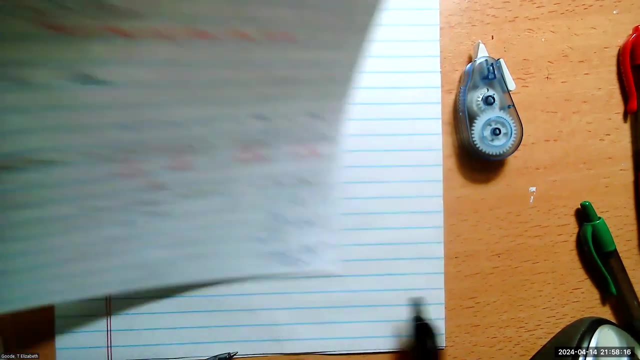 Maybe not. Let's do another one. I have a question. Yeah, go ahead. So if it is n minus 1, would it also be n as well? Ah, that's a great question. Let's look at an example like that. 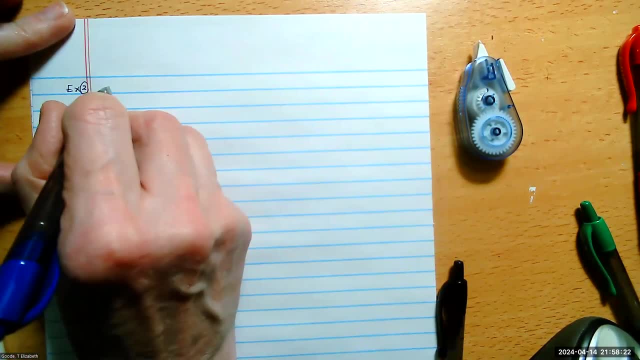 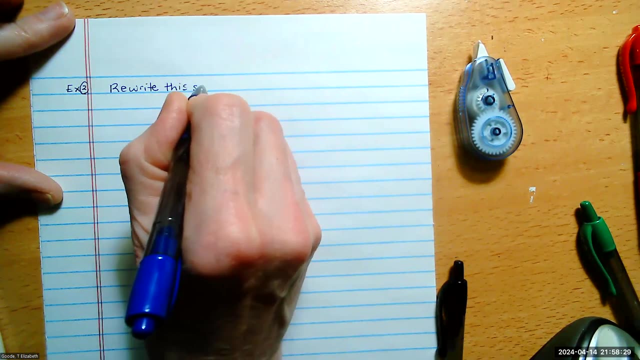 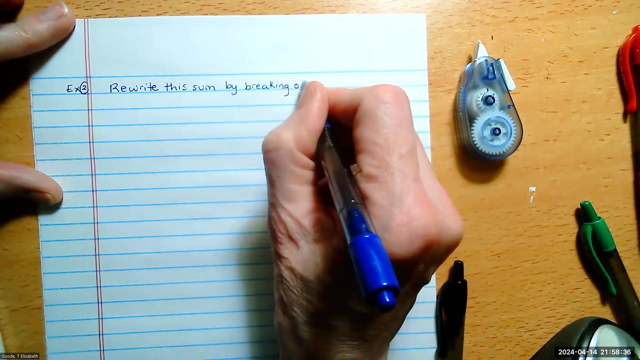 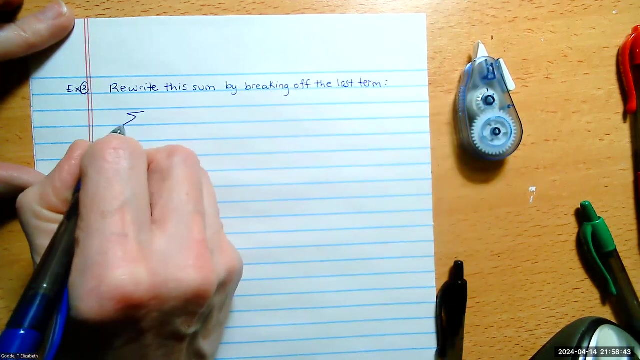 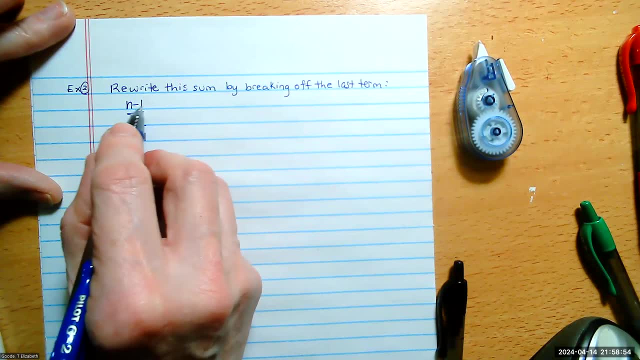 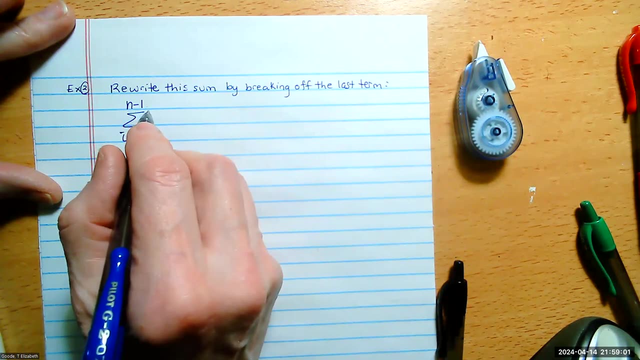 What happens? What happens, What happens? Is that what you're saying, that the upper limit is n minus 1? Yes, Or is that not what you meant? That's what I meant. All right, We can look at several. 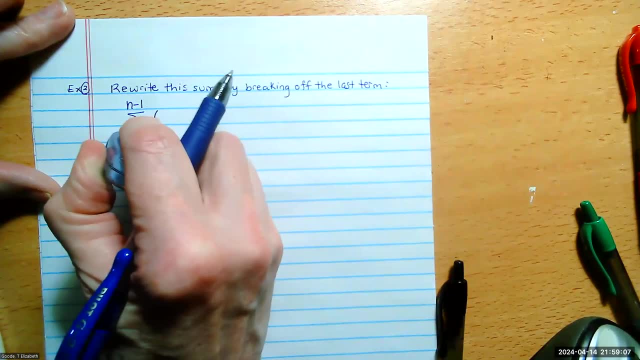 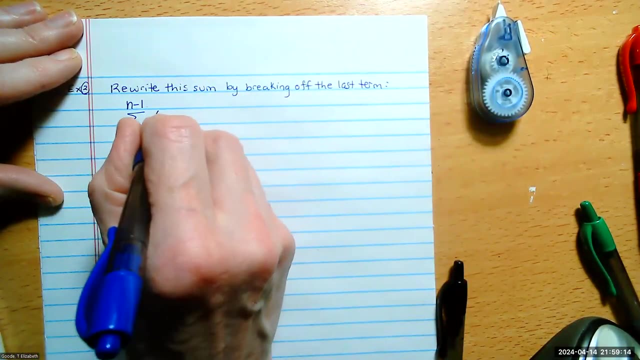 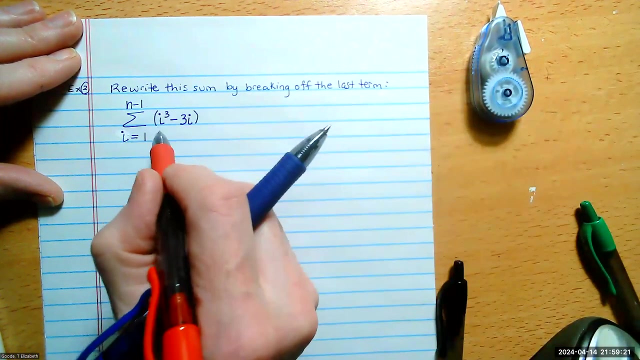 All right. So let me make something up: Oh, instead of i, I'm going to use Oh, why not? Let's just use i? Let's say it's i cubed minus 3i. All right, Let's say that's the term: a sub i okay. 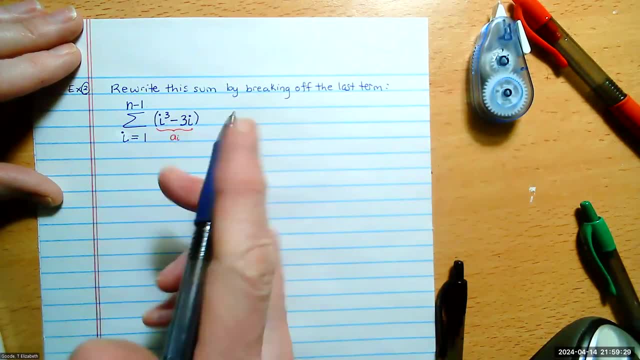 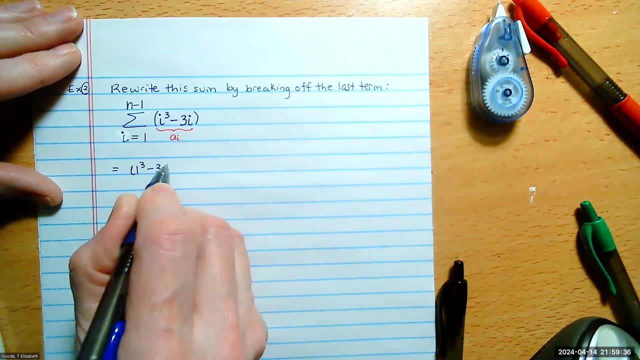 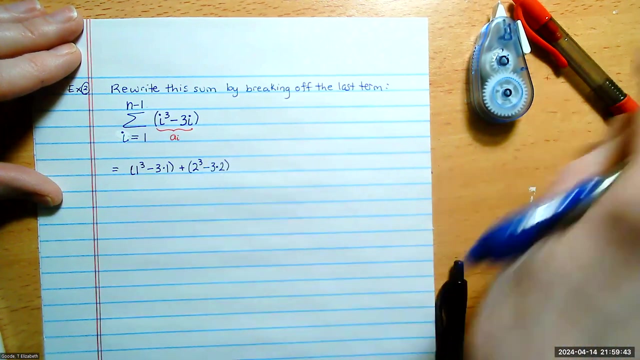 All right, so that's what we're starting with. So we need to realize this is, you know, 1 cubed minus 3 times 1, plus 2 cubed minus 3 times 2, right, You with me. 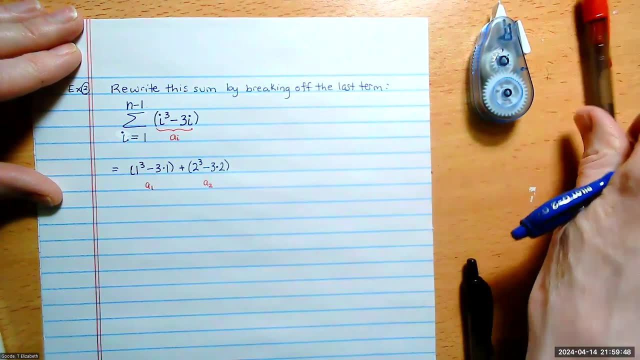 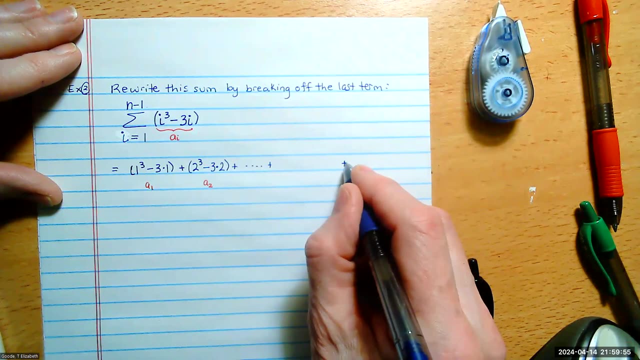 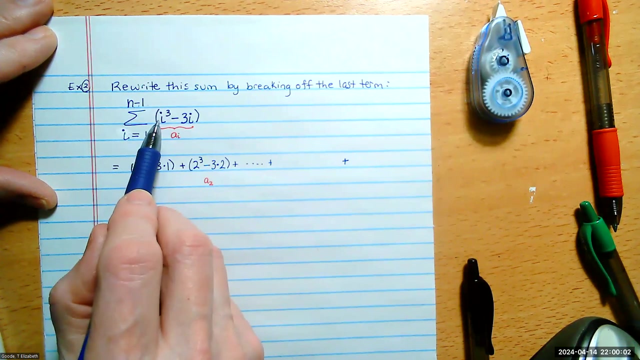 This is a sub 1.. This is a sub 2.. Keep going. I'm going to leave some room here for the term that's called the penultimate term, the term before the last term. What is the last term? It's when i equals n minus 1, okay. 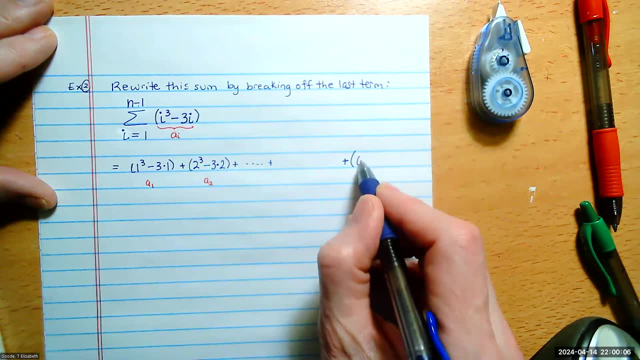 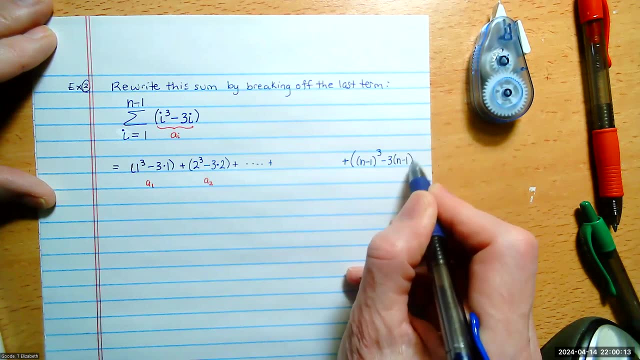 So we're going to plug in n minus 1 for i, So it's n minus 1 cubed minus 3 times n minus 1.. All right, so do you agree that this is a sub n minus 1? Yes, 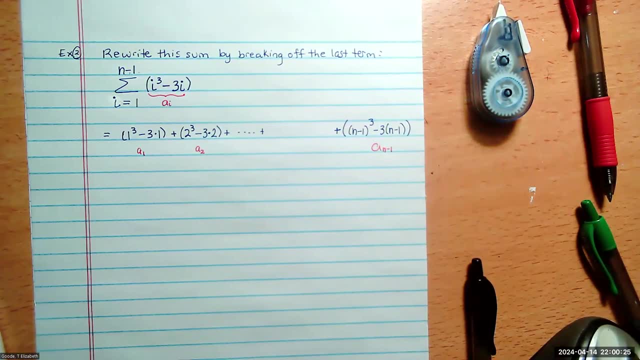 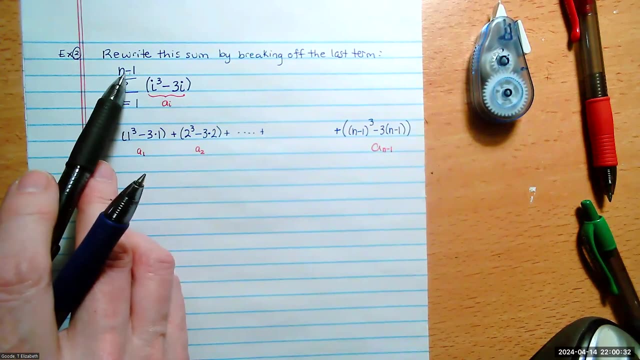 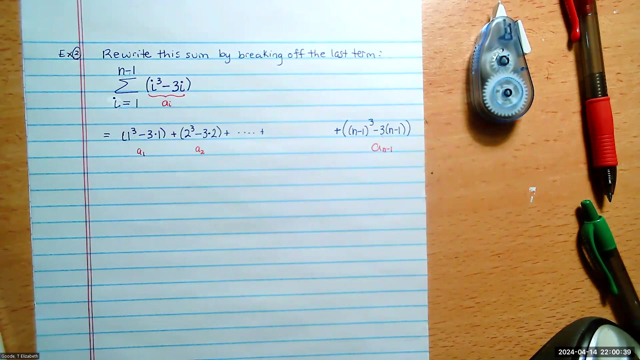 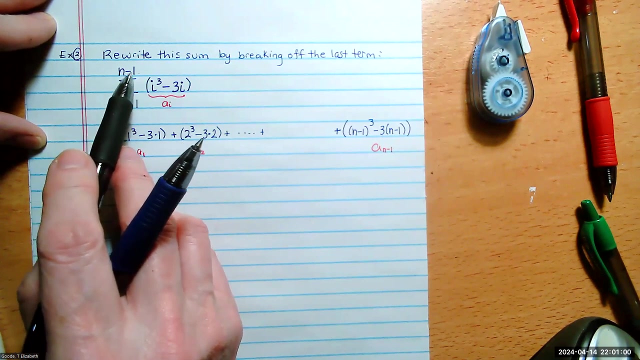 Yes, All right. What does the term right before that look like? Well, what is the integer that comes right before n minus 1? You tell me. Just subtract 1 from that Interesting n. what is it just n? no, n is one bigger than this. to get to n from n minus one, we would be adding: 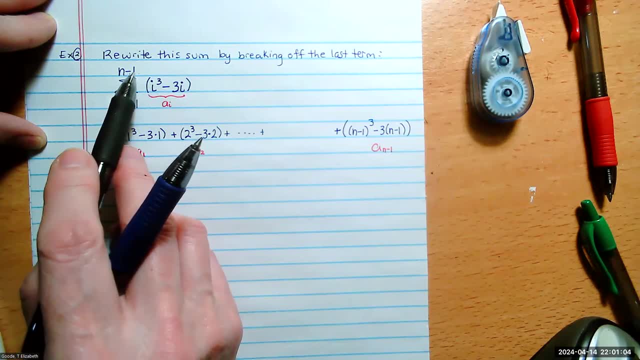 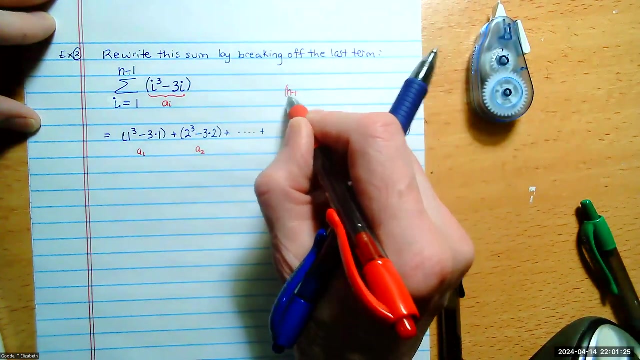 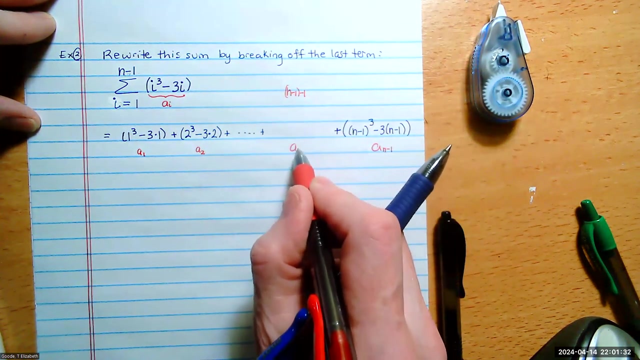 one, the term right before n minus one, the integer that comes right before n minus one, is one less than n minus one. what's one? if you subtract one from n minus one, what do you get? what is n minus one? minus one and minus two, yep, it's n minus two. so the penultimate term, it's the. 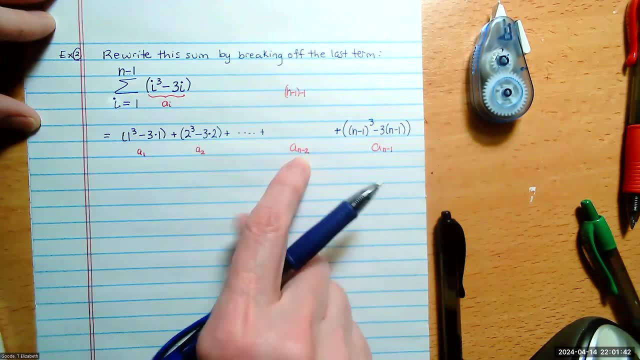 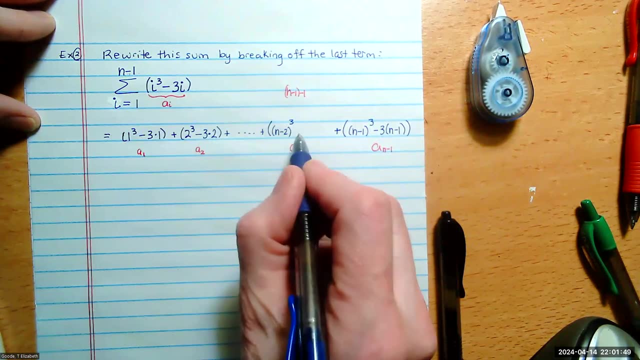 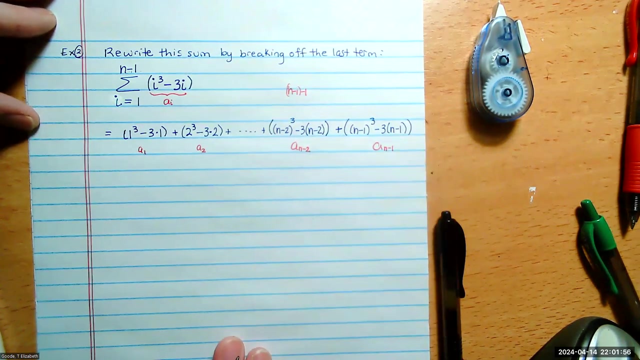 sum only goes to n minus one. so the sum only goes to n minus one. so the sum only goes to n minus two. n minus one would be the n minus two term and it would look like n minus two, because that cubed minus three times n minus two. okay, does that make sense? 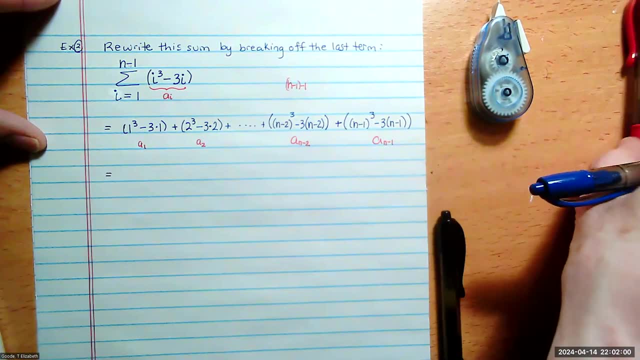 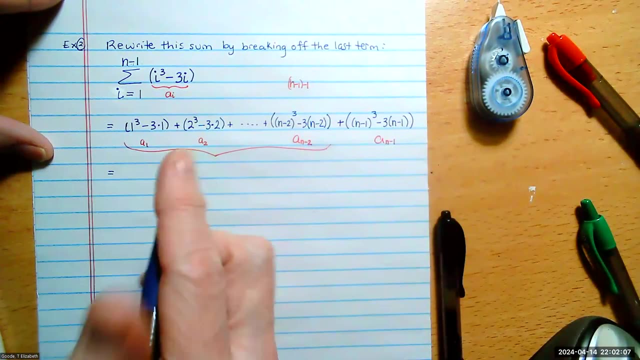 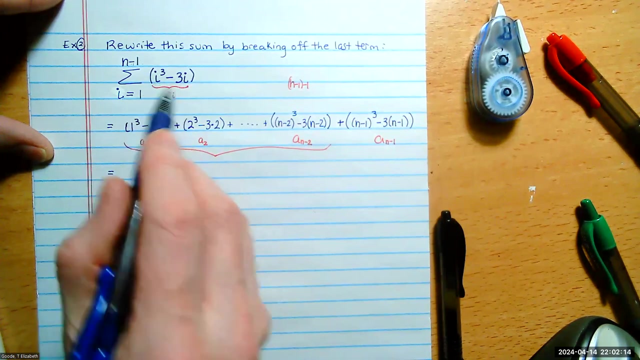 so the point is we can gather these together, these all these except the last one, into a single sum. this is the sum. this is the sum starting still at i equals one a sub. i still looks the same. it's i cubed minus three i. but what is the upper limit of the sum? if we're just looking from here to here? 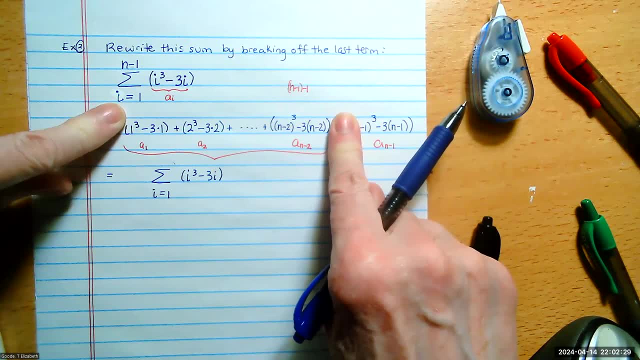 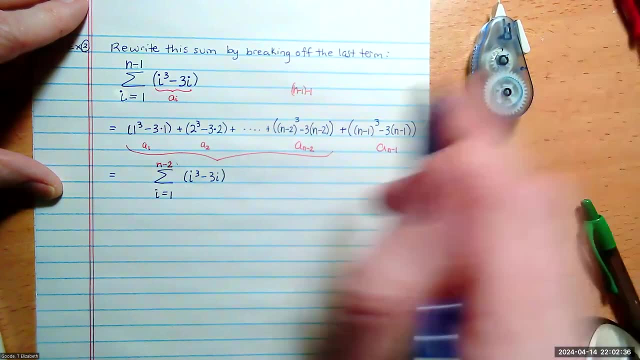 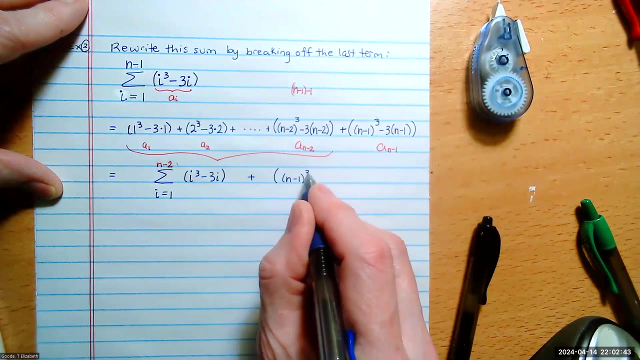 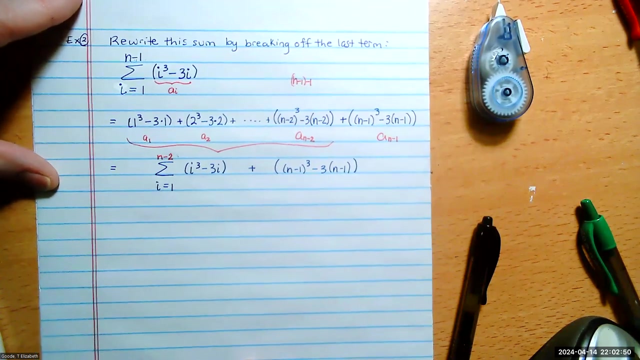 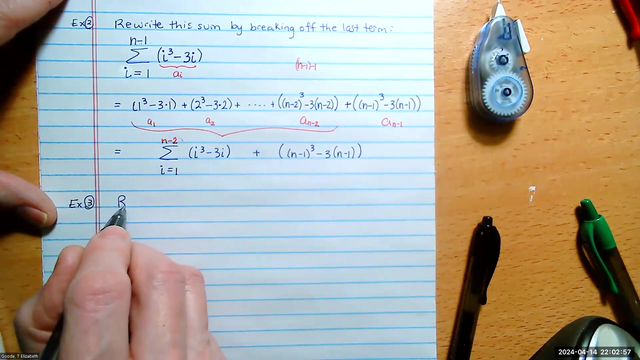 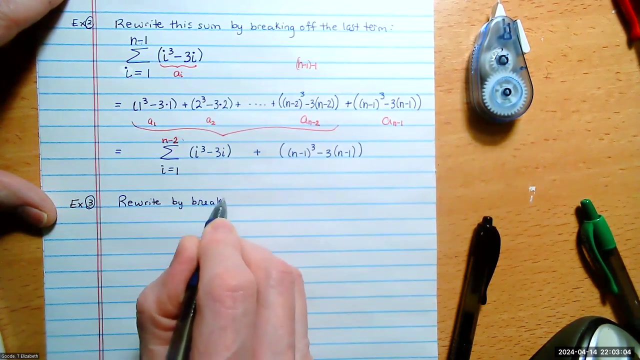 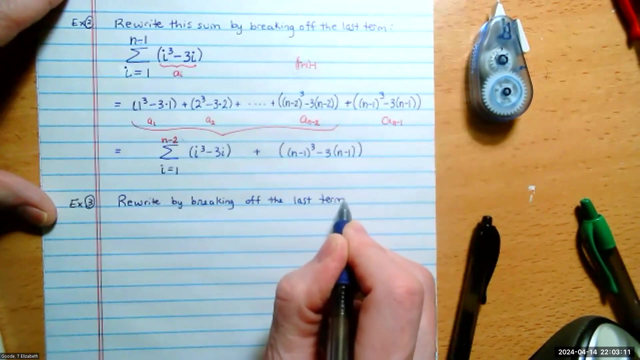 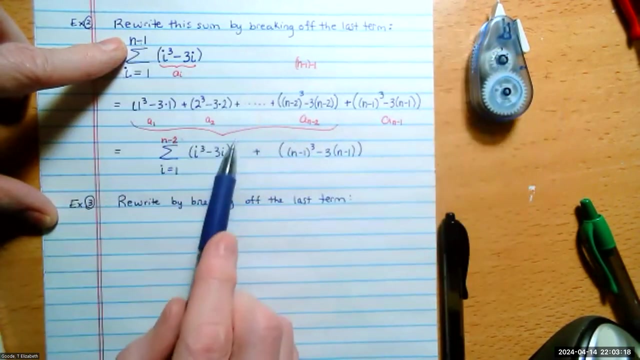 what? n minus two? yeah, n minus two. and now this becomes the broken off last term. it just happened to be the n minus one term. okay, should we do one more rewrite by breaking off the last term. so again to break off the last term. we have to see what the term before. that is right, we have. 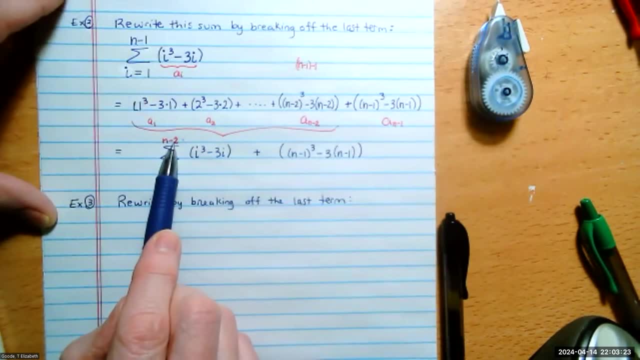 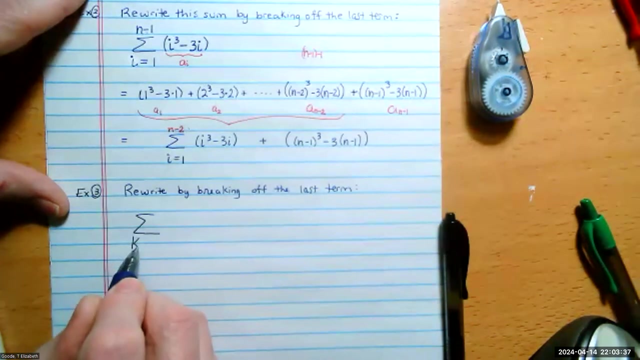 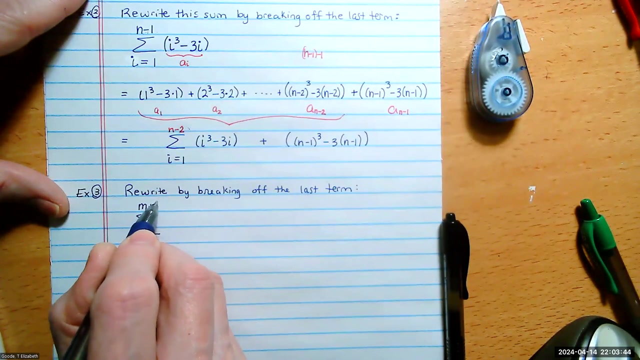 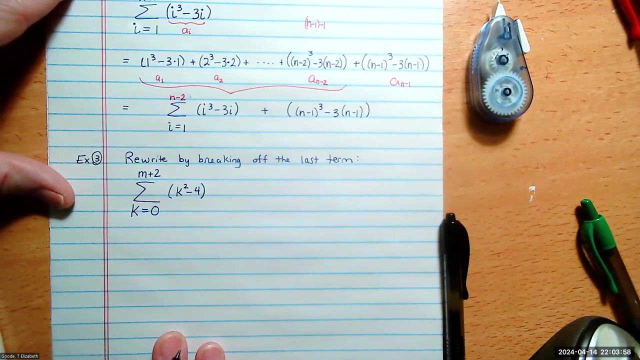 to see what this is. so we know what to put as the upper limit of this new shorter sum where we adding together one fewer terms than originally. how about the sum from k equals zero to three? how about the sum from k equals four to five? zero from k equals 0 to m plus 2 of k squared minus 4.. 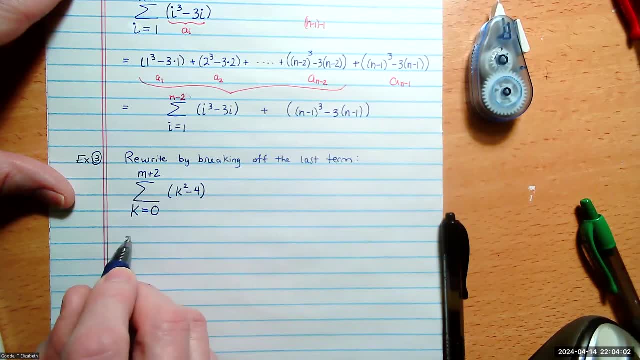 So we realize this is 0 squared minus 4 plus then, when k is 1, it's 1 squared minus 4, plus some more terms, and then there's going to be that penultimate term that we're trying to figure out. 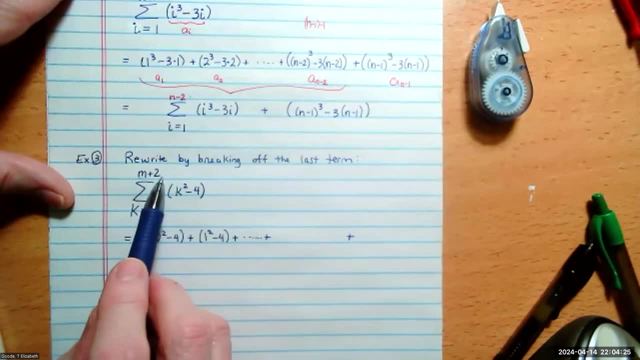 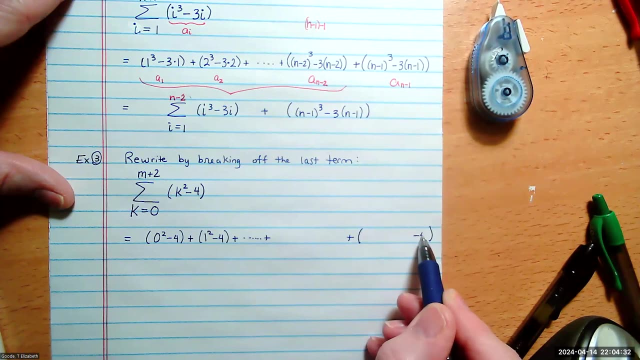 plus. what's the last term going to look like? It will be m plus 1.. That will be the penultimate term. The last term is m plus 2 squared right, And you're right. this penultimate term is m plus 1, squared minus 4.. 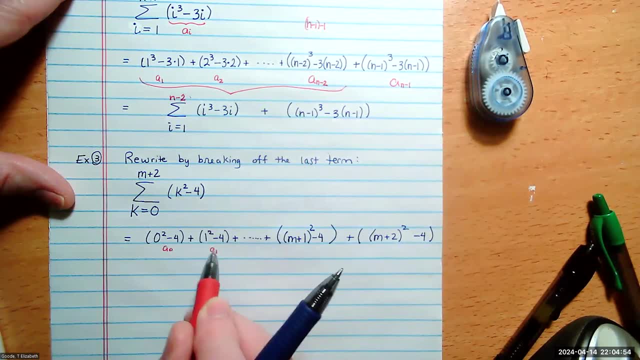 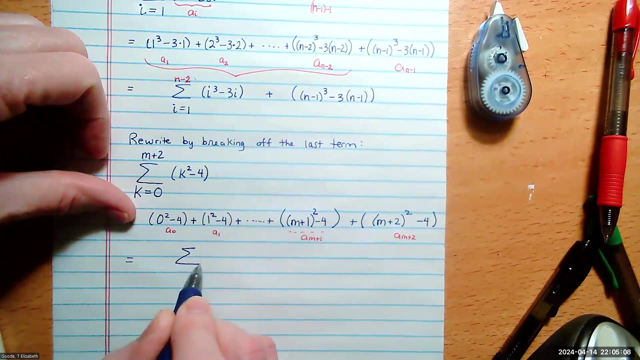 This is a 0,. this is a 1.. This last one is a sub m plus 2.. This term is a 1.. is a sub m plus 1. so when we run, write this as a sum. right, this is the sum from. 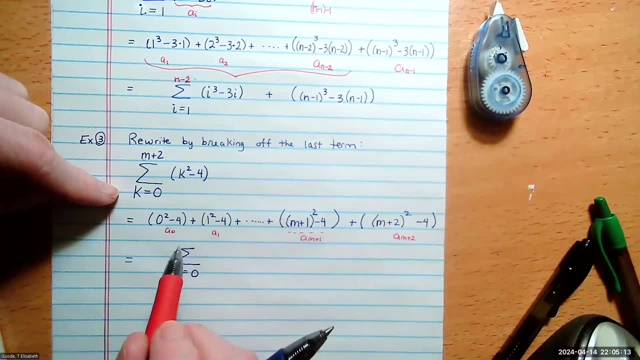 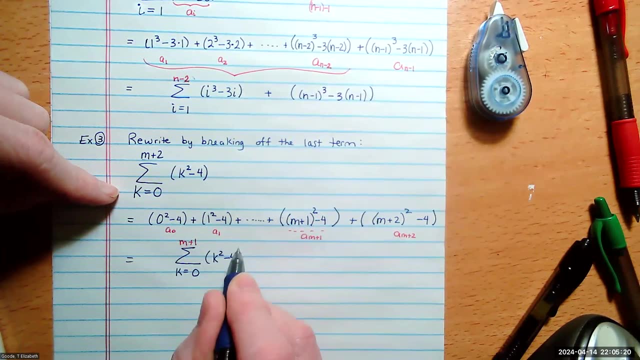 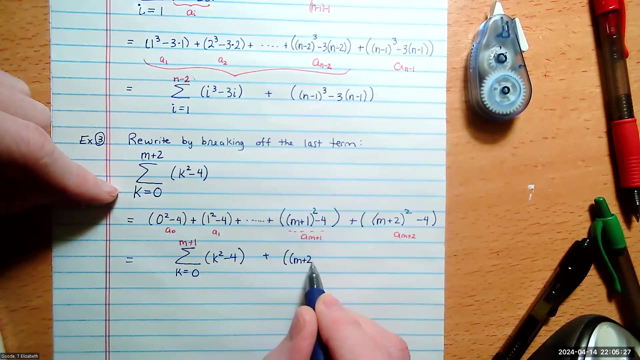 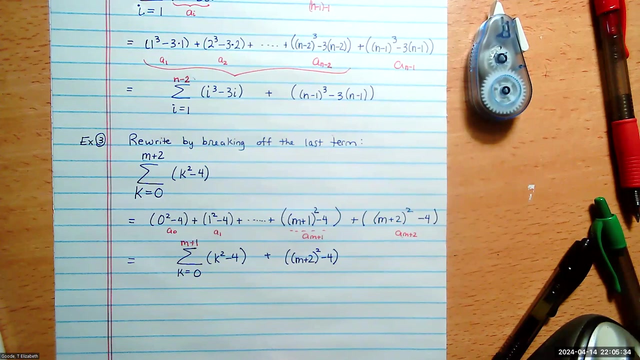 k equals 0 to m plus 1 of k squared minus 4, and now our broken off term is that m plus 2nd, m plus 2th term. does that make sense? yeah, okay, I'm not saying it's easy, but it is something that one you know once. 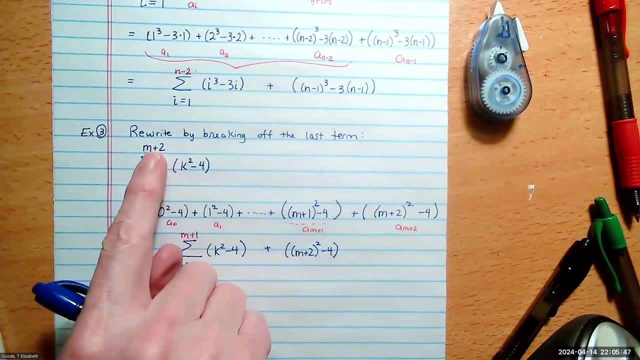 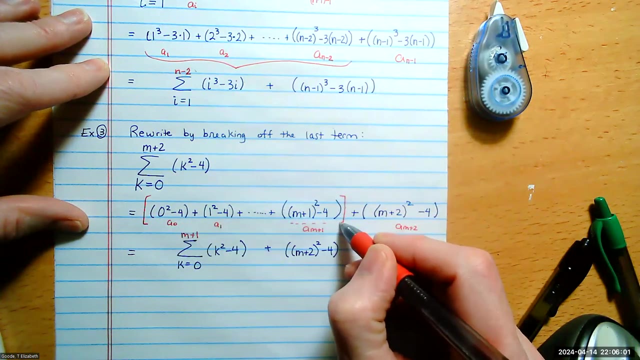 you see enough examples, it starts to make sense. you just have to figure out what the integer is right before this, and that becomes the new upper limit right before this, and that becomes the new upper limit right before this, and that becomes the new upper limit of this shorter sum. right, because we're only adding together that all the terms. 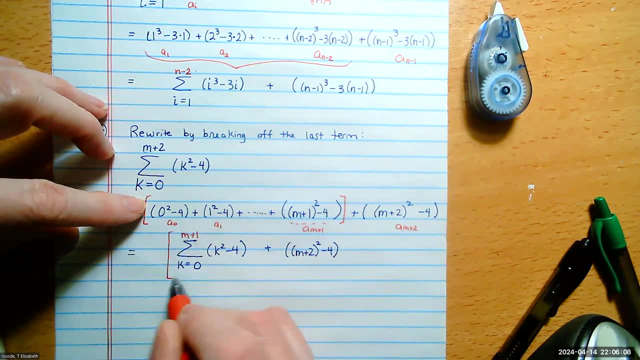 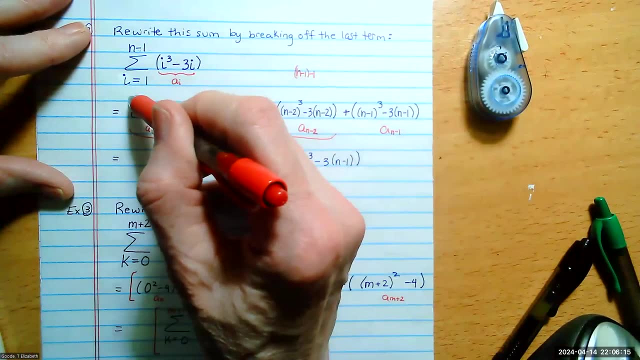 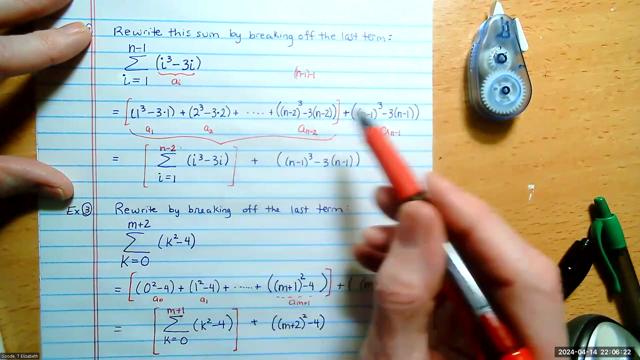 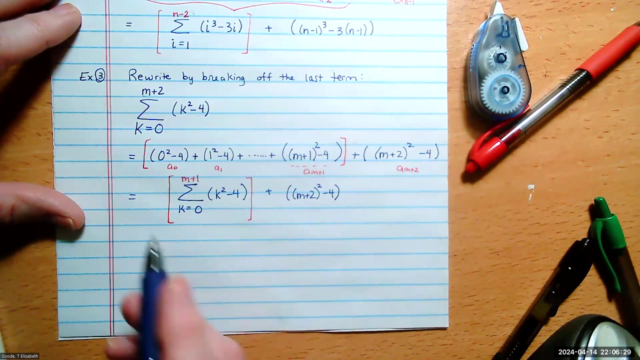 except for the last one up here. it was all the terms, except for the last one, which then just hangs up here. it was all the terms, except for the last one, which then just hangs off at the end, off, at the end off, at the end. okay, listen, you know, in general, our most. 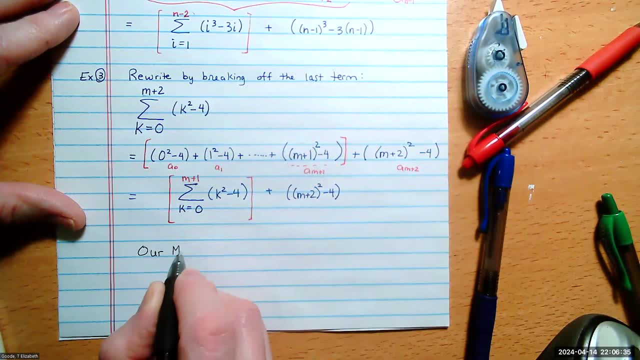 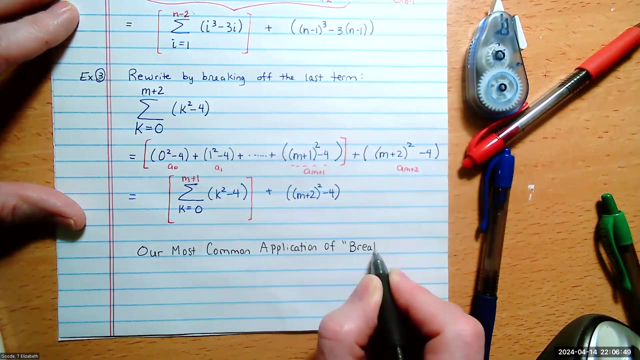 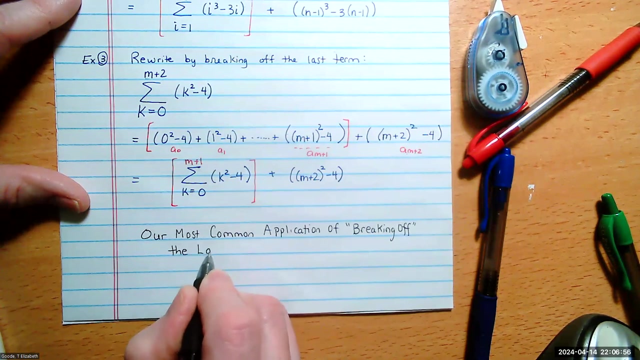 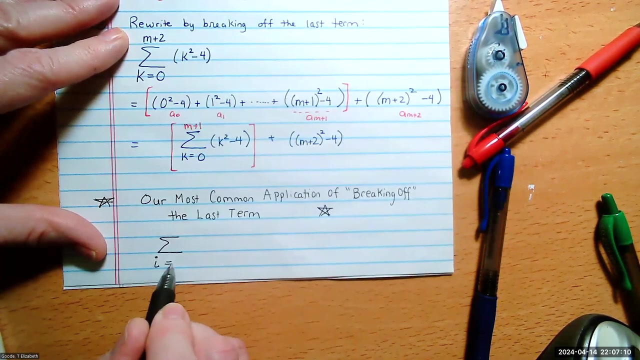 okay, listen, you know, in general, our most. okay, listen, you know, in general, our most, our most common application of this breaking off, breaking off the last term, there is a, you know, a fairly common application in proof by induction, which is what we're going to start looking at, is when we have the sum from: i equals. 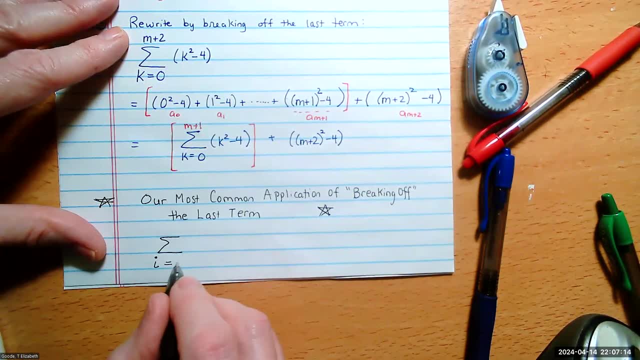 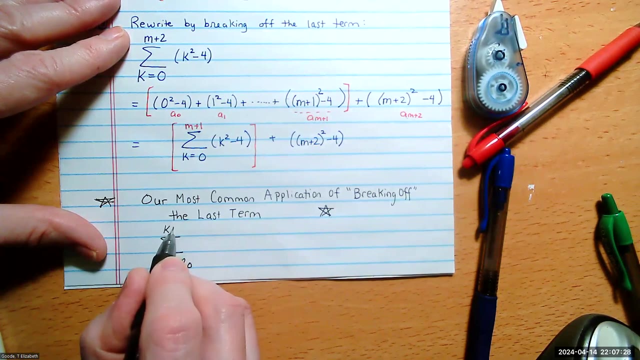 you know some bottom level number. I'll call it. it may not be zero, it could be something else. I'll just say n sub zero, some lowest level, but usually we're going up to k plus one of some term, a sub i. this could be, you know. 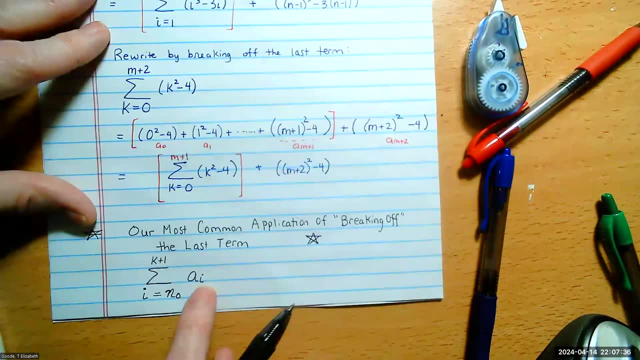 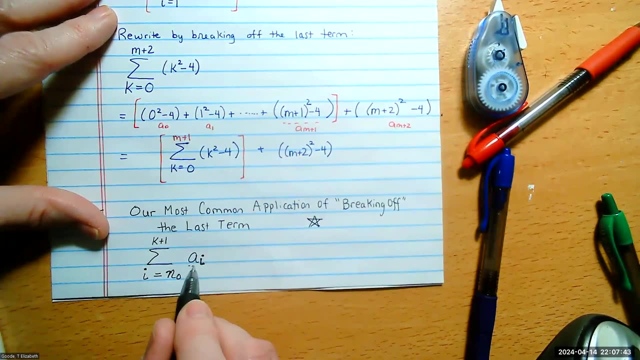 k squared minus four, or it could be i cubed minus three i, or it just could be k i cubed. you know whatever it, you know whatever. this is isn't really the hard part, the hard, you know, the interesting part. 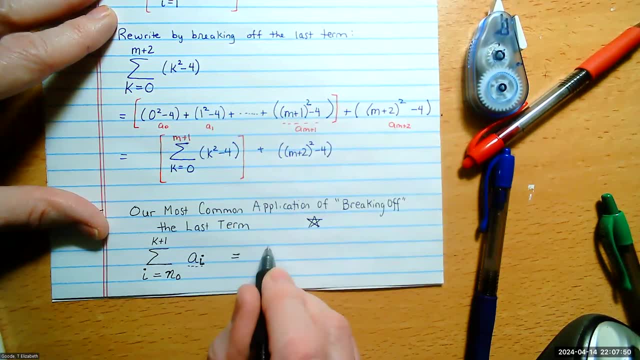 The interesting part is happening here is that we write this as the sum from i equals whatever it starts at. it could be zero, it could be one, it could be two, it could be three as the lower limit, but we go to the term before. it's usually the kth term and 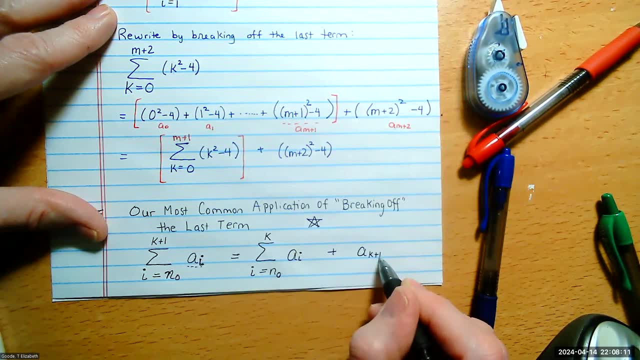 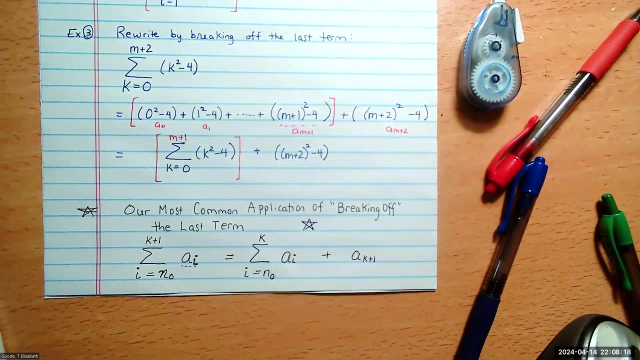 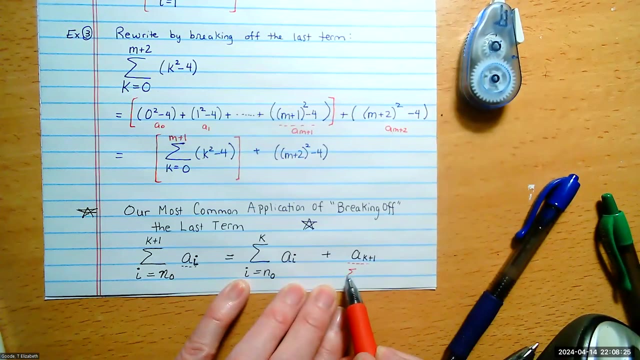 then the broken off term is the k plus first term. Okay, This is actually literally the sum from i equals k plus one to k plus one of a sub i. That's actually what this is. it's just a single term where the lower limit of the sum 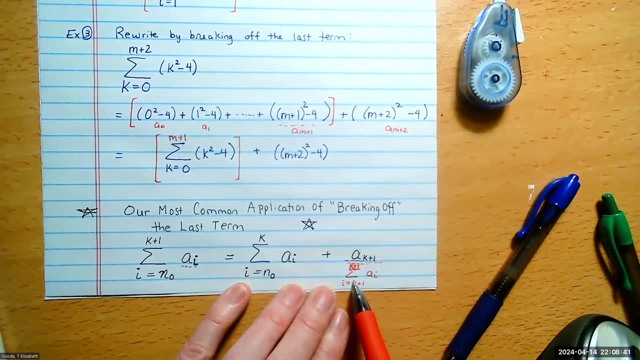 is k plus one and the upper limit of the sum is also k plus one. That's perfectly legal In summation notation, If the lower limit and the upper limit are the same number, it's just the single term where that number is getting plugged in, for i 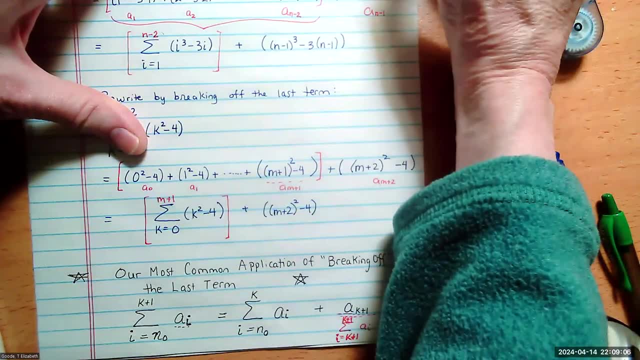 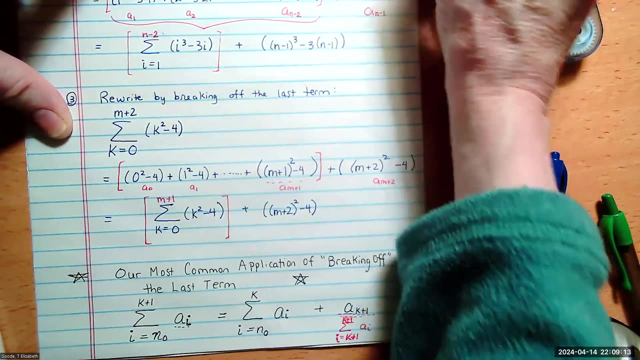 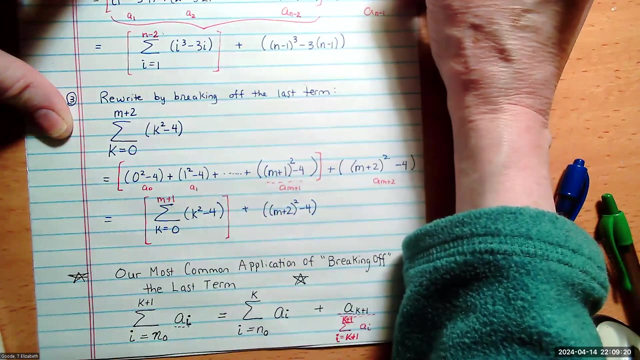 All right, gentlemen, it is 10.09.. So, unless somebody's got a burning question, Okay, I have a last question, So it's the last one. All right, I understand, I offer to keep going. It's okay, you're good. 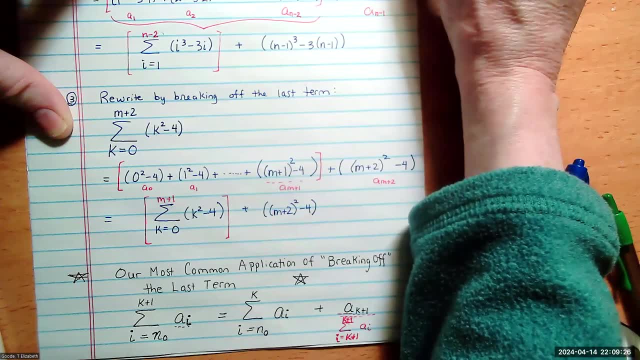 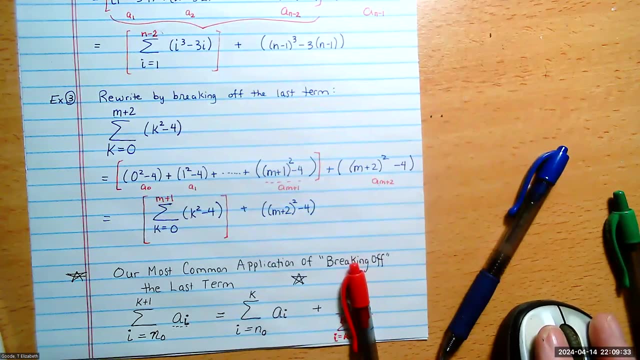 What is it? Yeah, it's just the last one, the last number 28.. It's like a I don't know. All right, let me go back. Yeah, Yeah, let me go back To what it's on. 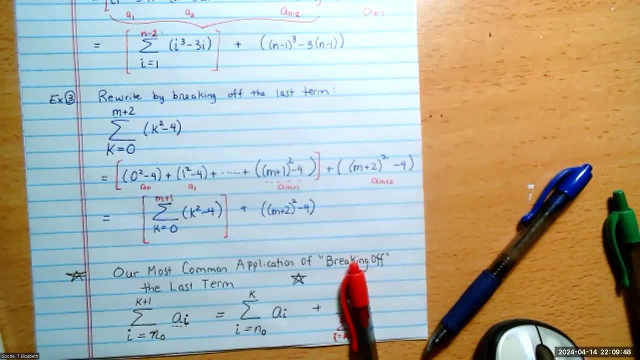 Okay, Does it bump me? I know Number 28.. You want to read it to me while I'm getting this? Okay, So it says: compute the following: Assume the value of N is restricted so that the expression is defined: 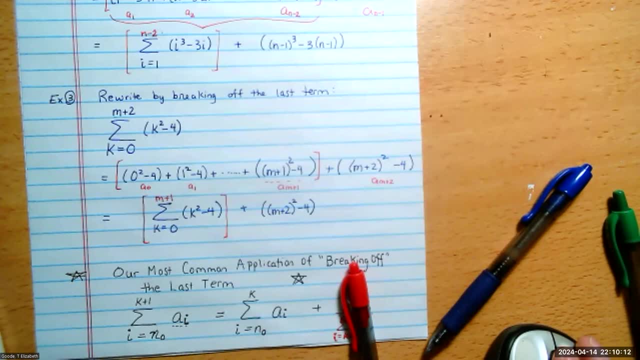 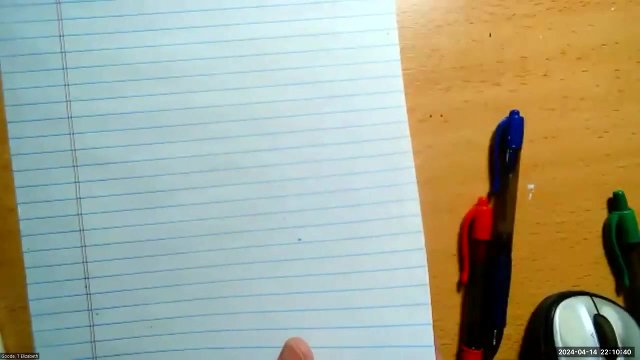 Then it's bracket: N plus one over. N minus one. Uh, okay, So excuse me, Let's see. i don't know if it's over. i feel like it chooses n plus one. yeah, because if you don't see that horizontal line, it's not a fraction, it's choose. 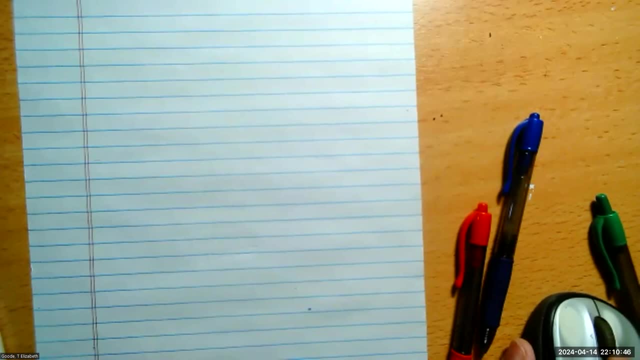 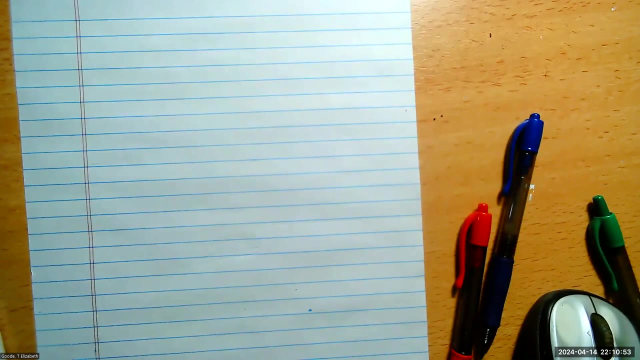 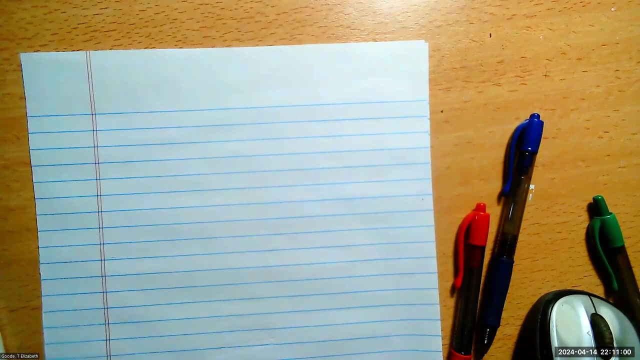 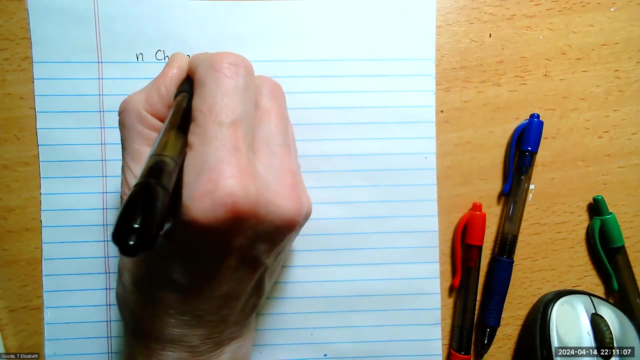 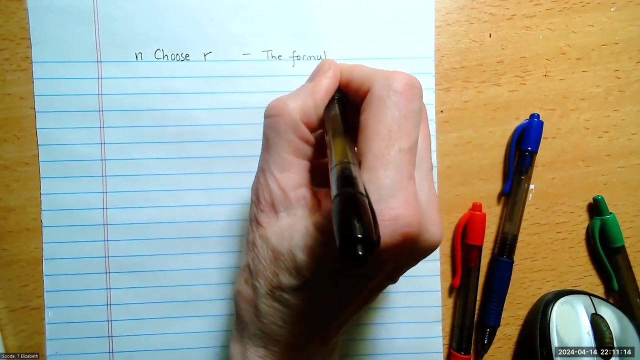 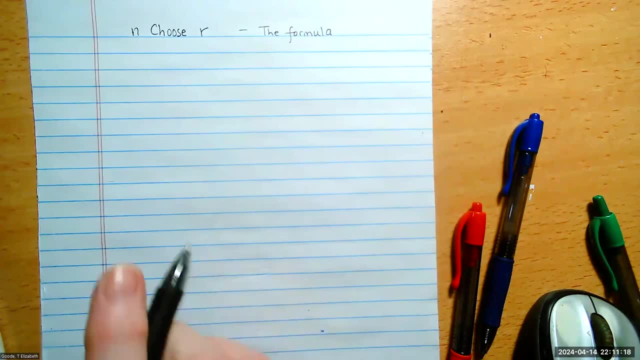 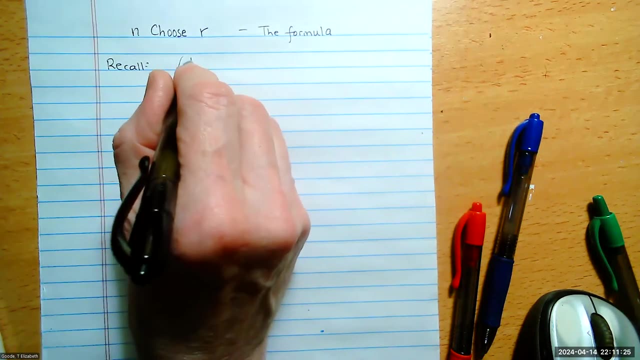 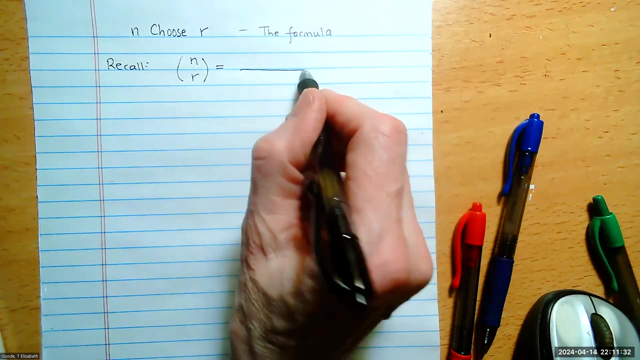 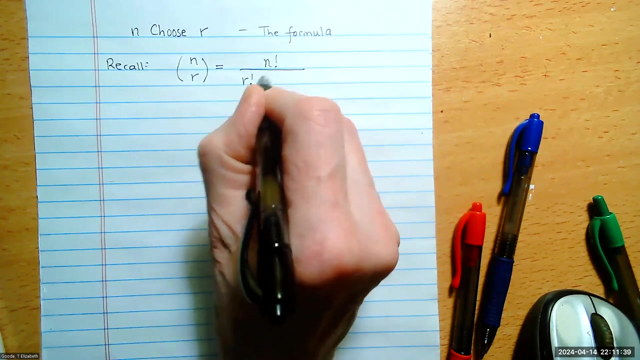 factorial formulas. a lot in class, right? so let's just recall what the formula for n shoes are is. do you remember what n shoes are? is what the formula is. yes, that's um. n factorial over r factorial bracket. n factorial minus r factorial. okay. n minus r quantity factorial. 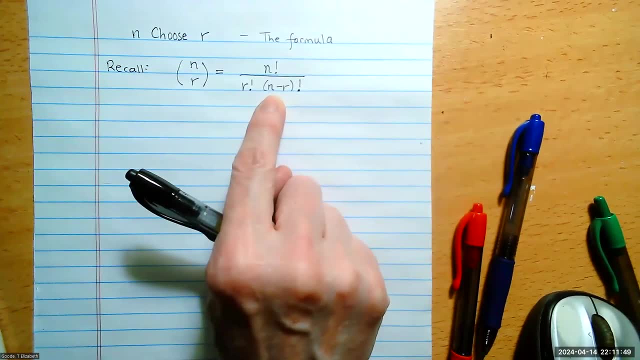 n minus r quantity factorial. that's how we actually read this. we either- that's how we actually read this. we either say bract, usually we just no bracket. okay, fine bracket. n minus r closed bracket, factorial. but the way this is normally red is n minus r quantity, an goddess. 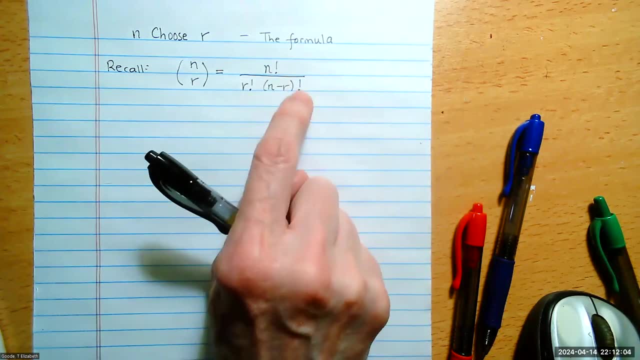 it into the brackets: factorial plus brackets and regular form. that kind of puts it into the brackets: factorial times, extra done, factorial, all right, great, accurately. so you know it says restrict n so that no, it makes sense. but notice n plus r scarce nitrate. if non-physical things, do you start writing☆? 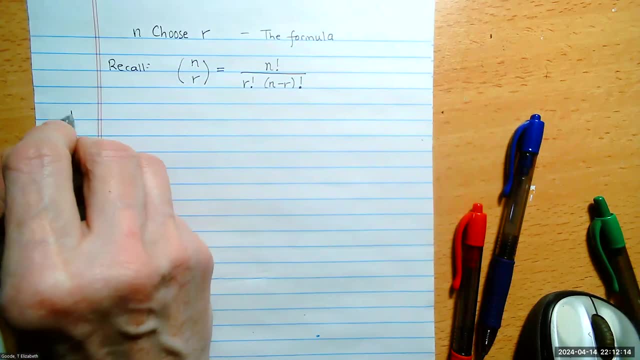 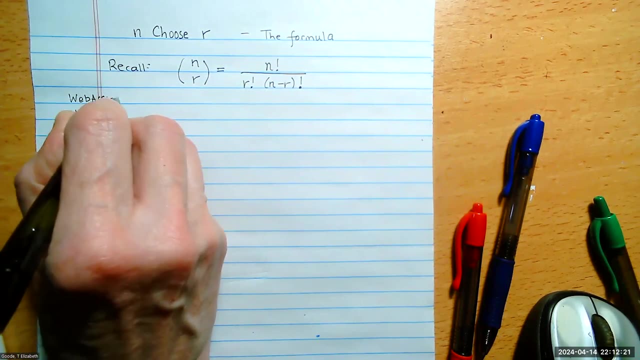 IK material. sorry, start by copying. it never copies what these guys wrote. yeah, that's all right, whole knowledge when you're using it as your database. But let's do a slightly different one, because I don't want to give this one away. All right, see, because this one is n plus 1.. 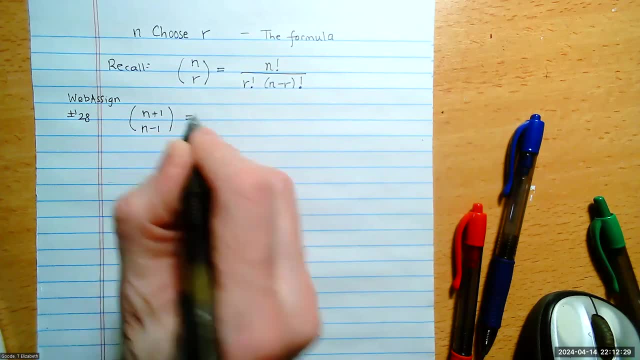 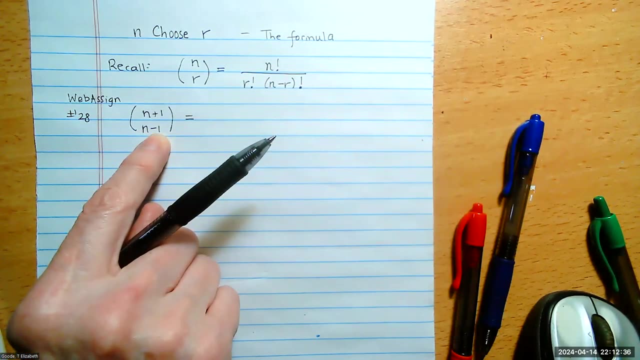 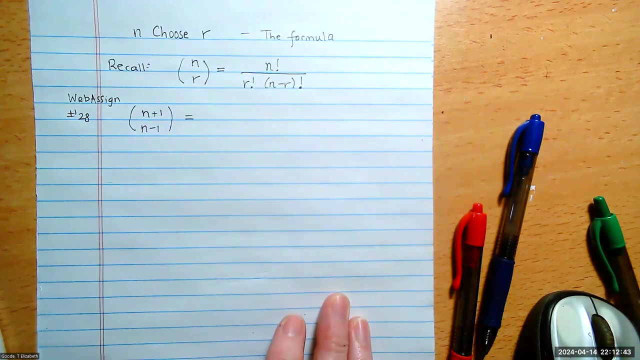 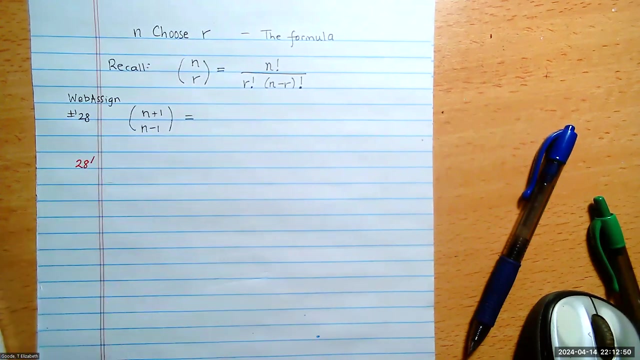 Choose n minus 1, OK, I mean you can just naively plug. you know, r is n minus 1, right? I mean I'm assuming you've plugged these values into this formula. But we can do what I'll call 28 prime, all right. 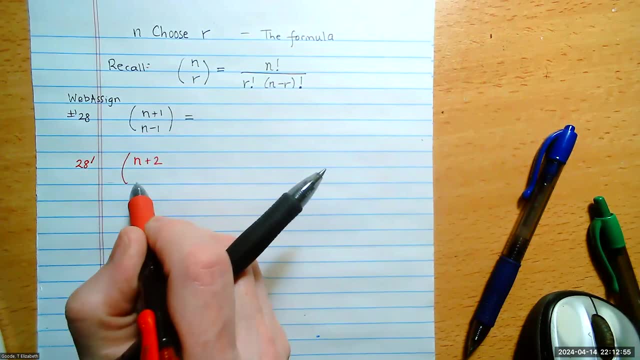 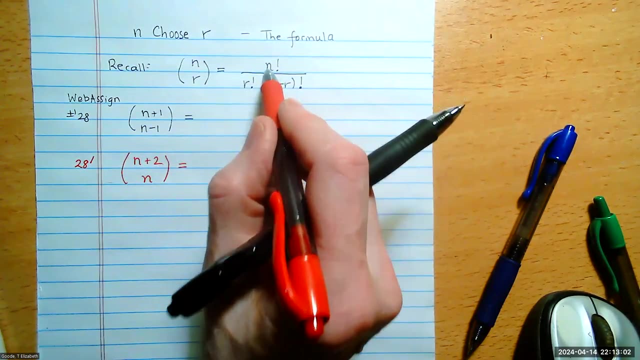 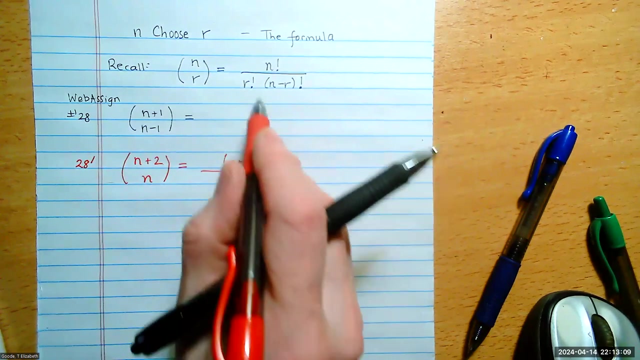 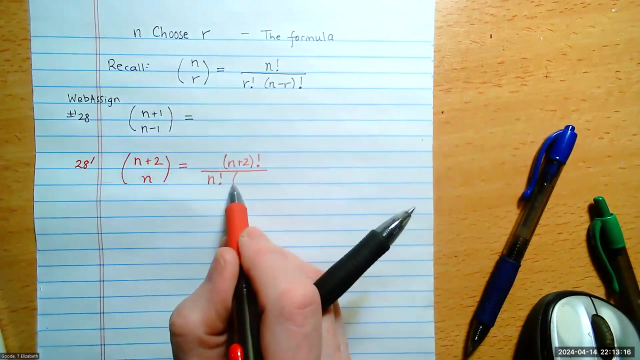 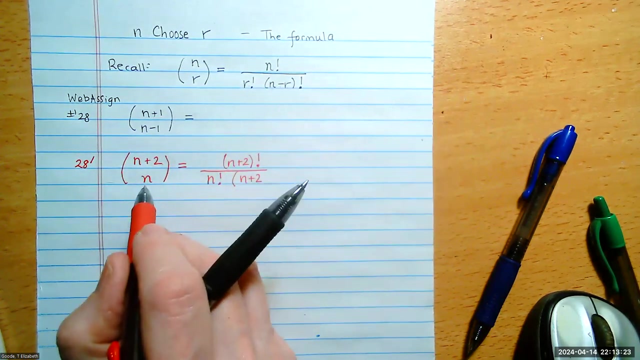 How about n plus 2, choose n, All right, so the top number it's factorialized in the numerator right, The bottom number is down here And then it's the top number minus the bottom number. So the top number is n plus 2 minus the bottom number n. 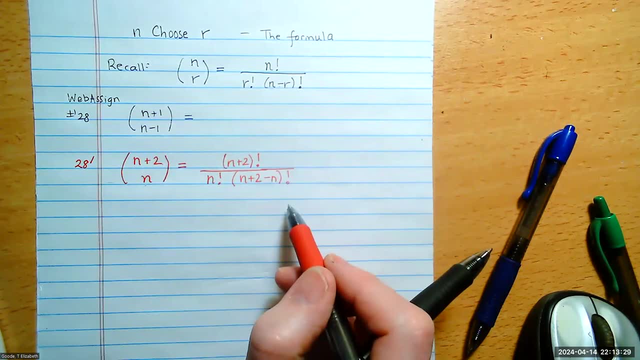 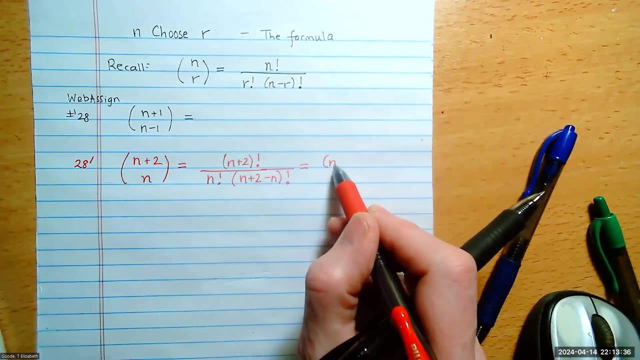 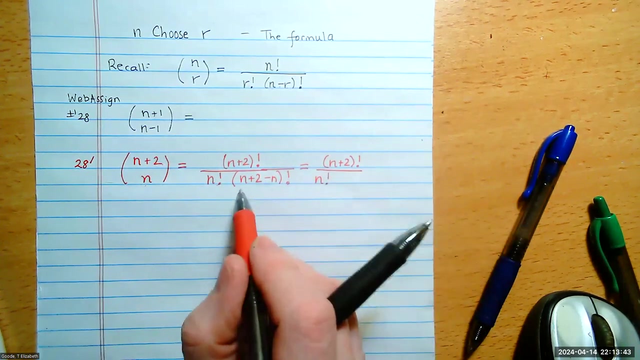 And that gets factorialized. all right, You with me? Yes, All right. so here let's see what happens. In the top we have n plus 2- factorial. In the bottom we have the n- factorial. Let's simplify: n plus 2 minus n. 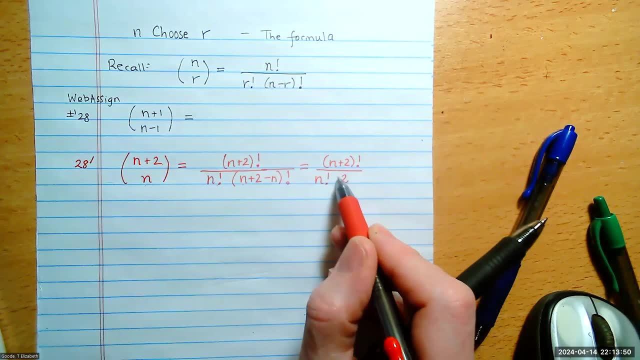 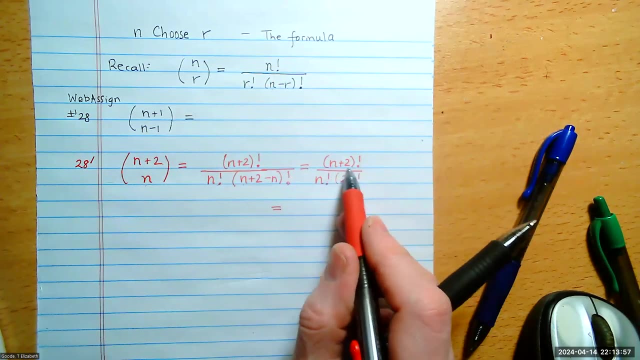 Well, the n minus n cancels, and that's just 2 factorial, Do you agree? Yeah, All right. well, we learned that the thing to do is look at the bigger one. n plus 2 is bigger than n, right? 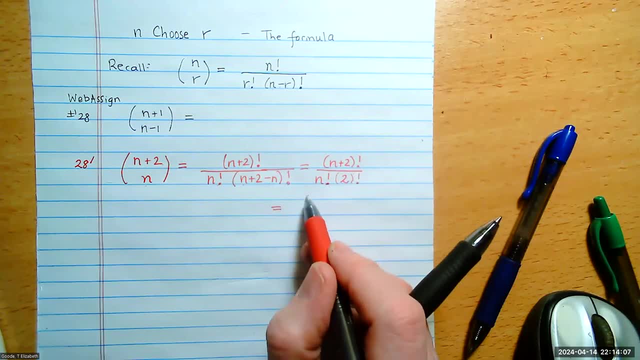 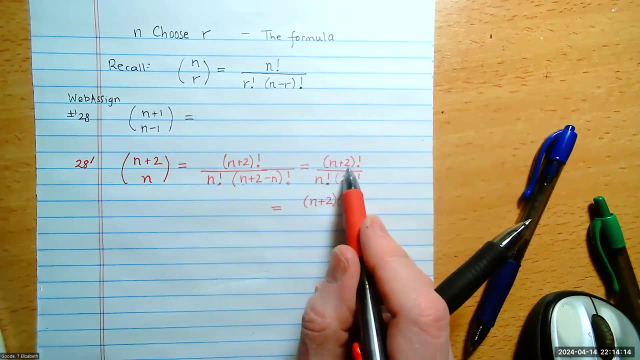 So we're going to break n plus 2 factorial down. It's n plus 2 times the number right before, n plus 2.. What's the number? the integer? that's right, One less than n plus 2.. n. 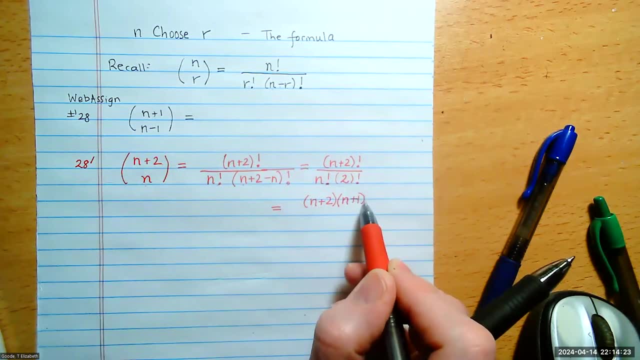 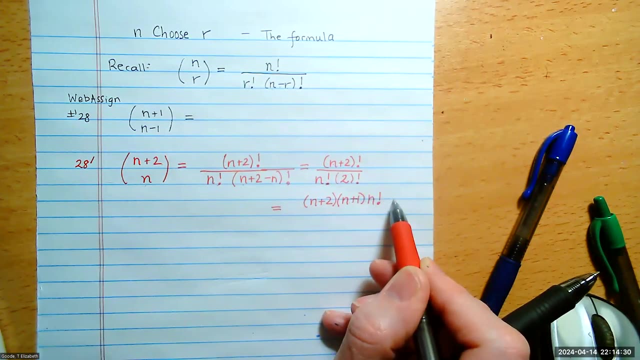 Nope, n plus 1.. There you go. And then what's the one before that n All right, and then we can stop there because it just keeps going Times n minus 1 times n minus right. But the point is, once we see the n factorial up here, 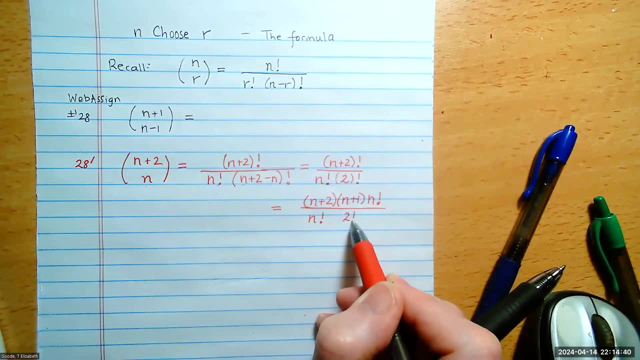 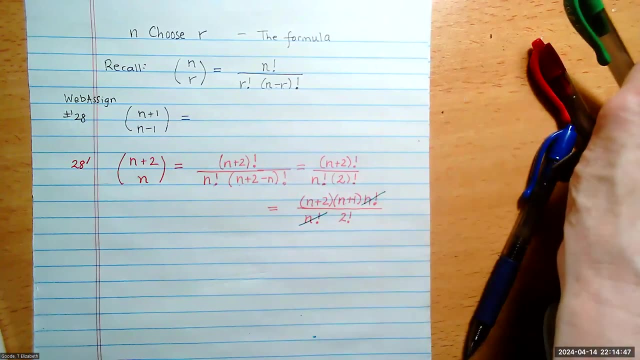 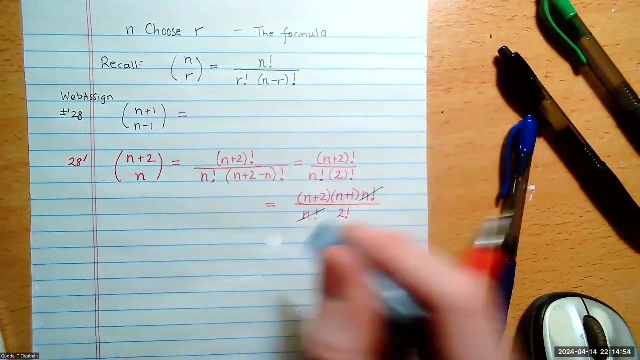 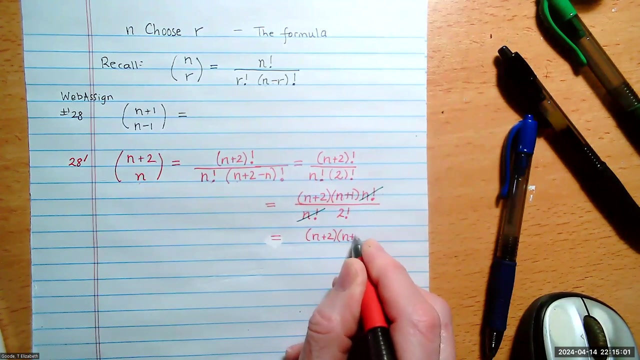 we know it's going to cancel with the n factorial downstairs, right Yeah, So these two cancel And then we have up top. we have n plus 2 times n plus 1.. We can just leave it like that And downstairs 2 factorial is just 2.. 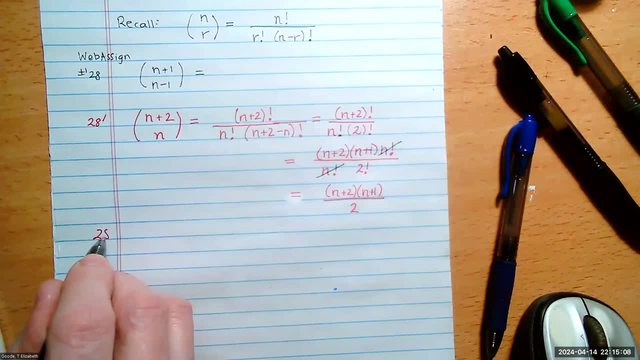 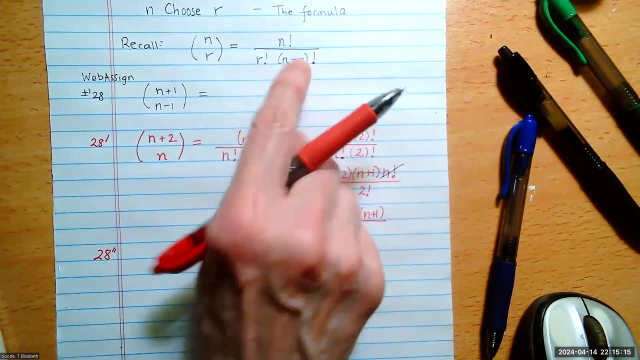 All right, let's do one more, because it's a little bit different when the denominator is a binomial. Let me show you why. Because when we subtract, you know, the bottom is the r right, And when you're subtracting r, if it's a binomial. 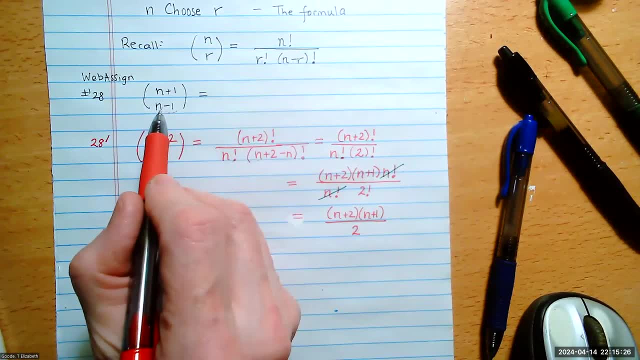 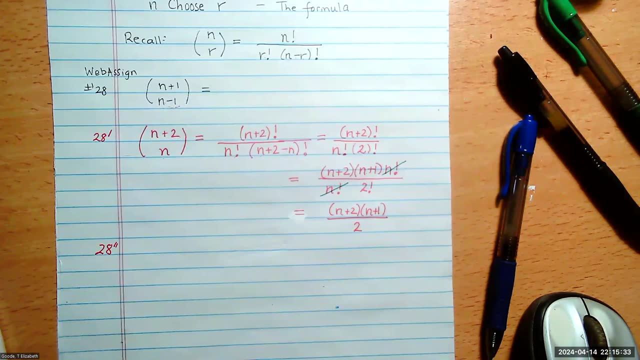 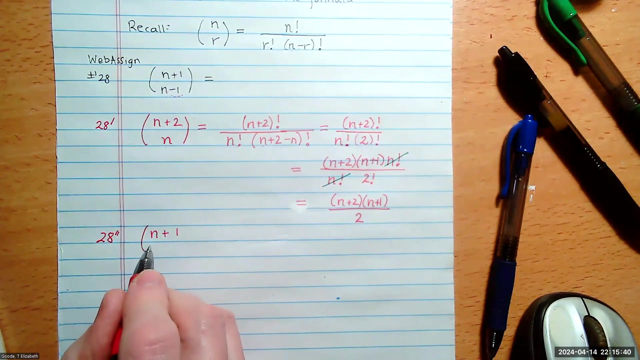 you have to be sure and distribute this minus sign across the n minus 1.. You see what I mean. It'll flip this minus 1 to a plus 1.. Let me show you what I mean. What if we have n plus 1, choose n minus 2?? 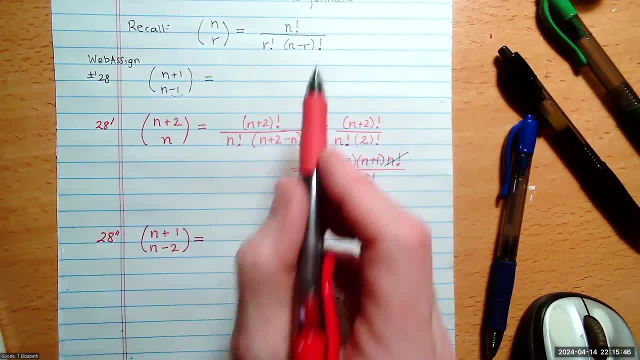 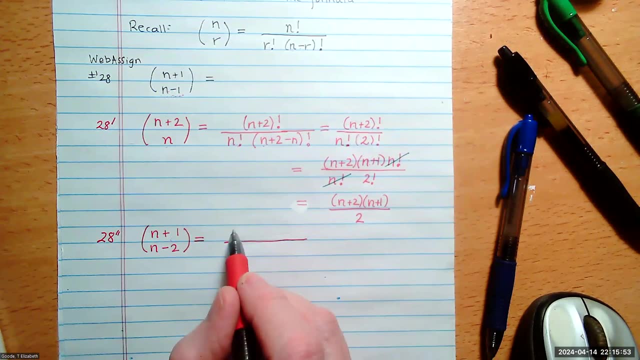 Okay, All right, using our formula Up top, what do we have? We have n plus 1 factorial, Good Over bracket n minus 2, bracket close: factorial. Then bracket open: n plus 1 minus n minus n plus 1.. 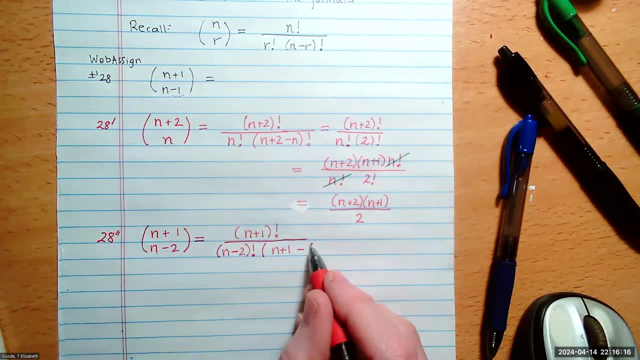 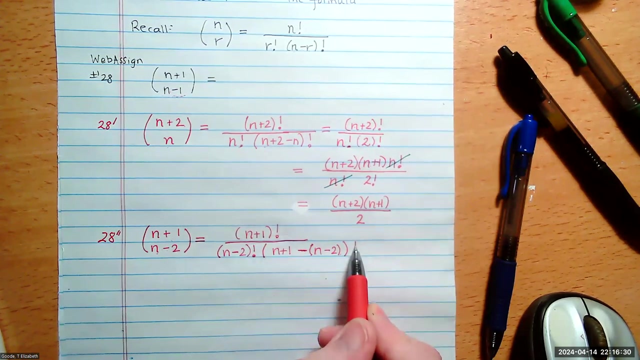 So n minus 2.. All right, so, no see, this is the r- is n minus 2.. So look, I'm putting a parentheses here. I'm putting it because this minus sign has to distribute across the n. 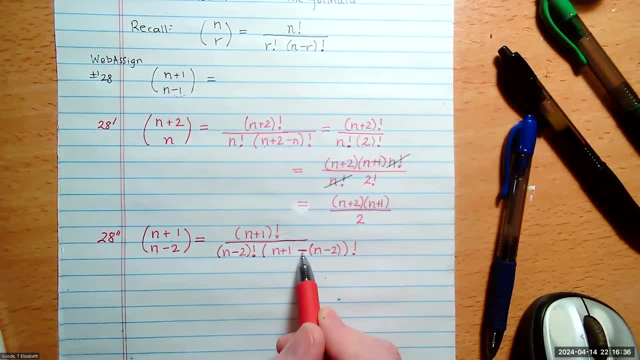 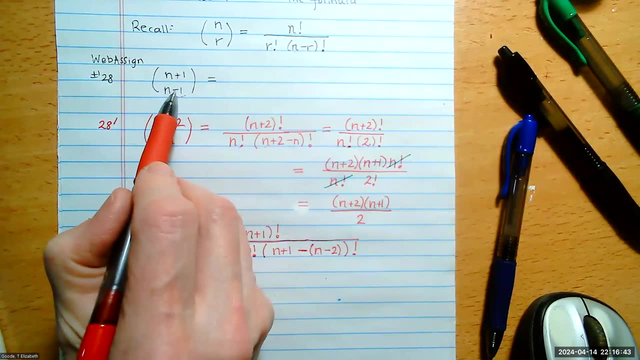 and it has to flip the sign of this minus 2 to a plus 2.. See, that's what I'm trying to tell you. So when you do this, this minus sign is going to flip. It's going to flip the n minus 1 to minus n plus 1.. 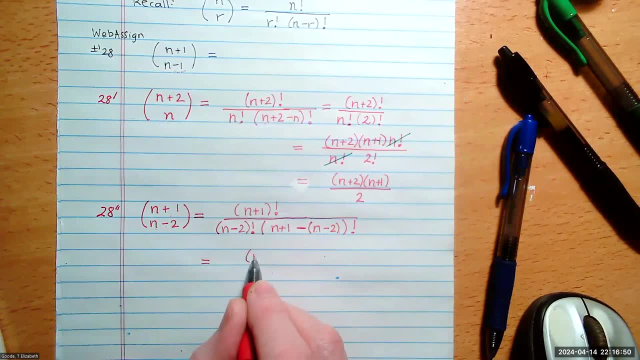 Got me Mm-hmm. All right, so here we go. So we've got n plus 1 factorial up top n minus 2 quantity factorial. and then let's simplify this: This is n plus 1 minus n plus 2.. 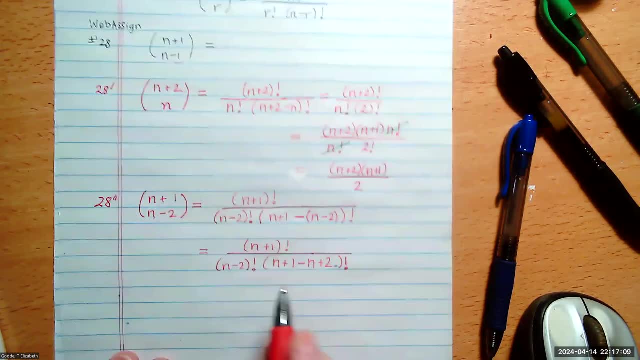 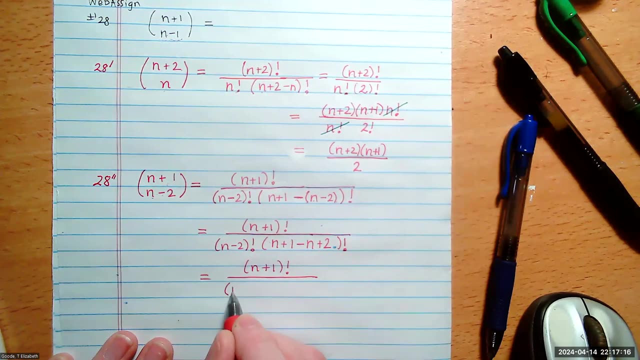 See what I'm saying. Yes, All right, now let's keep going before I even try to evaluate this. okay? So I don't even know what's bigger, right yet. All right, so we have the n minus 2 factorial. 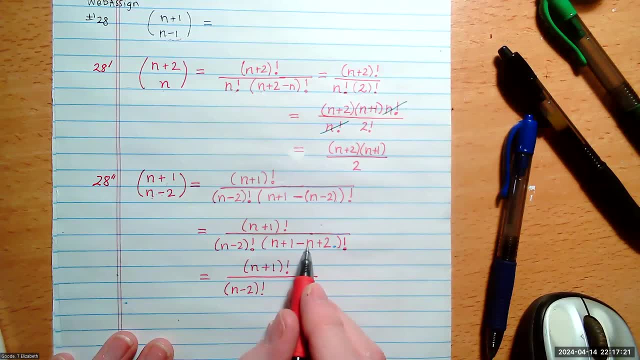 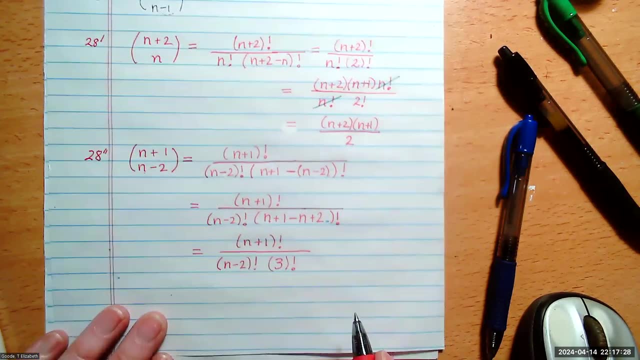 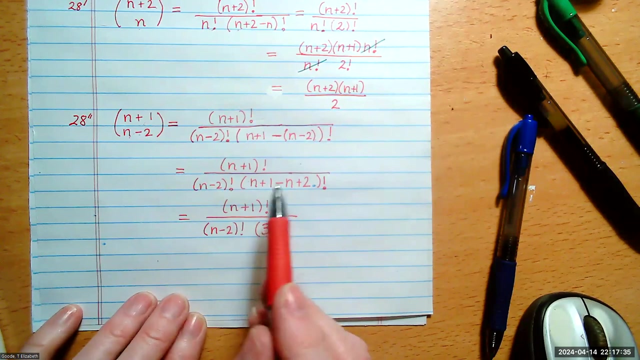 All right. so what is this? Oh, the n minus n cancels, but I've got 1 plus 2 down here. This is 3 factorial. You with me, Mm-hmm? Now, great, Now we're ready to start trying to figure out how to cancel stuff out. 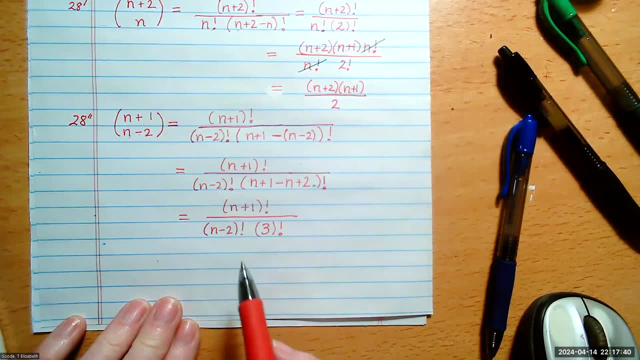 Which is bigger? n plus 1 or n minus 2? n plus 1.. So we're going to break the n plus 1 down until we see n minus 2.. So here we go. We're going to break down n plus 1 factorial. 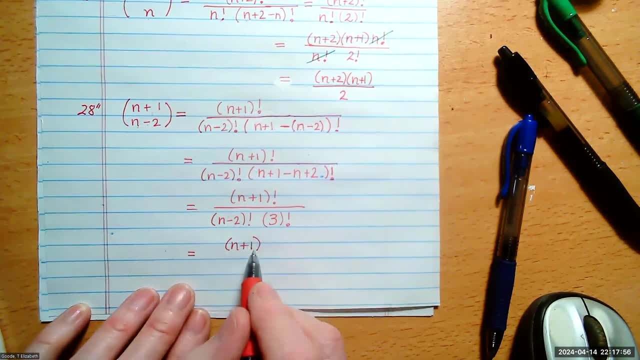 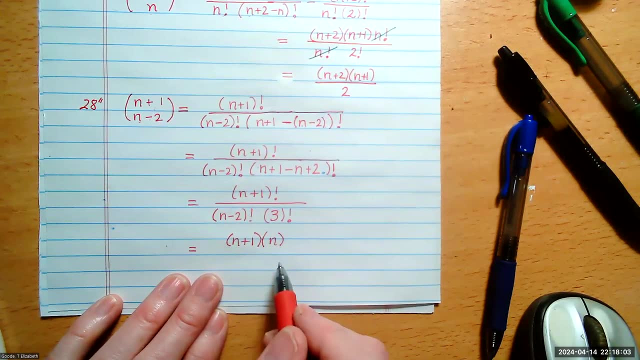 It is n plus 1 times. what's 1 less than n plus 1?? n? Good, And what's 1 less than that? n minus 1.. Good, Keep going. What's 1 less than that n minus 2.. 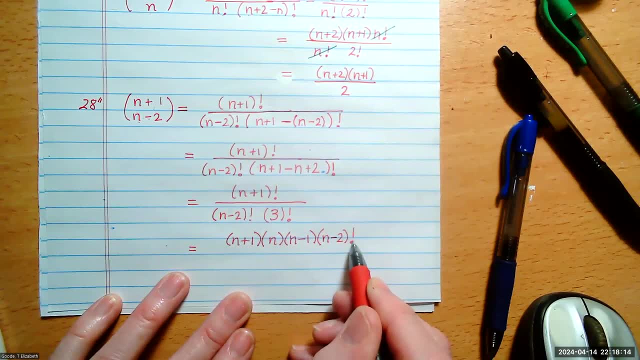 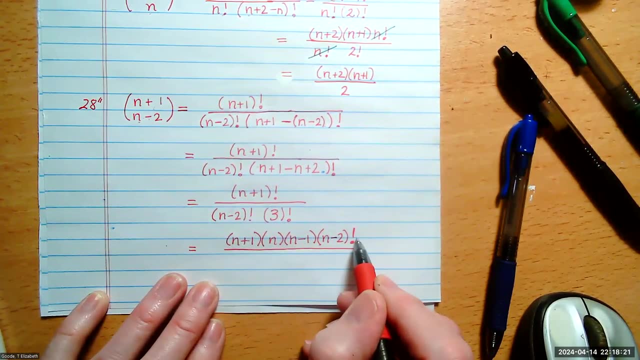 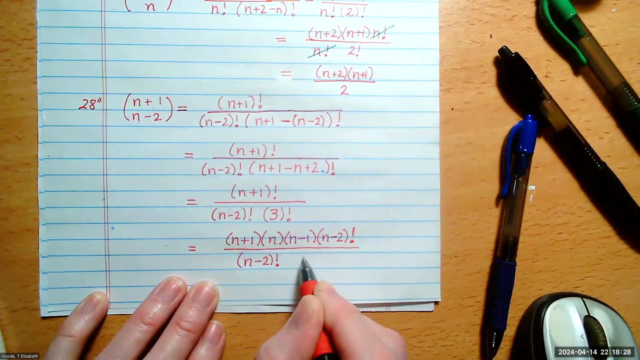 Ooh great, We got to the n minus 2.. And then everything less than that is expressed with this factorial, Do you agree? Yeah, Like the next would be n minus 3, then n minus 4.. But we don't need to write all that, because we're going to cancel the n minus 2 factorials. 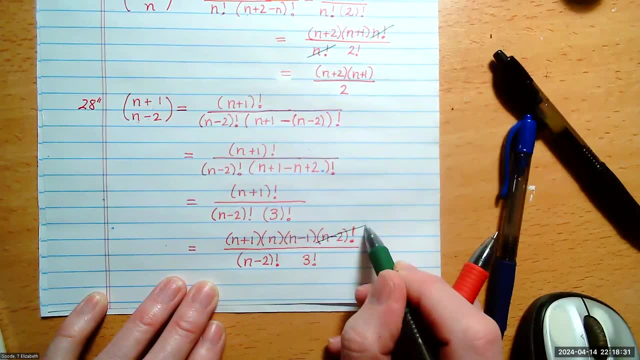 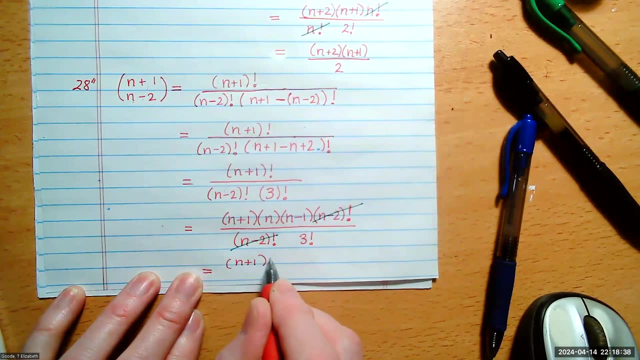 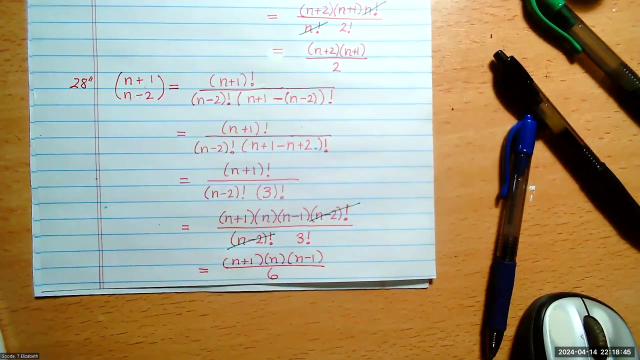 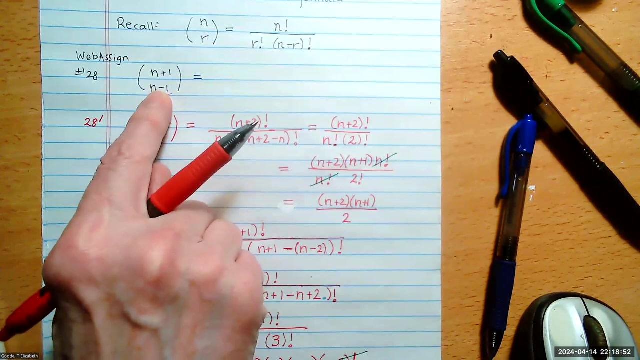 top and bottom now. So we're left with n plus 1 times n times n minus 1. Over 6. 6. Yeah, All right, So these two should make this look pretty easy. It's going to be a piece of cake now that we've done these two. 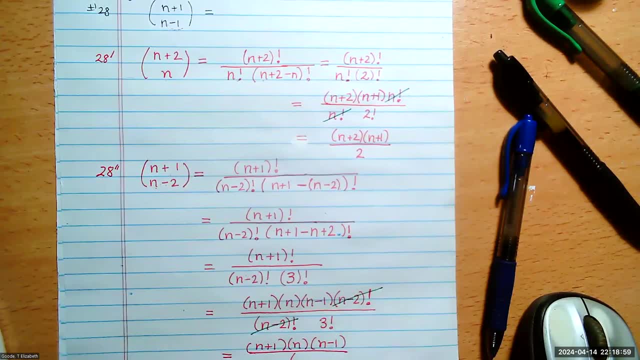 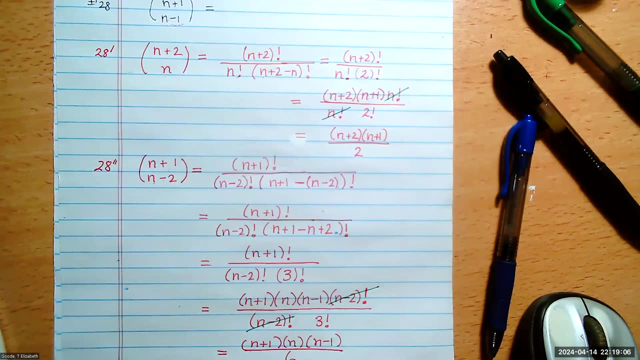 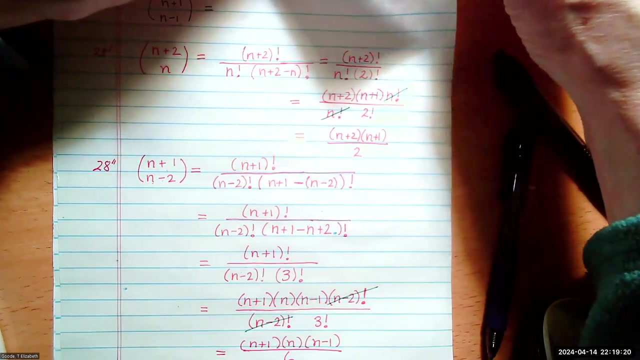 All right, Are we good? Yes, Well, thank you for coming to office hours and your peers and colleagues all thank you because you came. They're going to have a video, So you should definitely get them to take you out to lunch.